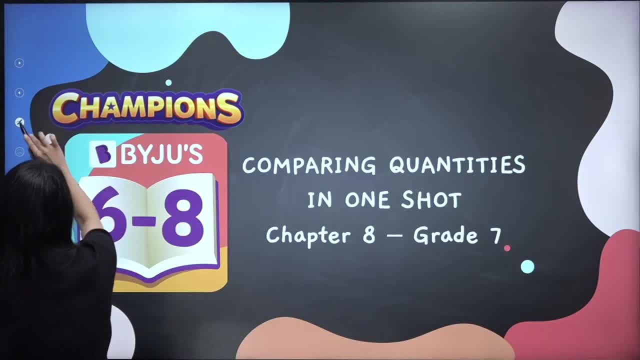 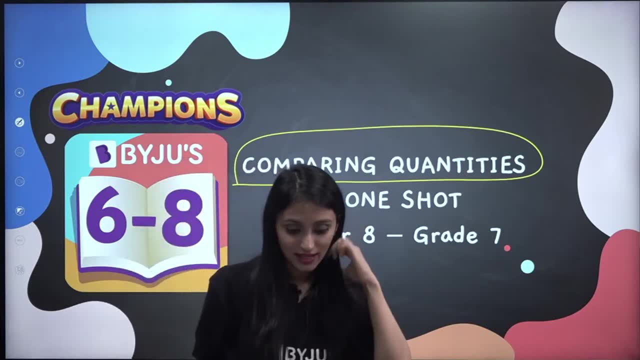 hume thot sa yeh discuss karte hain Aaj hum kya padhne wale hai, Kya padhenge, yaar aaj hum. Aaj hum baat karenge comparing quantities. Bohot time se kaya rahe the Ma'am yeh chapter lekar. aao Right New in this. 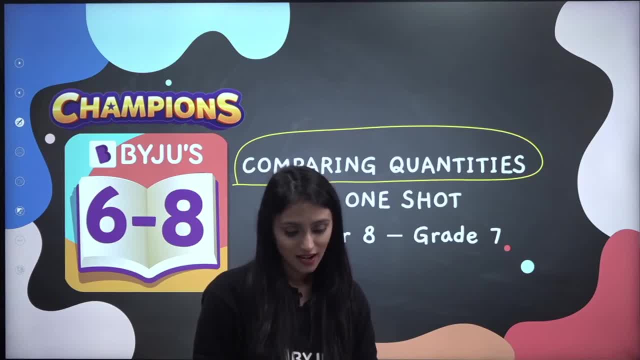 class Vignesh gamers. Yes, Thappan Dutta. See, some students are saying: ma'am, please explain in Hindi. Some are saying please in English: Amritanch, Kya ho gaya Block kardhiya Aarey, koi baat nahi. It happens at times because moderators also don't know ki kabhi, kabhi hojaata. 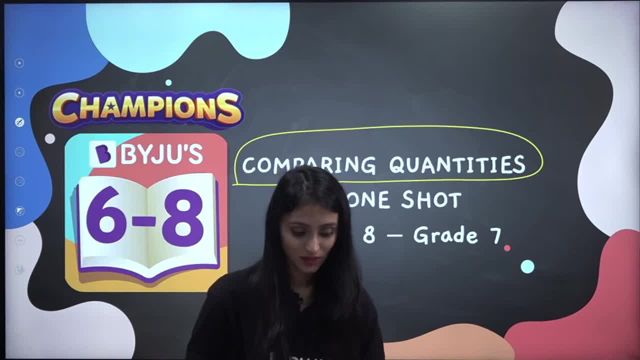 aise, But don't worry, Jab meri classes over hongi hai. I'll see to that. And I remember Gungun. you also said this thing. I'll see to that, Don't worry about it. So, Dhaniya. 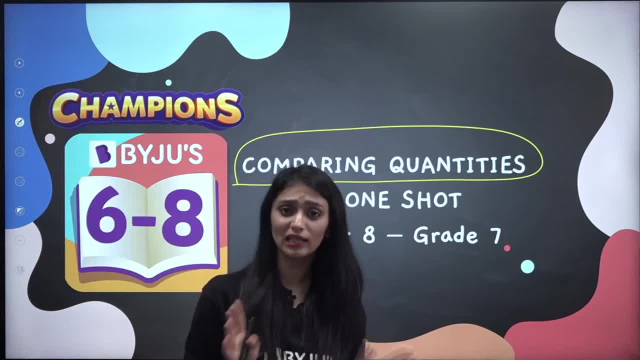 English, Hindi, Hinglish. don't worry, Ma'am will explain in both the languages. You just have to remind me At times what happens is when I'm explaining I also forget ki maine Hindi me bataya tha ya English me. So please you can just let me know in the chat, Ma'am. 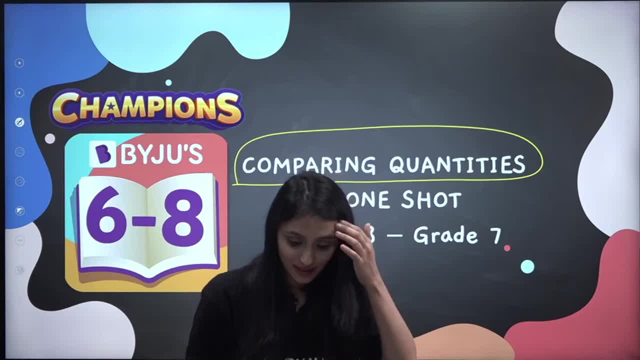 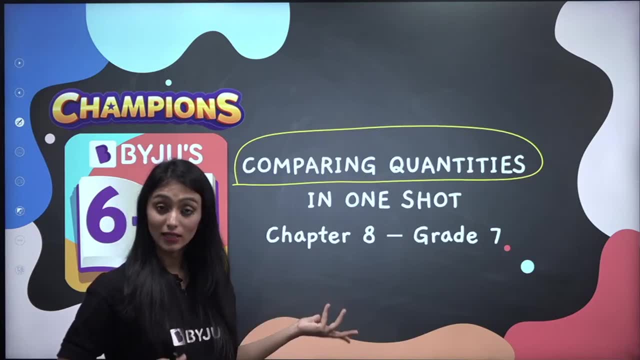 can you please explain the same thing in Hindi again or in English again? I know I know Thappan Dutta, So considering that I'm saying it please. Sometimes it happens with me also. I also don't realize ki Hindi me bataya ya English me. So in just one session we will. 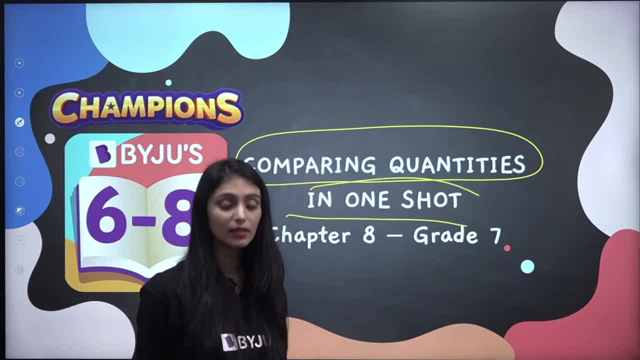 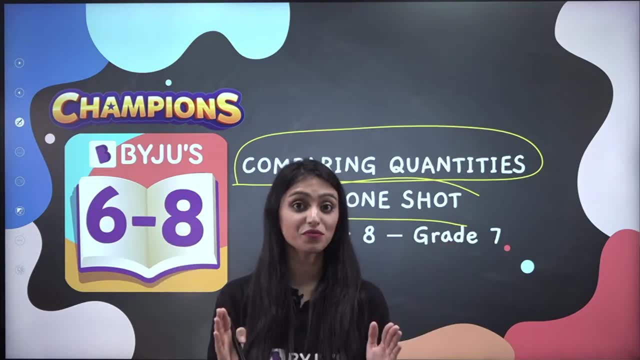 be covering the entire chapter, But when I say entire chapter, it's only the concept session. We will only be doing concepts today, But yes, just like we did for grade 6, we covered all the concepts first, and then we are coming up with a weekend session wherein. 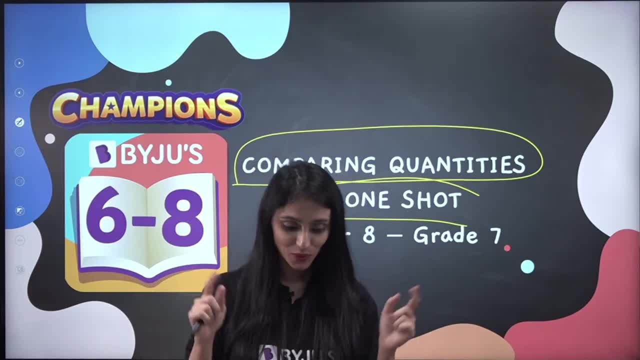 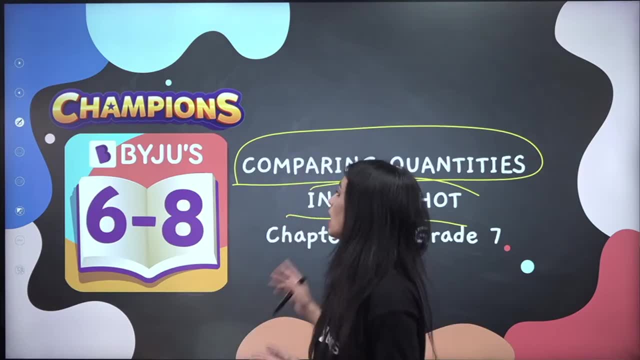 we will be doing the NCRT questions Similarly for you as well. Don't worry, Ma'am, we will get notes. Yes, you will get notes. Do you want the PDF of this session? Yes, I'm sure you would want. 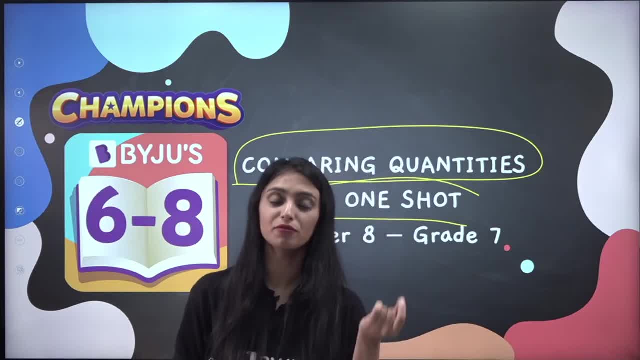 If you want the PDF, what you have to do is simply the link of the telegram channel for 6 to 8, it's given in the description. Go to that, join it. Arraam se apke paas notes saayenge Aaj nahi, toh definitely by tomorrow you will get it. Koi baat nahi. koi baat nahi. 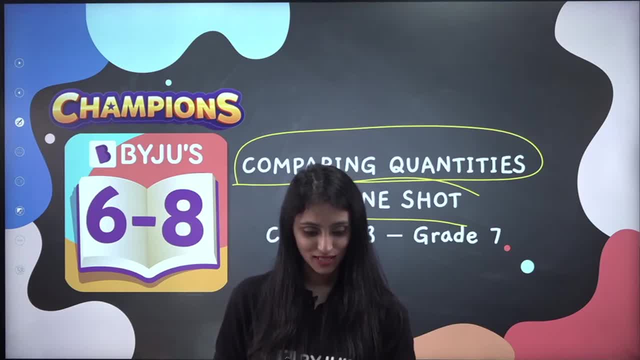 Teju, it's okay. Who is in KV? They will understand the language Hindi as well. Yes, Jasvi, bilkul, bilkul, Comfortable in both the languages, Great, great. Finally, class 7, after class. 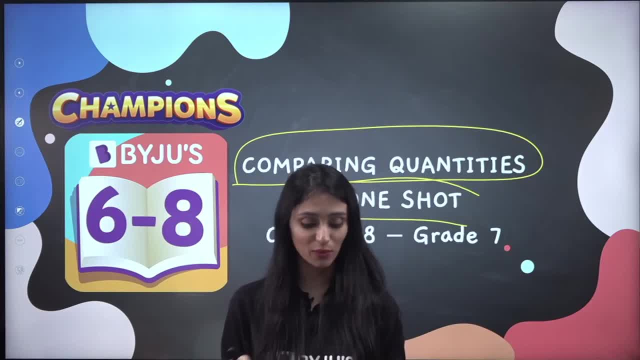 after a long time baise ek baat batta hu. I'm meeting you all after a long time, abhi kuch din ke baat se, Because we also thought to give you a break. exams kayi hoon ki over ho rahe hain. toh chur sa break, lo festive time bhi hai. enjoy it. Yes for this session. 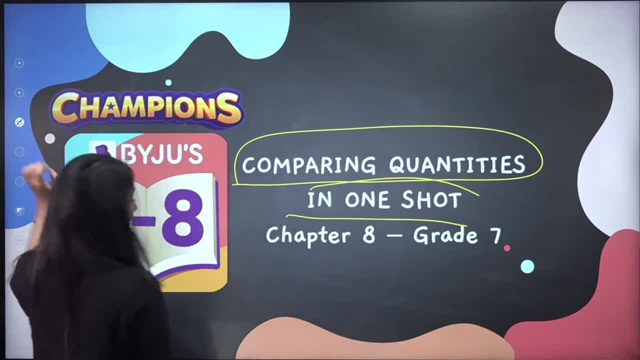 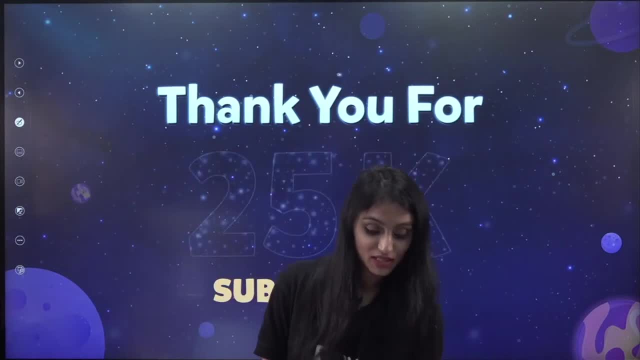 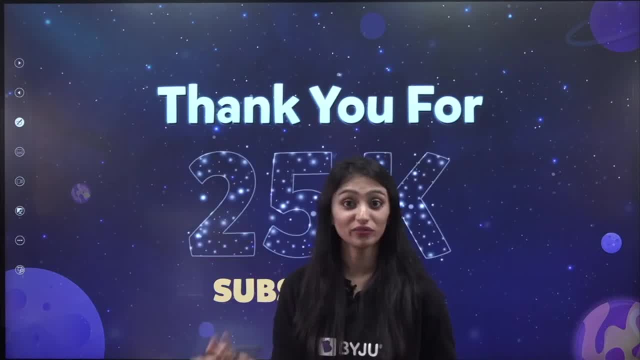 baar baar kyu bolte hain. There is a reason. subscribe nahi karte hu, aapko notifications bhi nahi aate hai. Aap bell icon hit nahi karte hai. Aapko notifications nae aate hai. You don't know whenever, when, which session is happening, when you say ma'am. 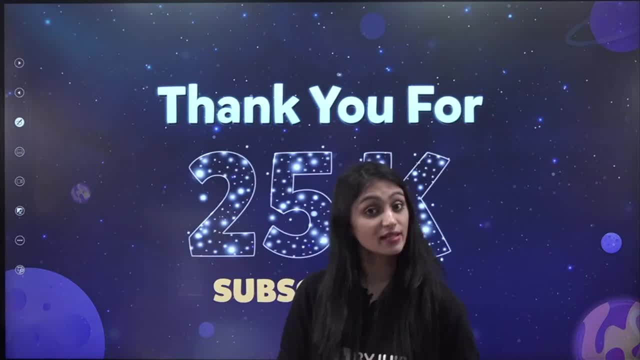 class 7, after a long time, ma'am, you are coming. you don't know that weekend sessions are also happening for maths. now, kaysa bata chalega aapko. If you will not subscribe it, if you will not hit the bell icon, if you will not join the telegram channel, ye teeno chise kar. 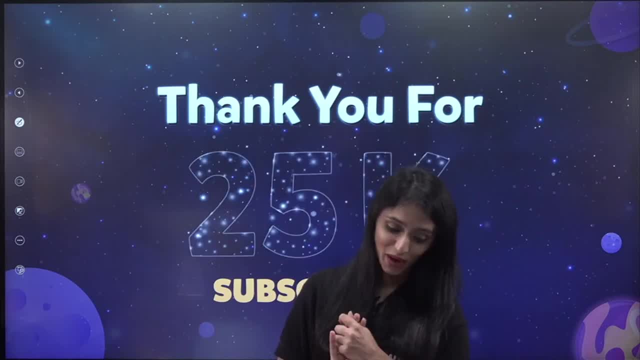 nahi hai, it's very simple, it hardly takes seconds. Yes, Thank you, Teju. I know you have subscribed. Abhi nahi, shival. wait, wait, wait, abhi aayega iske andar bohot jaldi hai. haan fatta fatte 50k bhi kar dete hain. 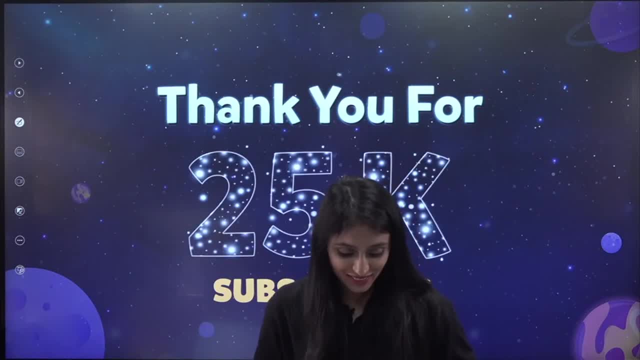 Kemer, Kosu. right see, my memory is so good. nahi sabke naam mujhe kaise yaad rehte hain for tomorrow's session, Naga Vaishnavi. nahi bhi hoga to. I will tell the team select karen. 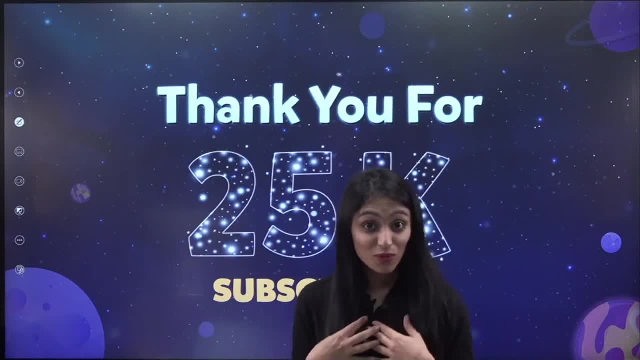 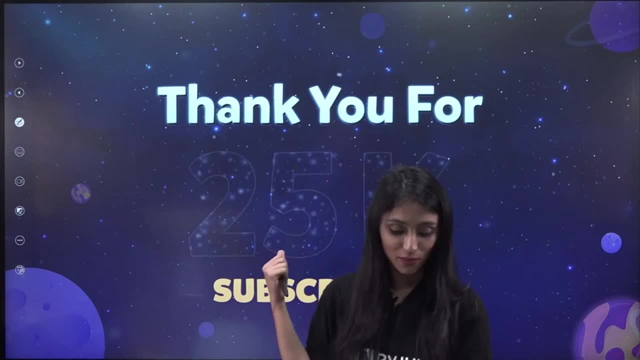 yeh aapko karwana hai. mujhe nahi puchna, ma'am, kab hoga yeh 50k aapko karwana hai, ma'am, thodi na karenge. yeh aapko karna hai apne friends ko share karo. yes, Aaru Madhu Nilaksha Gaming Mahi. 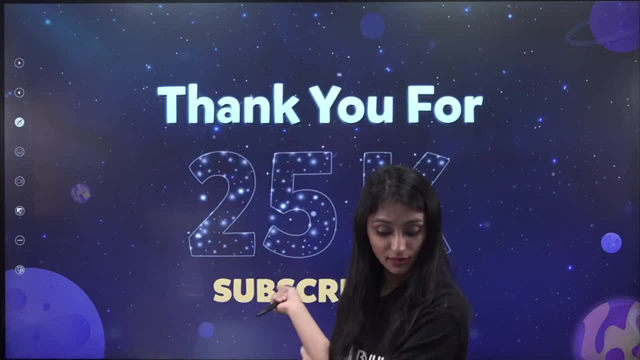 Antheka session. aaj bhi hai. aaj hai iske baad wala session. Antheka hai Sukanta Jaina. thank you, thank you, Kiran. yes, Laksh, of course I remember. ma'am always remembers. right, right, right Teju. 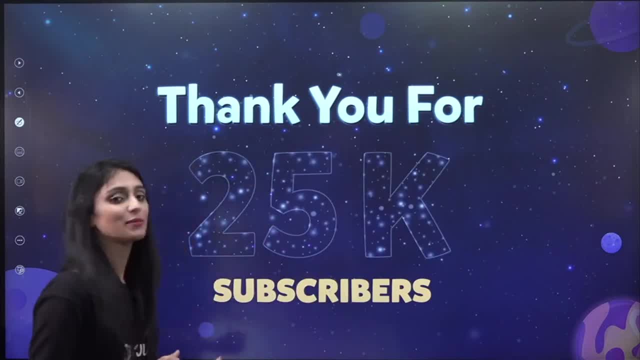 ab meri baat suno. jino ne subscribe nahi kara hai, pehle se fada word se pehle subscribe karo, aur sabko bata hai, purane students ko bata hai session me bohot maza. 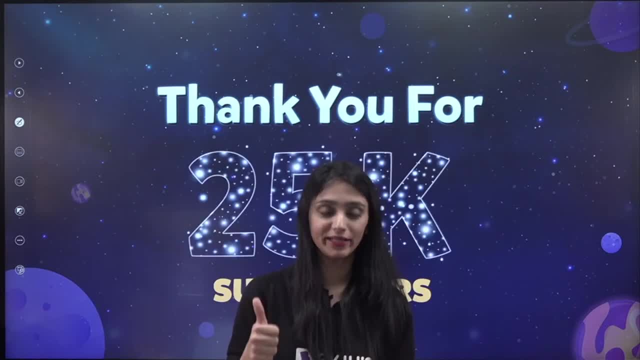 sabkot bhi aayega, sabkot samaj bhi aayega. so please, session ko like I can see here phone mere haath me hai fada word se abhi start kar rahe hain. Snagendra, badi chaldi hai, kya baat hai right, Prasanna Swapna, Arun Satya Prakash. 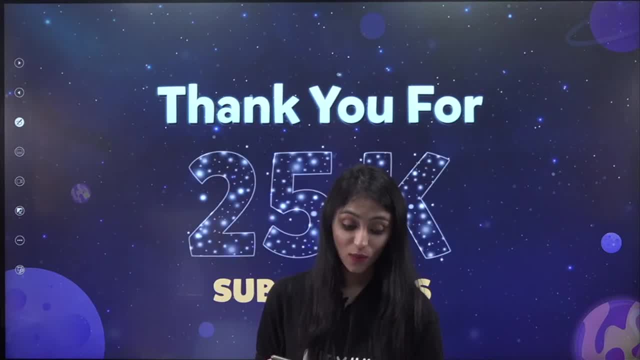 see, a lot of new names I am seeing here. but I tell you one thing: ek session ki andar mujhe yaad nahi honge naam. you keep coming for the classes regularly. I tell you, mujhe sabke naam dhyan rehti hain tab. 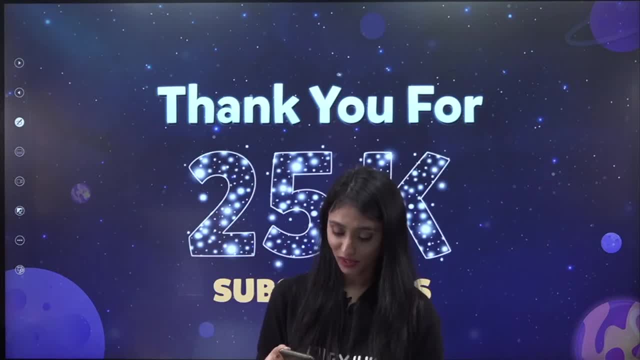 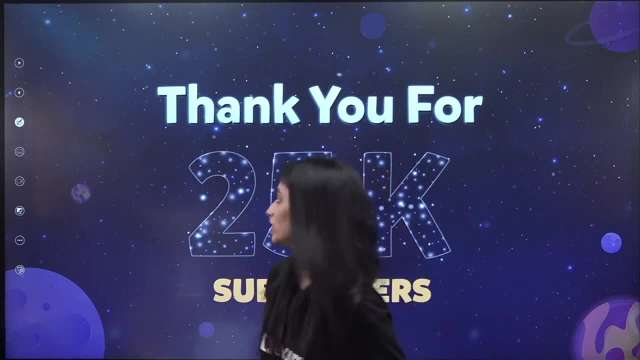 wow, Amritansh, her name is also Khushboo. Khushboo is a very common name now. wow, Amritansh, her name is also Khushboo. Khushboo is a very common name now. yaa, yes, yes, yes, likes zyada log session dekh rahe hain. likes come. how is this possible? 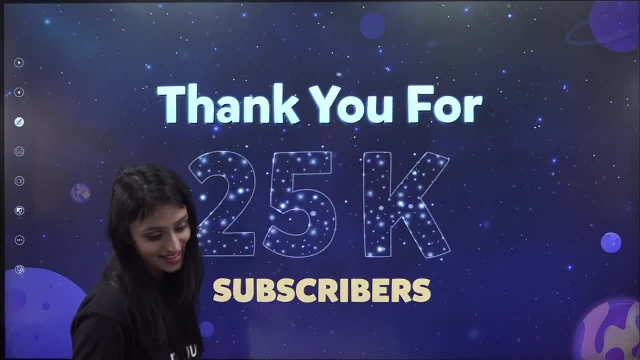 jabki pata hai, sabkot samaj aayega session me bohot interesting tarike se batayenge. yes, Amritansh, wow, 10th ki liye session me 10th class ho kaise phool chakti ho? 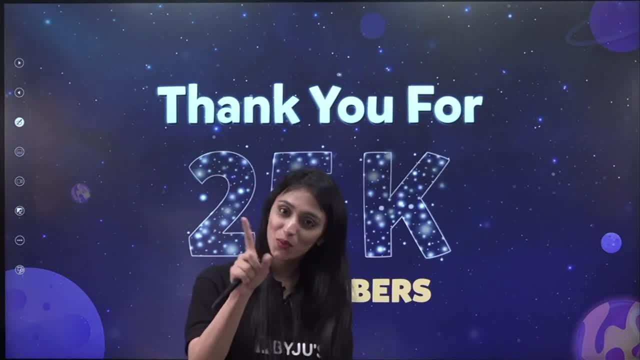 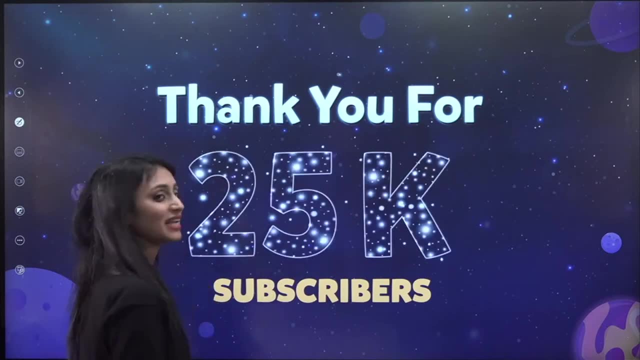 yaa 10th graders, come on, agar yaha par aayen yeh puchne ke liye session. kab hai weekend pe again? I am coming, don't worry. yes, chalye Kaustub, chalo theek hai bitta, ek hi baari me naam bata dete, toad, toad ke sabkuch bata rahe ho. 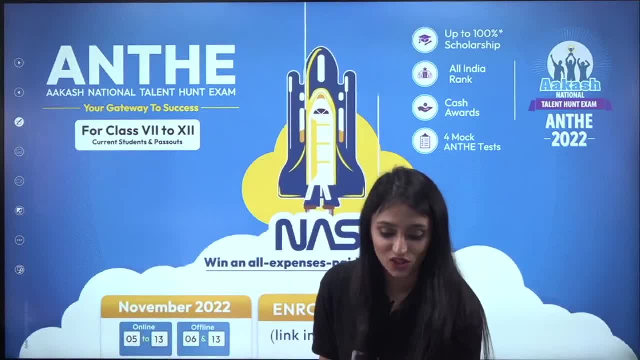 another interesting thing, sabke liye, ANTHE ke liye, jo log kera te ma'am session lekar aao. yes, Vaishnavi Agarwal, Prasanna new students subscribe kar diya. fata bache, patao chat me ma'am subscribe kar diya hai. 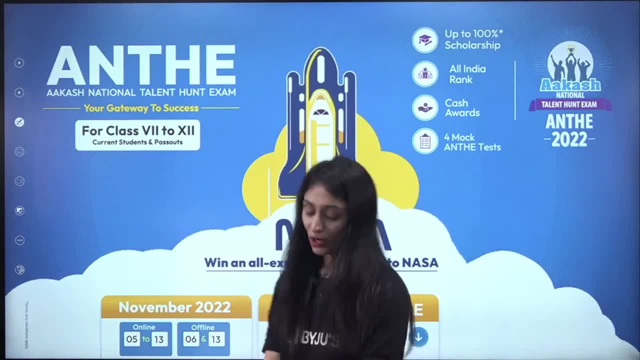 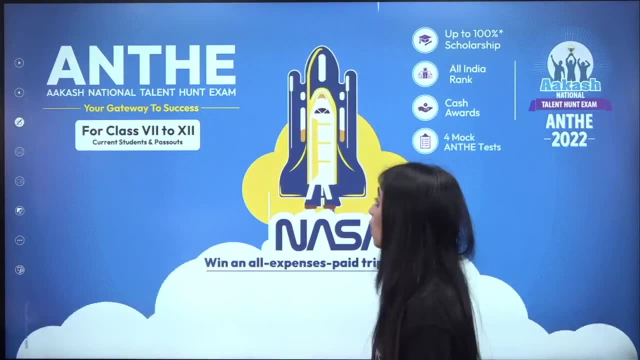 bell icon hit kar diya hai. yes, ok, ANTHE, kya hai? this is basically the biggest competitive level exam, I would say. this is conducted by Akash Baiju's now kis classes ke liye. this is for 7th to 12th graders ke liye. 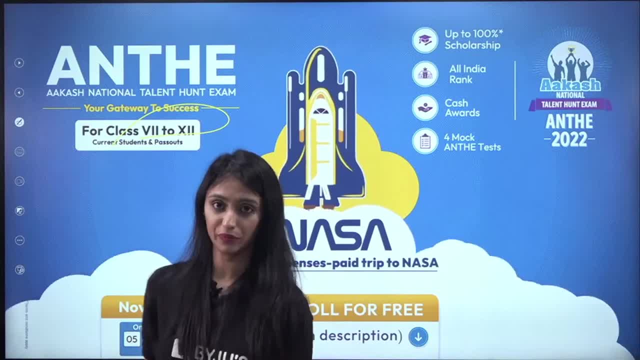 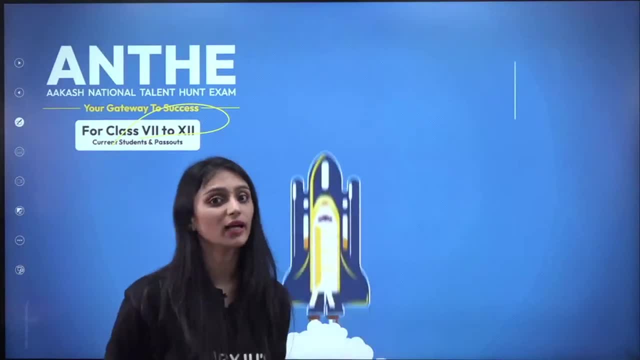 so aap sabke liye you are eligible to go for this exam. kyo dena hai paper kyo important hai, agar hume pata hai, hume medical ke liye agar jaana hai, hume non-medical me jaana hai, hume agar JEE dena hai, hume agar NEET dena hai. so you are very clear. 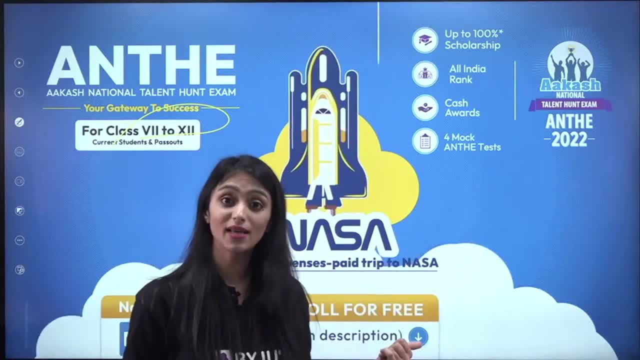 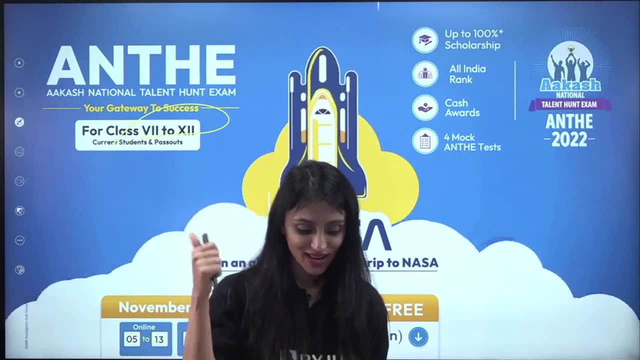 already aapko pata hai what you want to do in life. right, go for this exam, jitna, it's better to start early, always, right. yes, Radhika Yadav, subscribe, yes, subscribe karo, pehle name dekh liya, har bari name change karte ho. 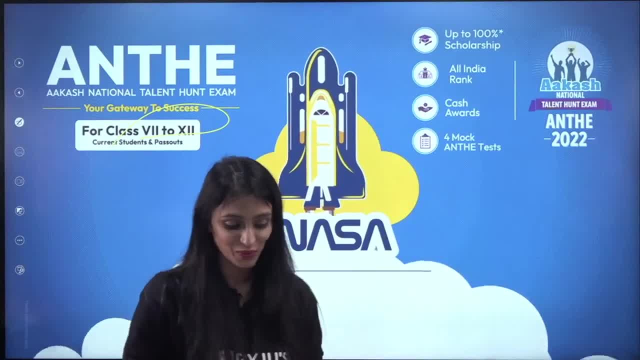 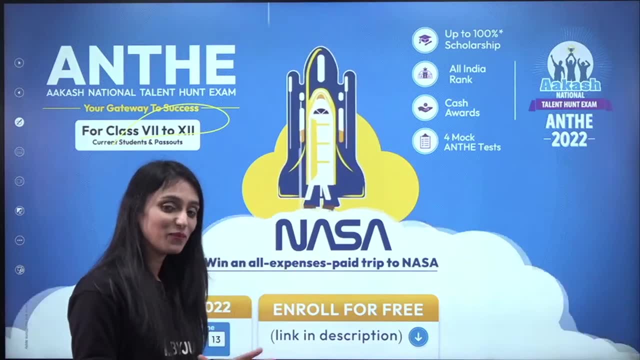 journey from your intelligent boy to board topper. I am sure you will top the boards. thank you, Laksh theek hai. so please, clarity hai already. kya karna hai? Medical dena hai, non-med dena hai? please go for this exam, yeh paper. dekho aapko idea lagega. 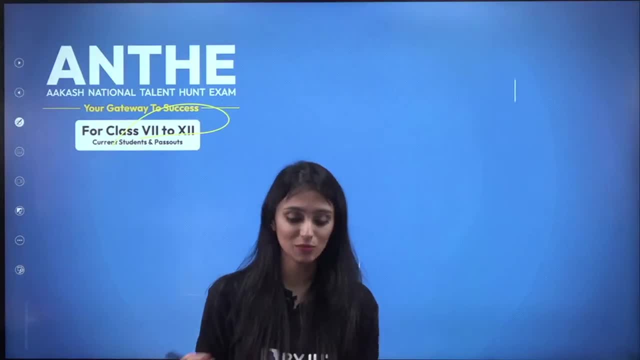 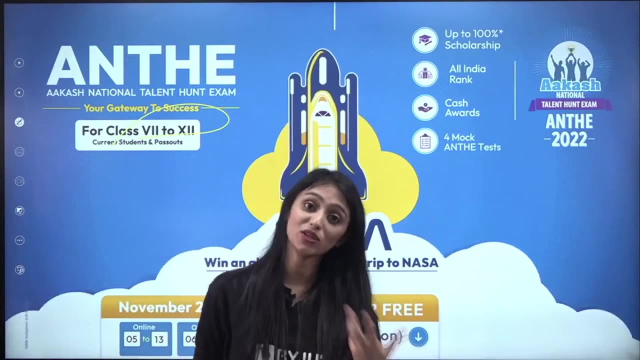 ki kaise compete karte hai at the all India level? yeh koi school ka paper to hai nahi, jisme syllabus sirf itna hi hai. yehi type ke questions aate hain. right, yaha par aapki actual knowledge check hoti, aapko pata lagta hai aapki strength kya hai, aapki weakness kya hai. 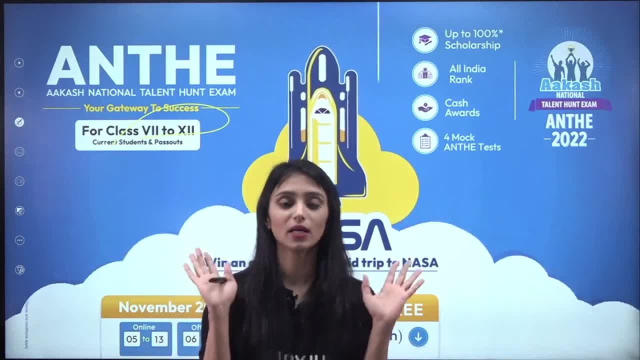 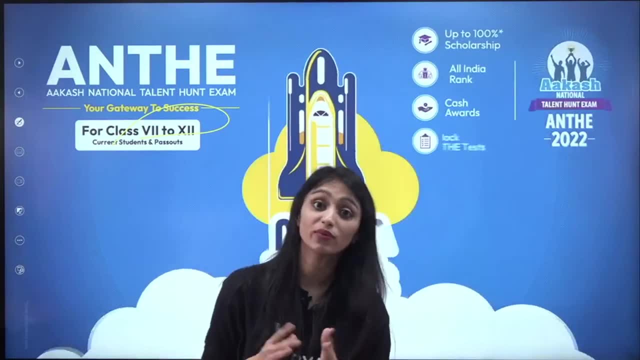 school paper se nahi pata lagta. I am telling you a very, I would say ek woh cheez jo hum generally realize nahi karte hain. hum top karke khush hota hai. achchi baat hai, hu asaan nahi hai, but hu difficult bhi nahi hai. right, yeh kuch hai jo cheez hai. 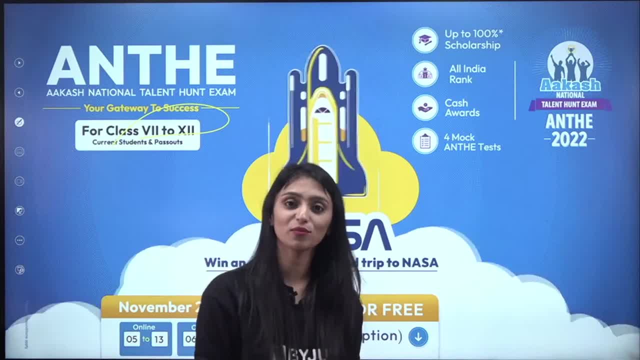 very challenging hone wala hai. go for it, aapko khud samajayega areas of improvement. aapke kya hai? agar aapne suna hai, toppers ko, agar aap ek bar unki video sunke, dekhiye, you will understand. 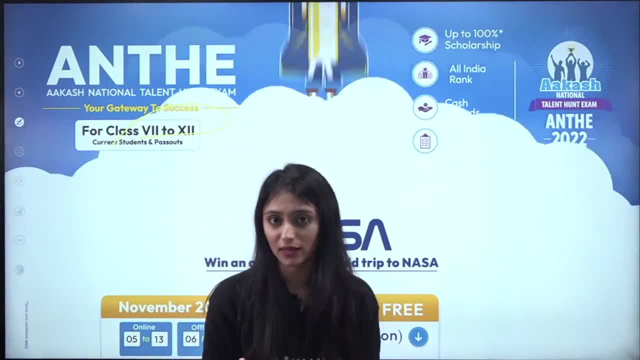 ho sakta as a teacher, when I am saying this, utna aapko na lage, but apne seniors se puchhiye: yeh yes, absolutely free hai, bilkul free hai. iska bhi description me link hai, description me link hai. 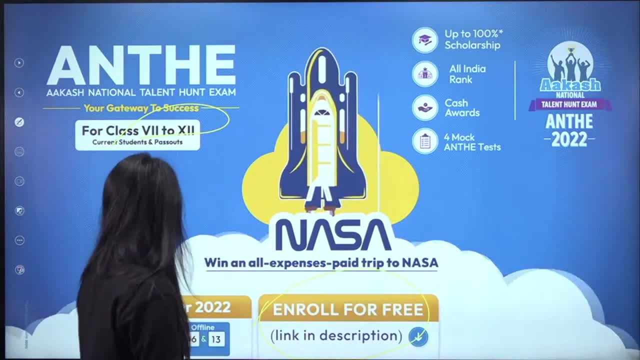 go for it. go for it and register, absolutely free of cost. aur yeh exam dono modes me ho raha hai November me. online mode me bhi, hai offline me bhi. aapko offline jaake nahi de na. 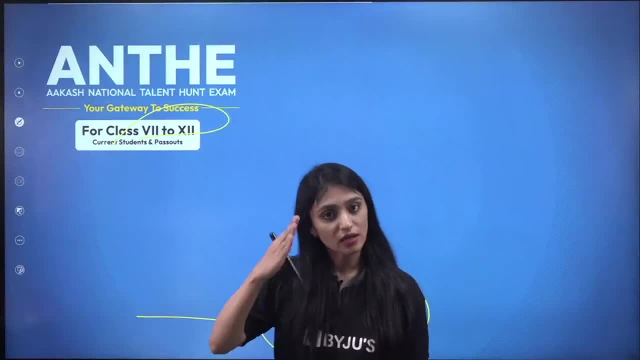 online mode me aap exam de sakte ho. 5 to 13 November me different different dates bhi di gayi hai, so that you can select accordingly, ki mujhe iss date pe nahi de na. that's why we have given you the option of multiple dates. 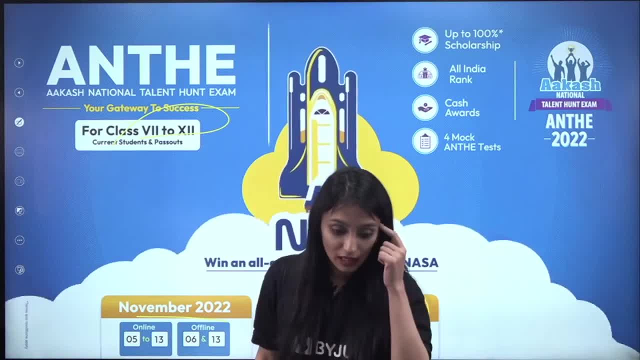 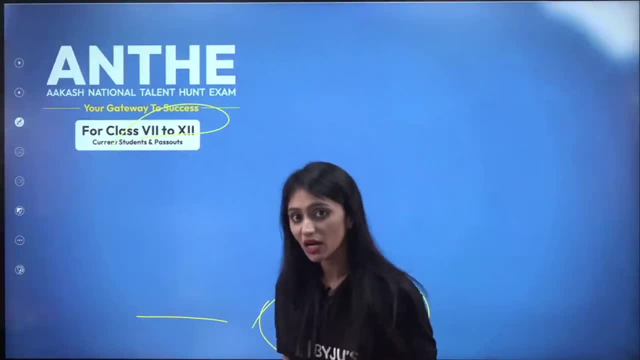 offline 6 and 13 November milta hai ke nahi. kyun nahi hai anthe ka syllabus? we have discussed this. acha, humne sessions kiye hai anthe ke syllabus, ki kya hai, kya nahi hai. phir bhi confusion. I tell you one thing. 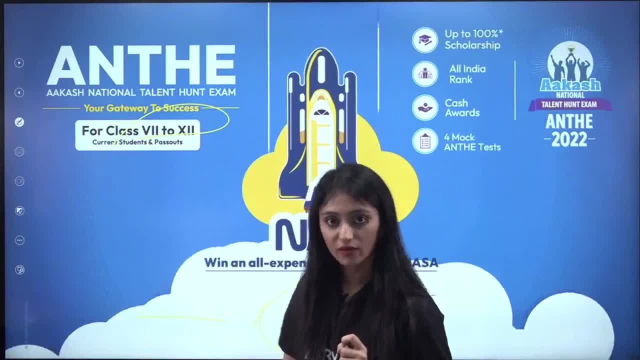 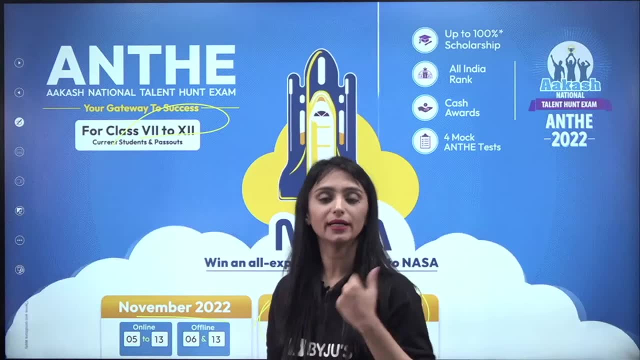 go to the site of Akash Anthe. Akash Anthe website pe jaiye class ke baad check karna. detailed syllabus bhi given hai. scholarship ka criteria bhi given hai. scholarship ka criteria. bhot interesting hai. 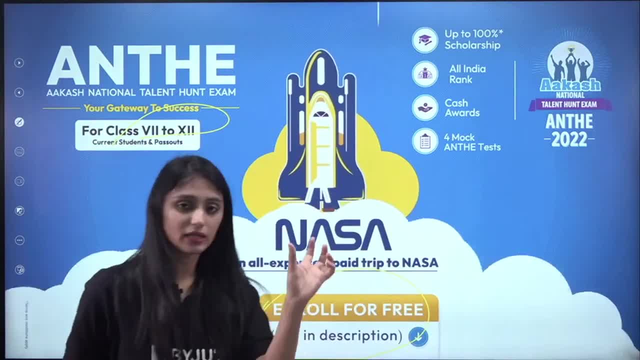 let's suppose usme rank wise diya bhai, aapka yeh wala rank aa raha hai, toh aapko 100% scholarship mil raha hai. 100% scholarship means: let's suppose aapko yeh Akash bhai jo course lete hain, aapko kuch pay nahi karna. 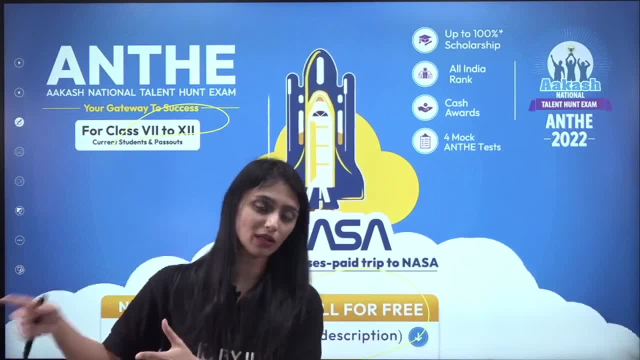 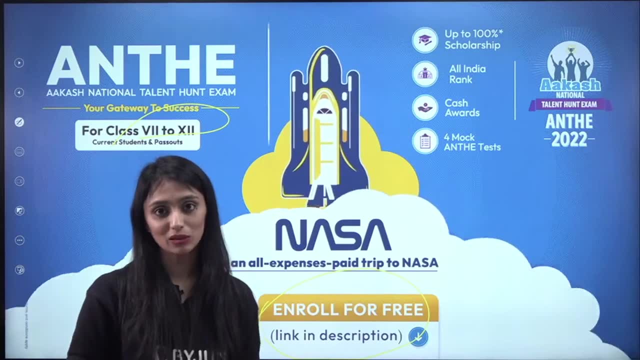 registration fees nahi, kuch nahi. so many things are mentioned there. kya, kya nahi pay karna hai aapko, so your parents are going to be so proud of you. aap ek exam dete hain, jisse aapko yeh pata lagta hai. pehli baat toh ki. 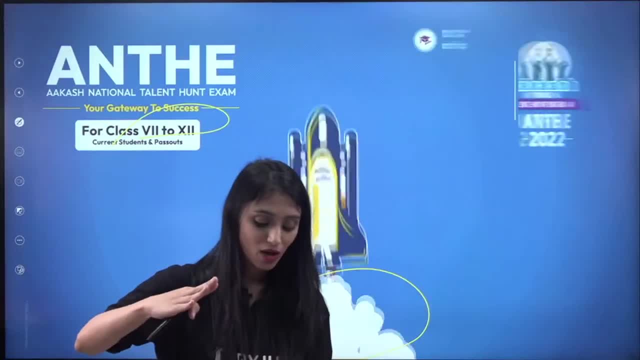 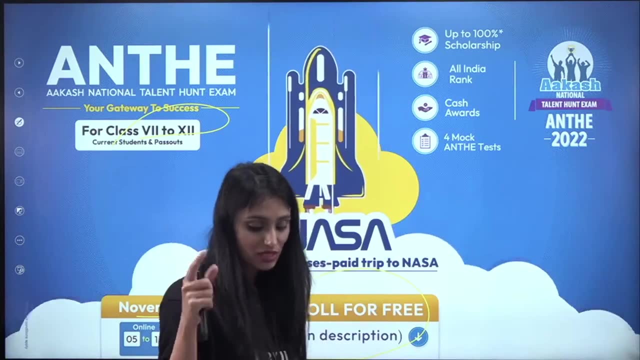 iss type ke competitive level exams, ka level kya hota hai, and you are saving their money as well. wow, yes, yes, Mona, you are visible. achche, maine bohot desi chart nahi dekha. toh don't think, ki chart visible nahi hai, bilkul visible hai. 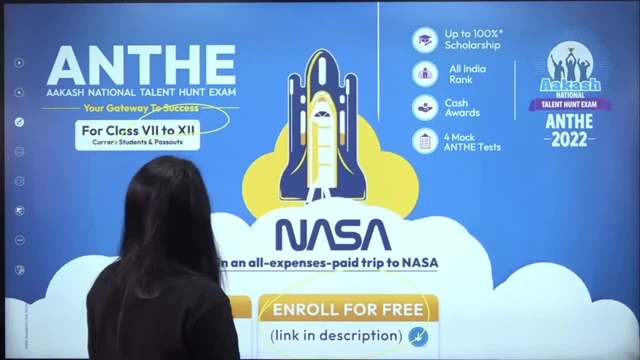 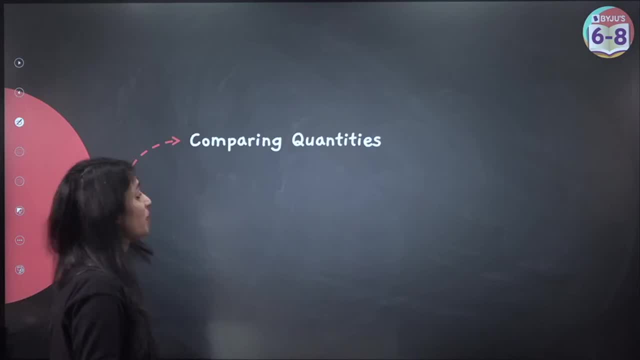 aur mock test bhi hongi usme. go for it, agar nahi, abhi tak register kar raha hai. kariyeh description mein link hai: chali, let's get started comparing quantities. ok, jahe, hum quantities ko compare karne ki baat karte hain. 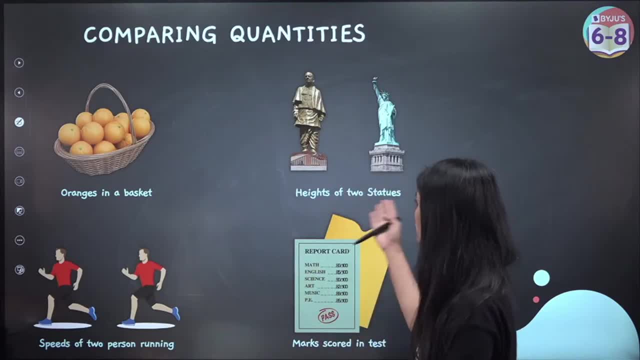 let's suppose yaha different different. aap examples dekh rahe hain: heights of two statues. agar michi yeh compare karna hai, dono statues hai, tabhi compare karungi. yaha par. aap dekh rahe hain marks code in a test. 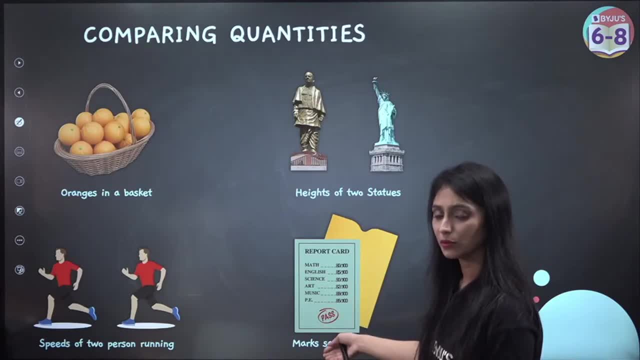 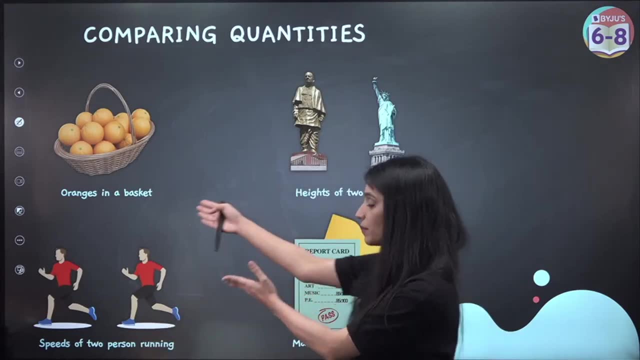 subjects hai different, different, tabhi comparison kar sakte hu. right, aisa toh nahi hai ki subjects ke mark ka comparison in ki speed se kar denge hum. aisa toh nahi hai. subjects ke mark ka comparison hum in oranges se kar denge nahi. 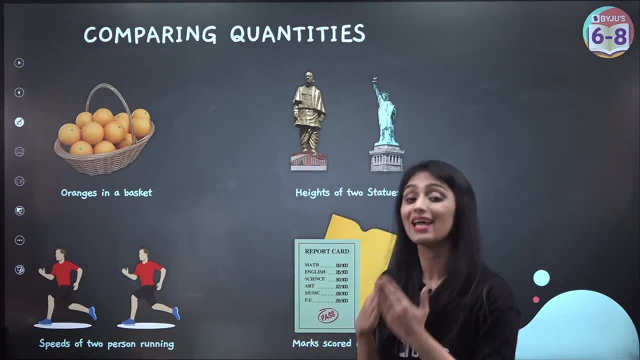 comparison karne ki liye. wo quantities chunko aap compare kar rahe hain, they should be same. whenever you are comparing something, the quantities that you are comparing, they have to be same, right, like we are comparing the heights of statues here. 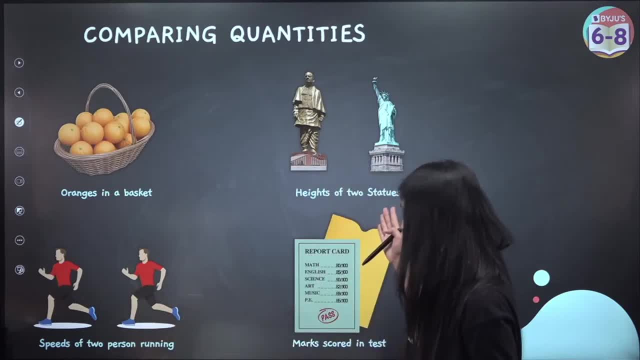 like we are comparing the speed of two persons running, like we are comparing the marks code in a test. quantity is same jis ki hum baat kar rahe hain. yes, Kiran, are you talking about beta anthe? yes, beta anthe exam. 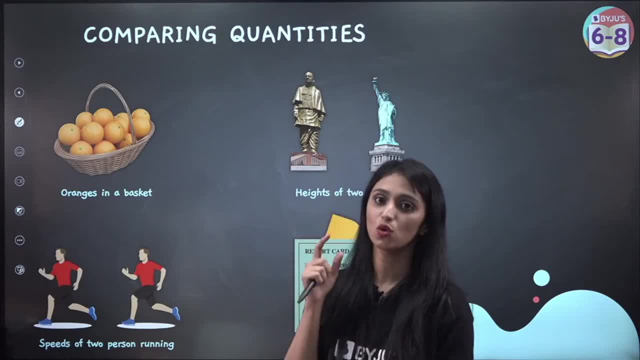 anthe exam kaise denge kya hai, offline, online jo hongi dates beta hu mentioned hai detailed. agar aapko ispe kuch bhi chahiye information, akash anthe site pe chahiye saari information available hai. 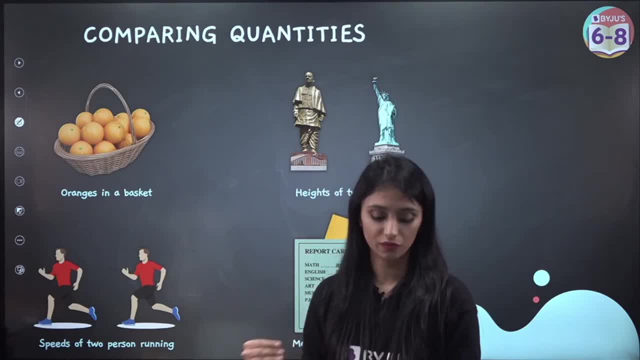 aap neeche jaake pele register kariye, aapko information mil jayegi fir right arey cost 0x koi baad nahi hai. mai class ke baad beta iske baad ek session hai, uske baad definitely check kar rahe hain. 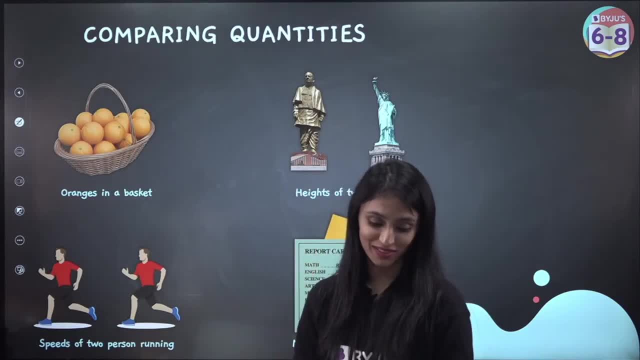 right, arey cost 0x. koi baad nahi hai mai class ke baad beta iske baad ek session hai. uske baad definitely check kar rahe hain. right, I'll check with the moderators, don't worry okay. 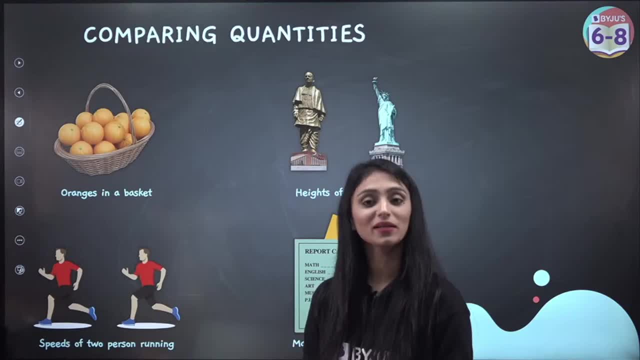 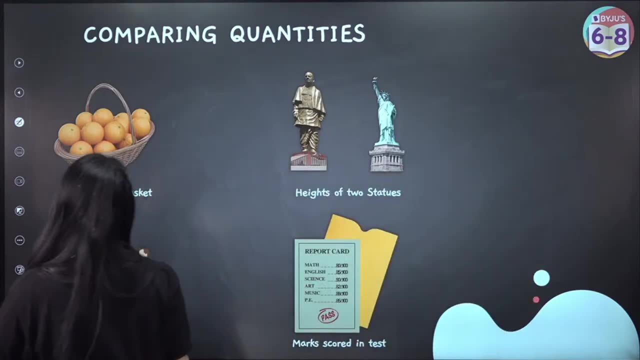 8 ka hai. arey, koi baad nahi, koi baad nahi, kya ho gaya prepare karo, uske liye thik hai. so quantities ko aapko, aap similar quantities ko hi kar sakte hain, right. 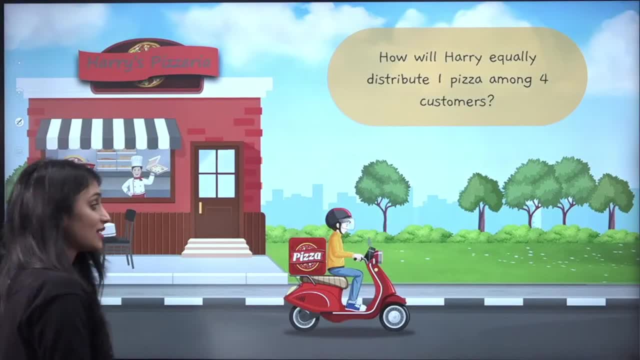 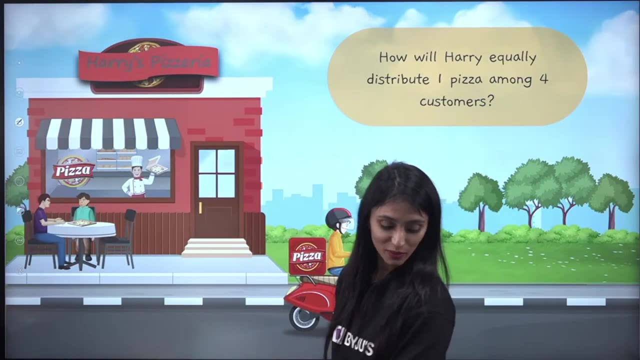 chaliye. let's move ahead now to understand this better. ek scenario: consider karte hai. can you see this? Harry's pizzeria. wow, yaar, pizza ke baarein baat karke na. I feel like eating it right. 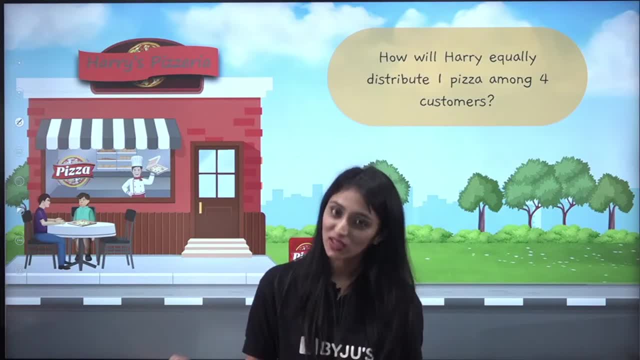 but abhi to obviously possible nahi hai, kyunki session kar rahe hain. yes, Srishti, of course your messages are visible. kiska mock test, shival. kiska mock test everyone. stop ma'am's pen. 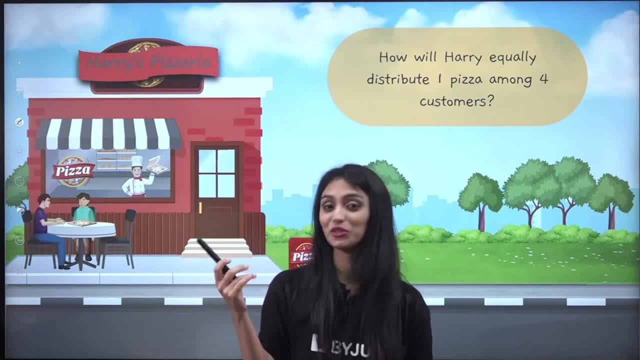 aacha sab koi pen ki story. aap bata hoge right, yeh koi normal pen nahi hai. beta, this is a magical pen. kitne marks laane honge? for what? scholarship ke liye? 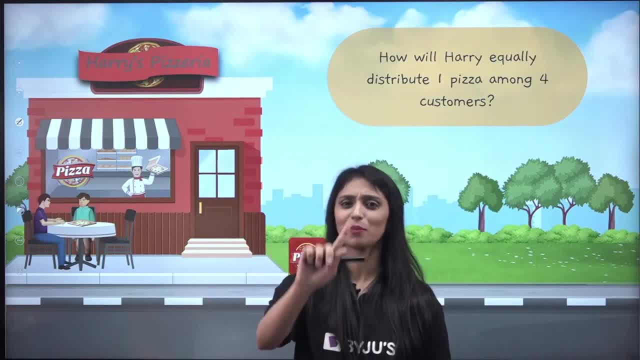 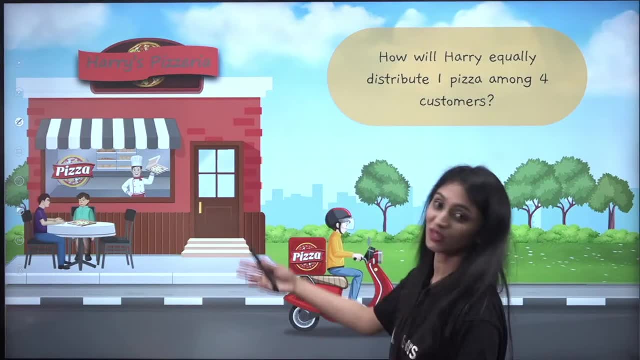 saara criteria sab mentioned hai. check kariye ekin class ke baad check karna. please, abhi mat check karna class ke baad. yes, hungry right I also. I'm also hungry, ek toh saath mein khana dikh jata hai. 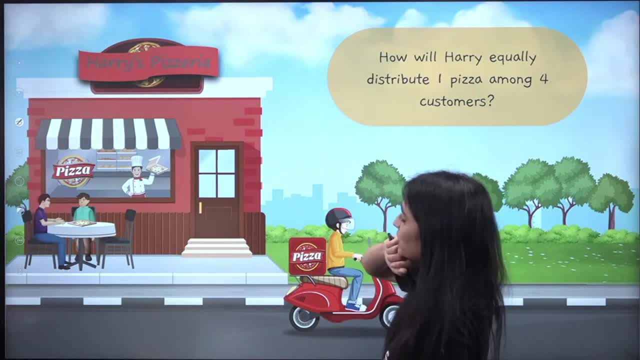 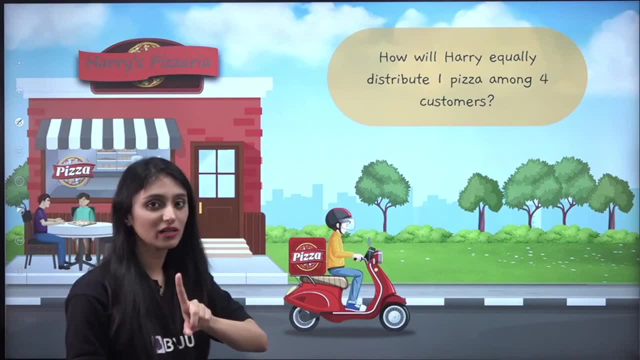 and you know it, mera khane ka story. so Harry's pizzeria ab ab ho kya raha hai yaha pe, ab yaha pe soch rahe hai, ki agar Harry ko equally ek pizza distribute karna hai. 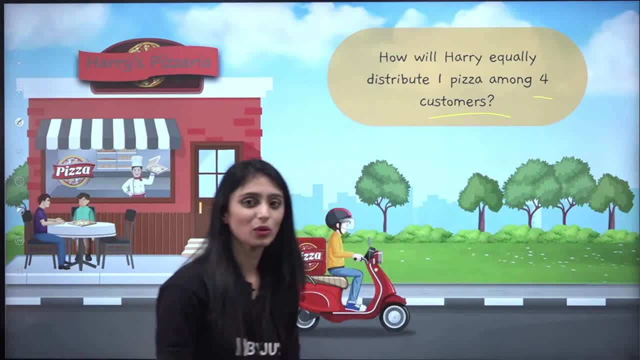 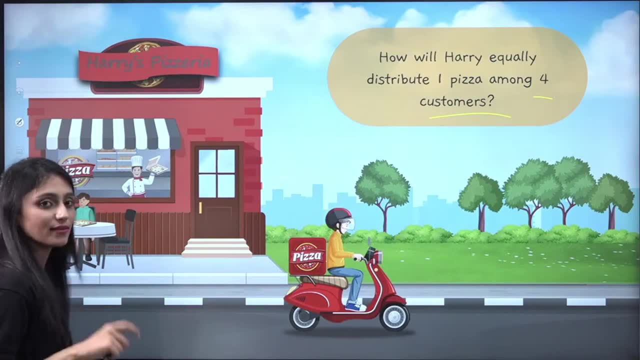 among four customers. so how Harry is going to do that? ek pizza among four customers. yes, yes, yes, I want answers. kaise distribute karenge? that's where this ratio, this comes into picture. so ratio kya hai? basically, yes, yes, yes, I want answers. kaise distribute karenge? that's where this ratio, this comes into picture. 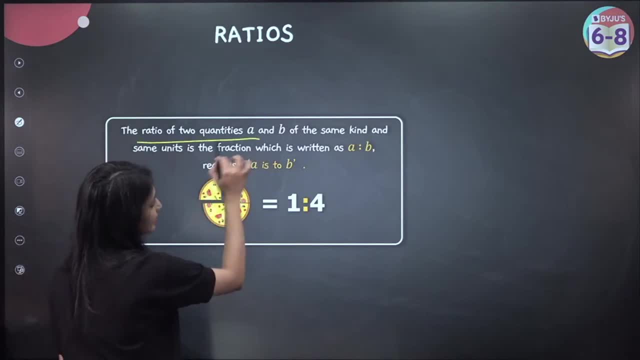 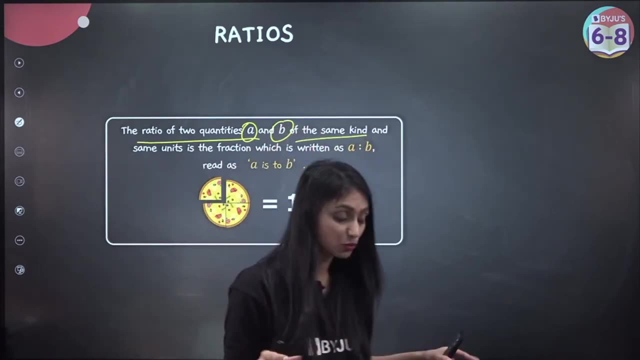 so ratio kya hai? basically? it's basically. doi koi doi quantities ke kar baad kar rahe hain, let's suppose ek quantity A hai, ek quantity B hai of the same kind, same kind. ma dubaara bol rahi hu. agar mai baad kar rahe hu, toh mai doi pizza ki hi kar rahe hu. same kind, honi chahi quantity hai. 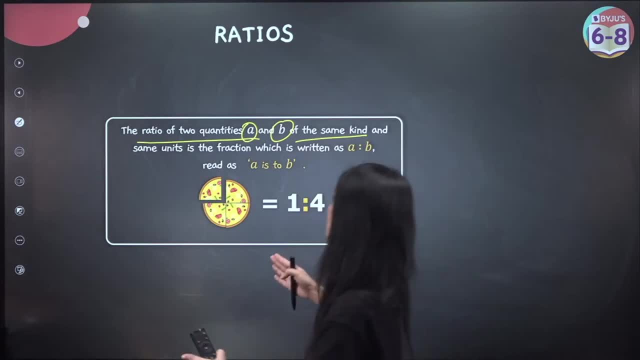 nahi apne pizza ko height le liya, kisi ka kahin bhi. aap kuch bhi aise compare nahi kar sakte. same kind and unit b same hona zaruri hai, agar hum length compare kar rahe hain. 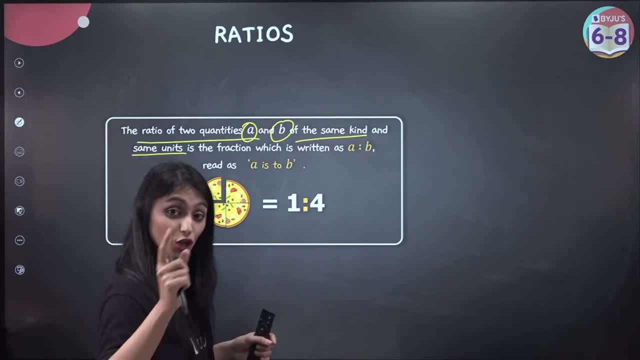 toh aisa nahi hai, ki ek length aapki kilometer mein hogi, toh ek millimeter mein unit b same karna hai. okay, now is the fraction which is written as A is to B. that means A is to B. how do you write it? 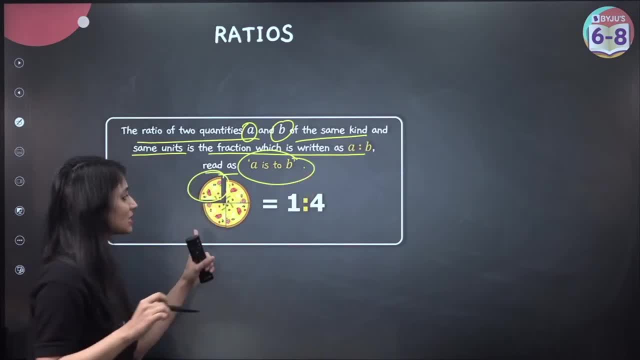 Let's suppose mai iss pizza ki baad karu iss mein yeh wala share kitna hai. it is yeh iska ek slice hai. rest poora pizza ki hai usme 4 slices hai. this is going to be 1 is to 4, that's how you compare them. 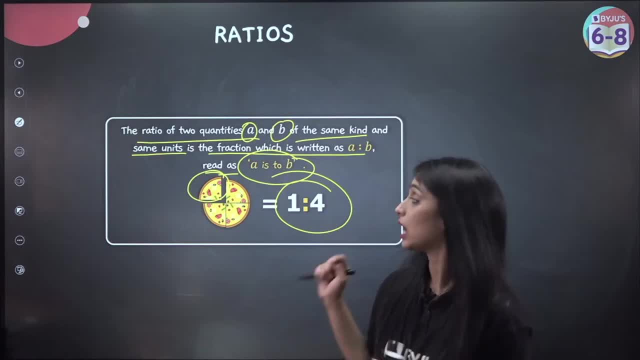 that's how you represent them. yes, 1 by 4, fraction mein aa gaya 1 is to 4, in ratio mein aa gaya pen dhyan delo, beta, pen pe sab ka dhyan hai. yes, 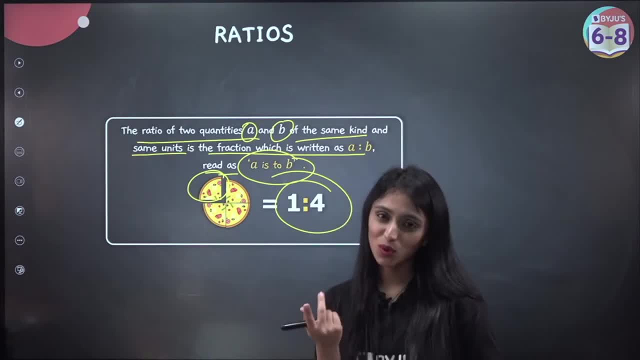 wow, wow, Pooja Yadav, amazing kuch cheeze bhool bhi jaati hu, but now that you are reminding me, that's very nice scholarship ke liye. that's what I am saying, Radhika bete, aapko Akash Ante ki site pe check karna hoga. 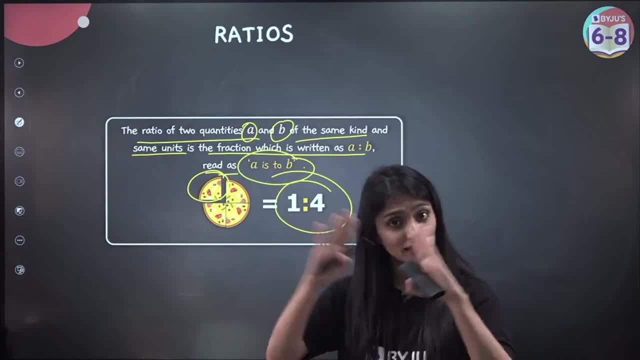 detail mein there is a big table. mujhe poora table yaad nahi hai, big table, aur usme ne ispe ek session bhi kiya tha. I am not sure, aapne wo dekha ya nahi. 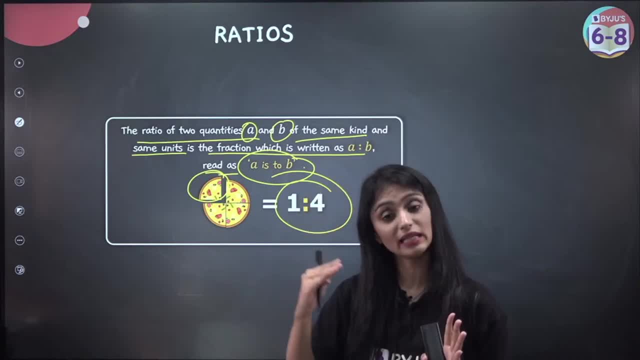 bohot bada table hai. aap usko dekhiye usme poora criteria mentioned hai. yes, fraction, this is fraction aapka. yeh numerator hoga hai denominator ratio mein. aap usko kaise likhte hain: this is ratio right. 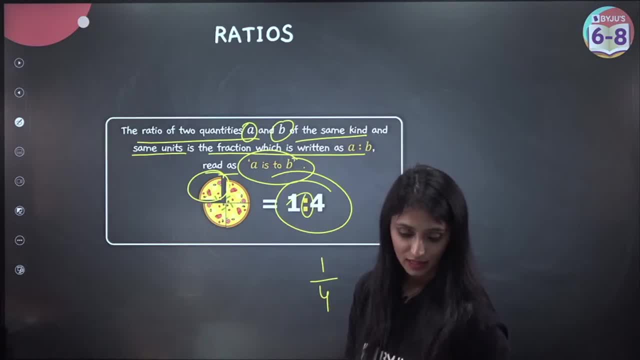 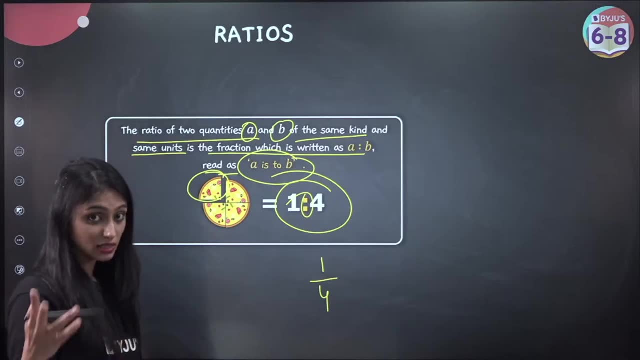 right Apsara. yes, Kiran, exam bilkul free hai. chalye aap check kar yeh proper criteria class ke baad, jab classes aaj over hoten. please do check it. Aakash Ante site pe jaake pehle register kar yeh and then check it. 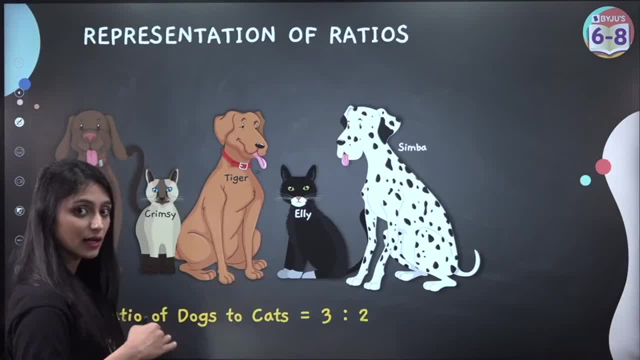 chalye, let's move ahead aur ek tarika dekhte hain, jo hum baat kar rahe hain, ki ratios ko kaise represent karte hain. yaha pe we can see kitne cute cats or dogs hain. I am sure yaha pe bohot sare pet lovers honge right Tuffy, Crimsy, Tiger, Ellie, Simba ya. 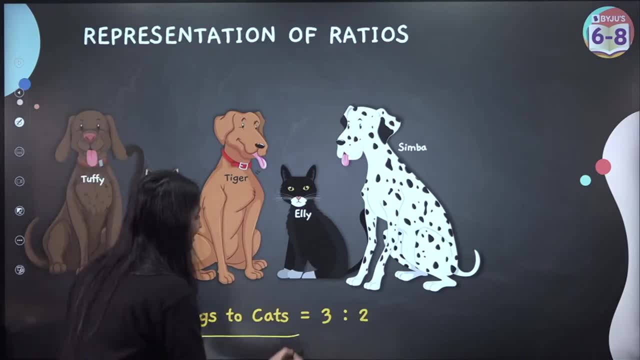 acha, agar mije ratio of dogs ko cats nikalna hai, toh yaha par yeh 3 cute se dogs hain, so 3, aur yaha pe 2 cats hain, so 3 is to 2, that is going to be the ratio right. aise hi dikhayenge yes. 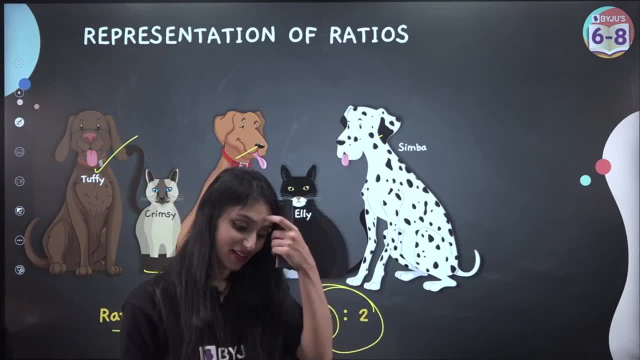 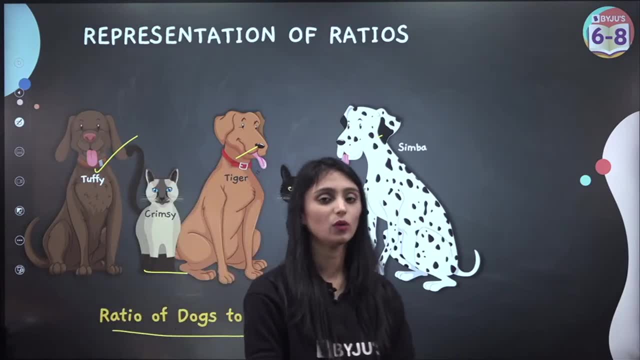 yaar Ante ki upar jo log mujh se pooch rahe hain, na ki ma'am ki kya iska price scholarship mein kitna laana hai, jo bhi still in questions hain, I tell you, I think aap log ne wo sessions miss kar di hain, but koi baat nahi. 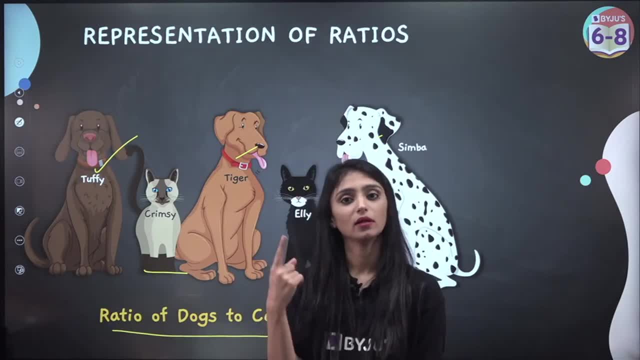 isliye maine kaha, ki pehle register karo, uske baad Akash Ante site pe aapko saara information beta available hai, proper in detail, araam se bedke dekhna. it will take time. bohot saari information hai araam se jib sessions saare khatam ho jayenge. watch it. 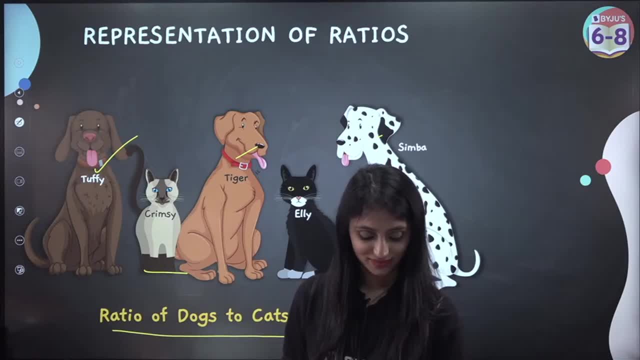 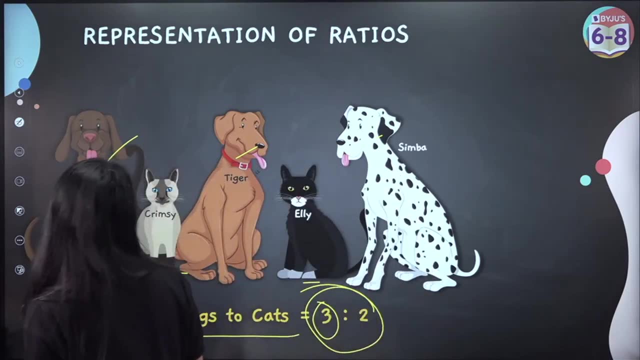 yes, Bhavya, Kaju, you have a dog blue colour. yes, Aadna Bhavya. ok, ok, ok, so this is what this is. 3 is to 2, this is visible right. cats to dogs. 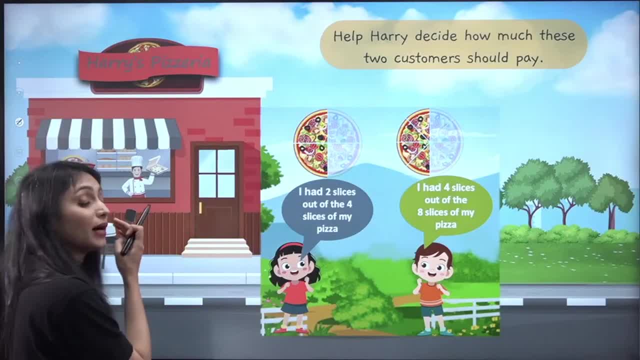 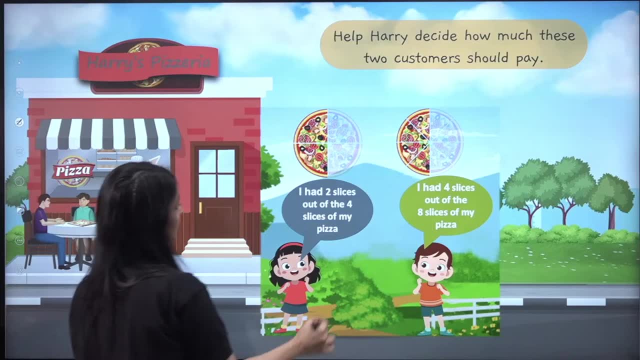 dogs- I mean dogs to cats- ka ratio chalye ab. hum baad karte hain dubhara. se aap dekhiye Harry's pizzeria pe, there are 2 customers right. one customer had eaten 2 slices out of the 4 slices of pizza. 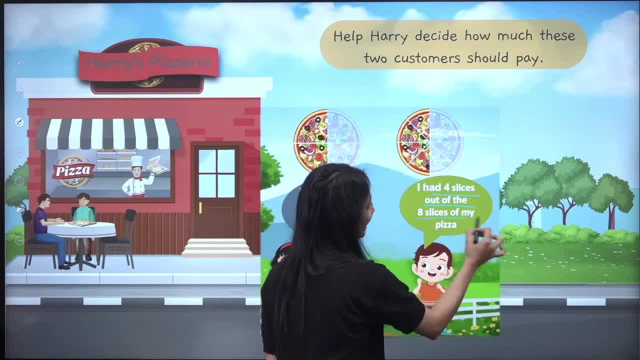 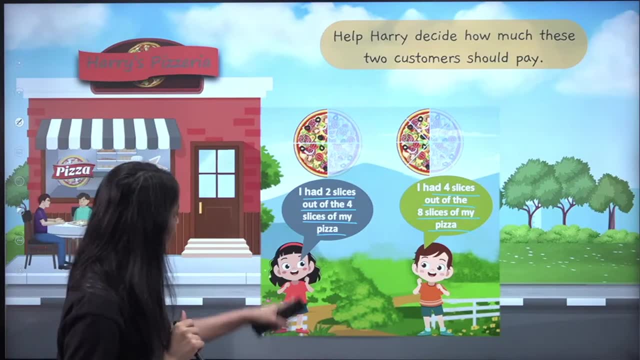 another one has eaten 4 slices out of the 8 slices of pizza. ab. ek question aata hai, Harry, ke mind me ki how much each of these customers should pay. is customer ne 2 slices khaye hain? is customer ne sirf 4 slices khaye hain, 8 pizza ke? 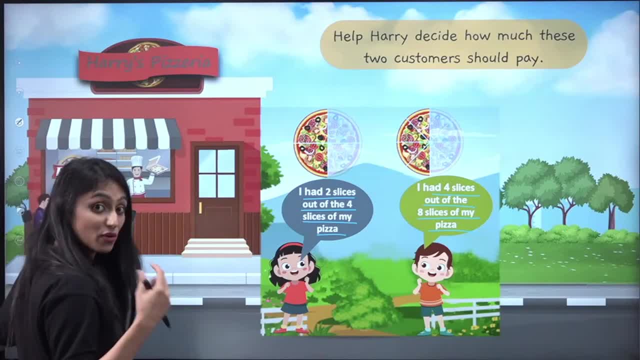 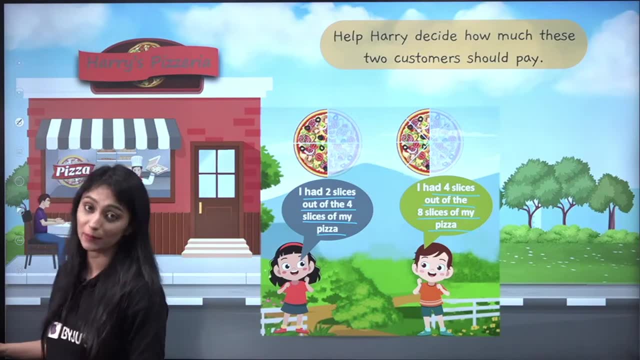 so har ek customer ko kitna-kitna pay karna hoga for the number of slices that they have eaten? bataa sakta hai koi for the number of slices that they have eaten kitna-kitna pay karna hoga? come on answers, answer, answer, answer. thoda, aap isko dekhiye. 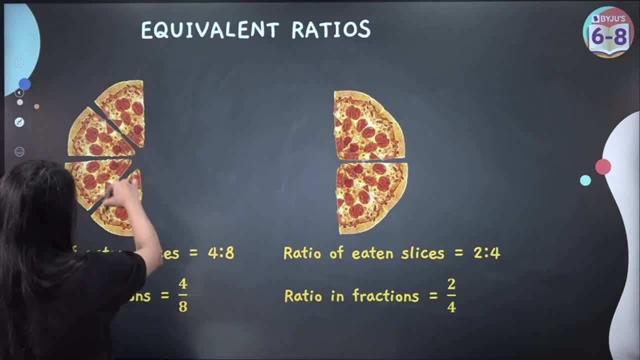 this will help us to understand better. each pizza ke andar 4 slices bache hain. that means baaki ke 4 slices kha liye hain, right? so ratio of eaten slices kya hoga? 4 is to 8, fraction mein aap isse kaise likh sakte hain: 4 by 8,. 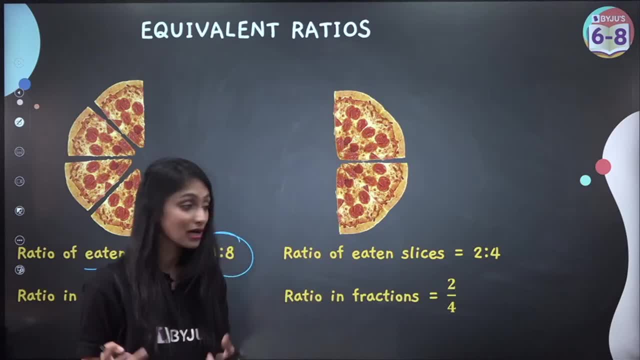 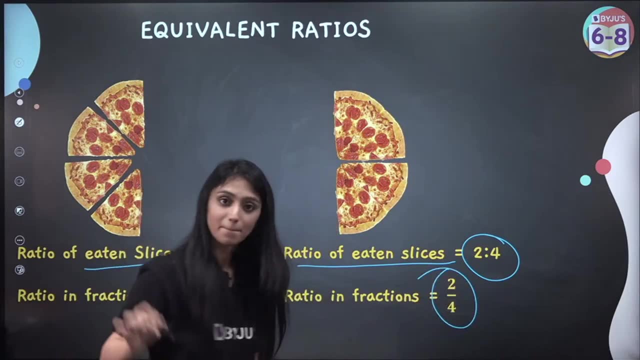 is pizza, mein 2 slices bache hain. that means 2 slices kha liye hain. so ratio of eaten slices kya hai? 2 is to 4, so ratio in fractions. aap kaise likhenge 2 by 4, make sense, right? yes, Dhaniya, yes, yes, yes. 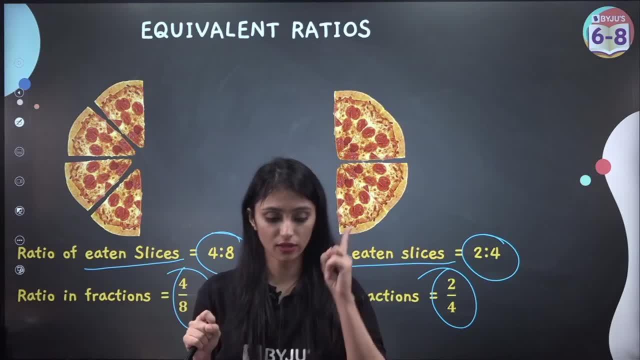 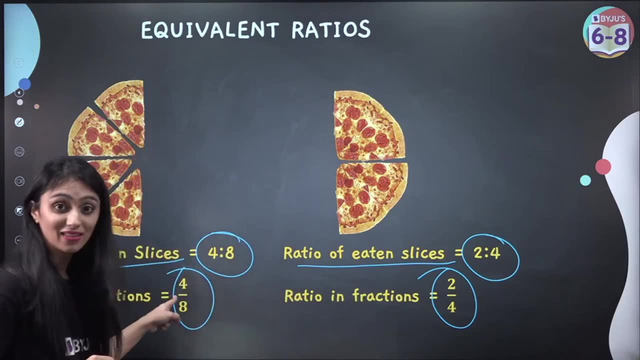 for anthe. I will tell you at the end how to resist it and all anthe ka information. last mein, we will discuss abhi right now. let's focus. yes, Dhaniya, yes, yes, yes. so number of slices that they have eaten is 4 out of the 8 slices here. 2 slices eaten out of the 4 slices. 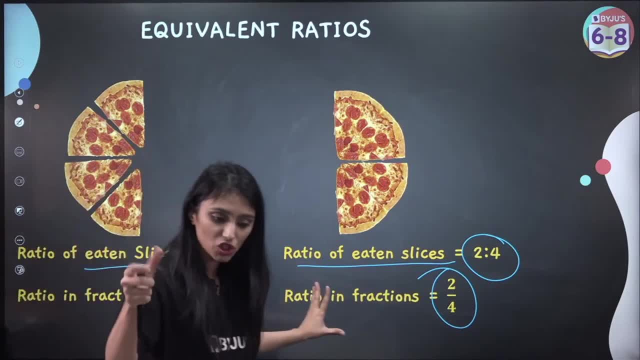 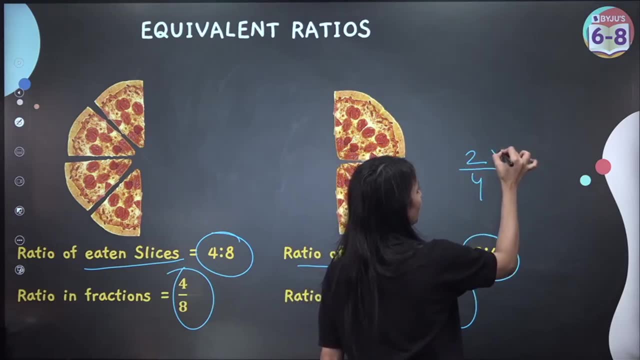 in fraction. you can write this way right. English may be clear. hai sabko. yes, now try this out. isko, can I write this way? can I say 2 by 4,? I will multiply to make it 8,? I will multiply here with 2, so I will multiply with the same number in the numerator also. 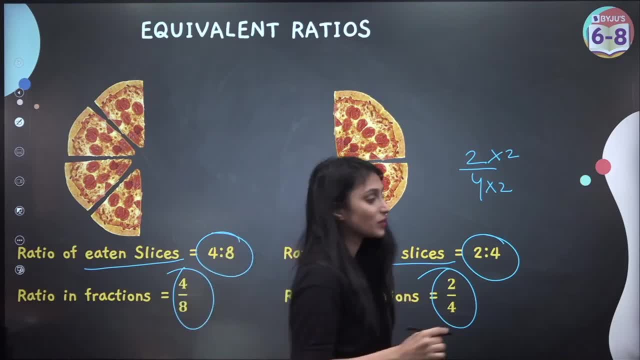 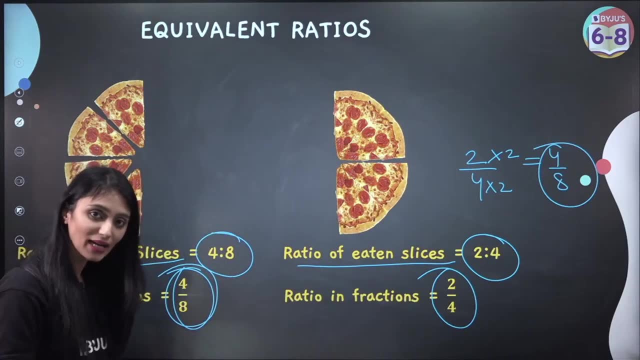 numerator denominator mein, we will multiply in the same number, right? so that's going to be 4 by 8, so what I see here is, at the end, both of these fractions are same, right, so that means they have eaten the equal amount of pizza. 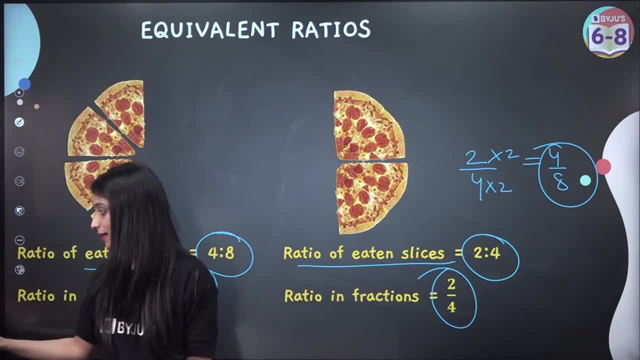 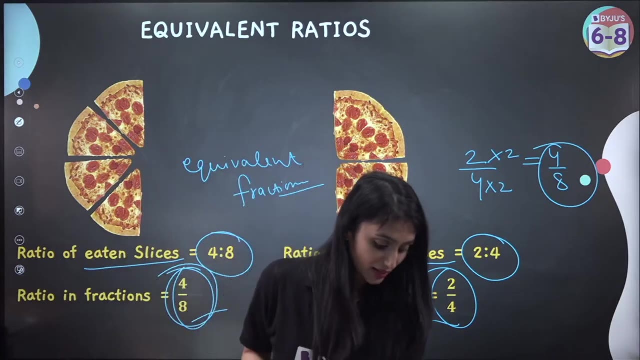 right, we can say yes. so what are these? what are these actually? these are equivalent fractions. what are these? these are equivalent fractions actually. yes, we have learnt about equivalent fractions, right? yes, both are same. right, we can reduce. we can reduce as well. 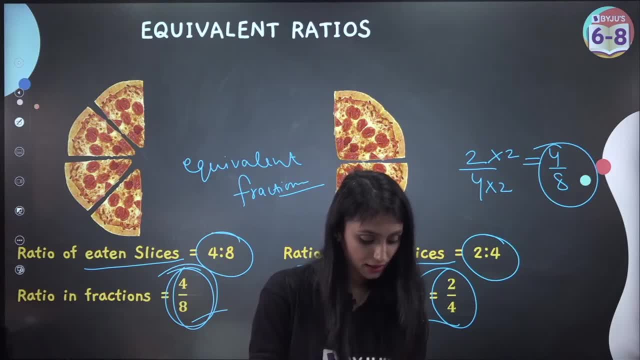 who said we can reduce? somebody said: yes, Harshita, you can reduce as well. if you want that way also, we can do it. also, we can do it. This is the standard. yes, yes, Yes, costa beta at the end. Antica discussion. 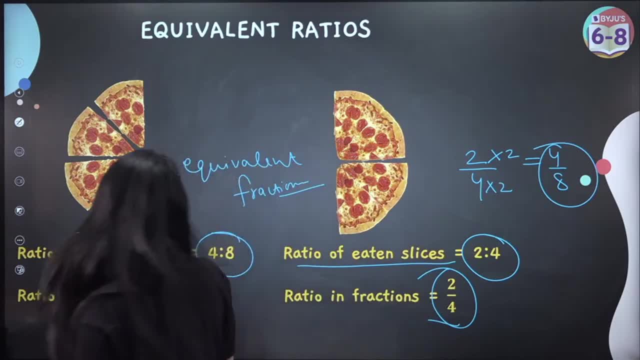 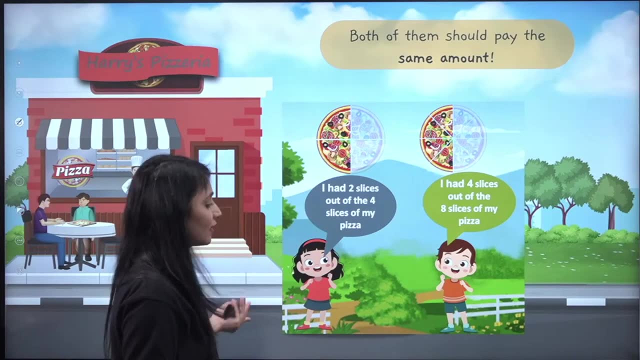 at the end, Simply, we can say: it's okay, Ayesha. Yes. simply, we can say: these are equivalent fractions, So I can say that both of them should pay the same amount. right in that case? Clear, right, because they were equivalent fractions. Yes, Shubh, you will get the notes. 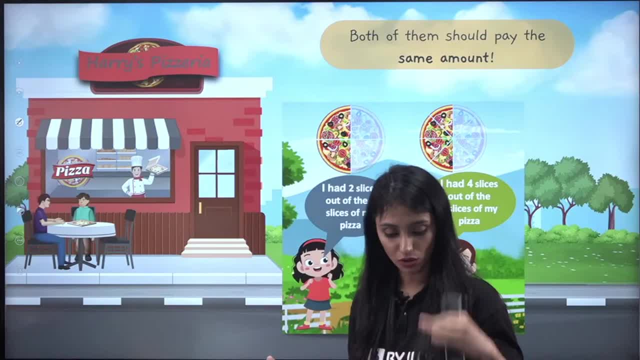 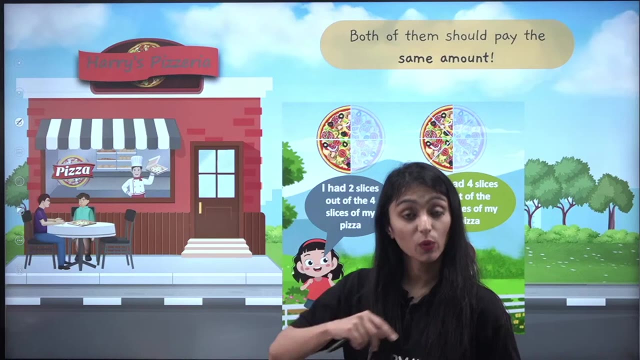 of this chapter- I mean the PDF on telegram channel- may be by today, by the end of today or may be tomorrow, definitely, Yes, yes, Karthik saheb, ma'am in 2 table, not able to understand ma'am in 2 table, a simple form of 4 by 8.. Yes, 1 by 2, it's much more. 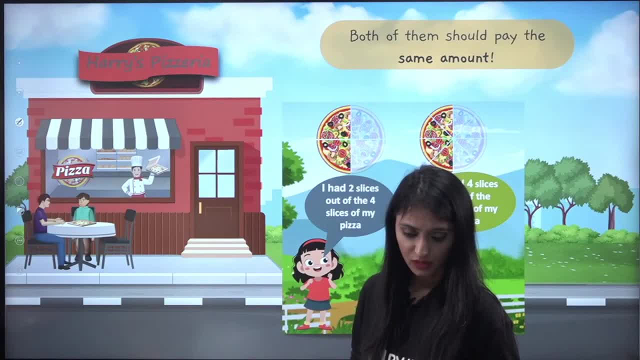 simplest form, I would say: right, Yes, it's not necessary, though it's not necessary, but you should always write them in simplest form whenever you know, when you are giving an answer. Yes, Srishti, you can ask. you can ask very nice, Kushagru, what if ma'am is? 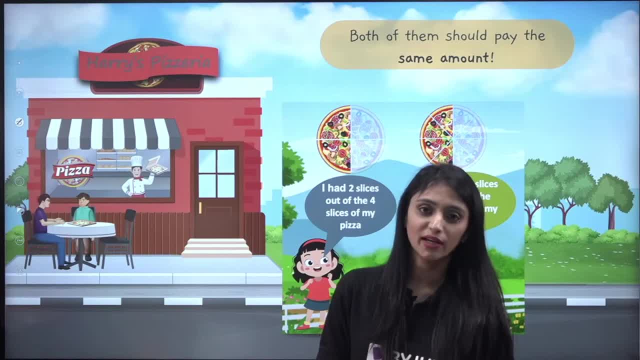 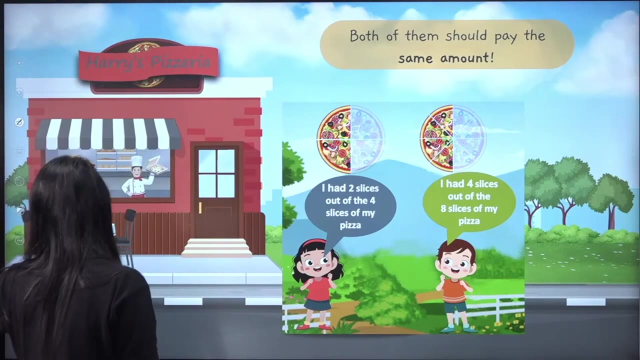 pizza is of different type? What if one is margarita and one is a non-vegetarian pizza? What in that case? Yes, yes, Chalye, let's move ahead so we can say: both of these were So. now we have a good understanding about equivalent fractions. let's try out this question. 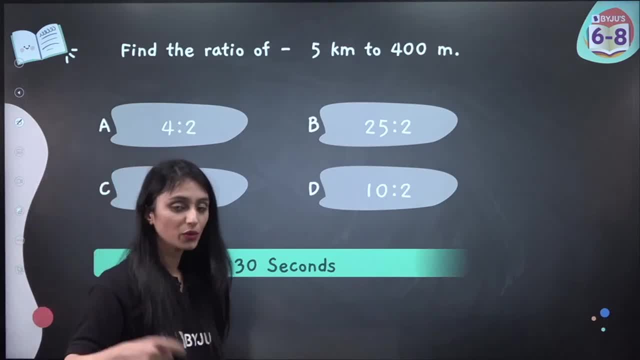 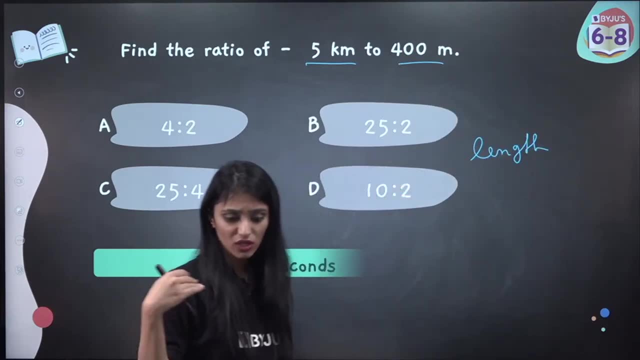 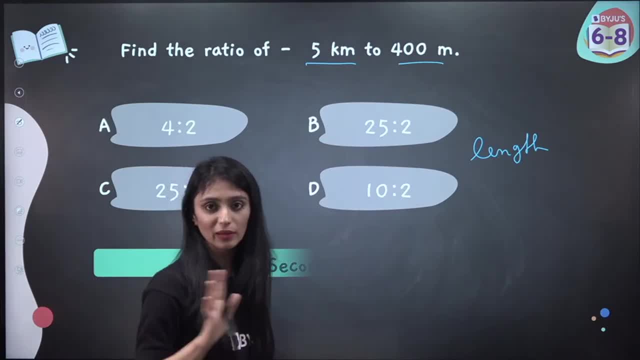 they have the same length. You think they have same length, aren't they? Please write in chat. I can obviously see properly from here, but you tell me Visible blue colour is visible. both of these are length. they are of the same kind, both of them are length. 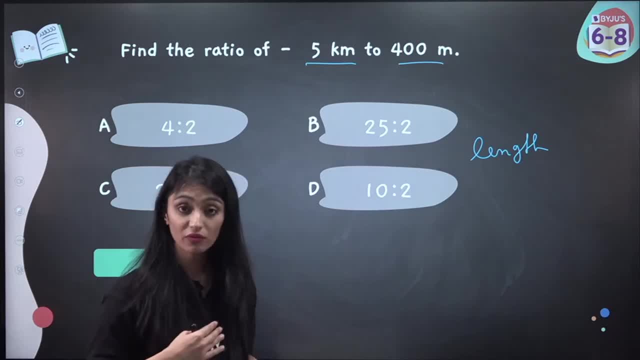 They should have the same units. whenever we are talking about ratios, whenever we are comparing them, They should have, they should have same units. Unit toh same nahi hai. unit toh same nahi hai. how do we find this out? Yes, clearly visible, great. How do we find? 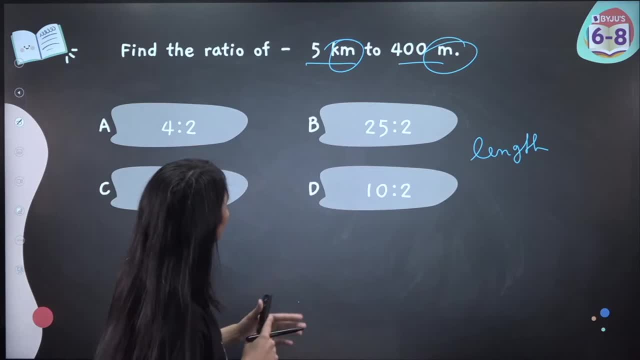 this out Unit. toh same nahi hai. Bilwa sahe, five is to four hundred, five is to four. This is not in the answers. Yes, Shivangi, I am seeing you here after a long time. Exams are going on. Stuti Nilaksha gaming. come on everyone. Ma'am convert. yes, very good. 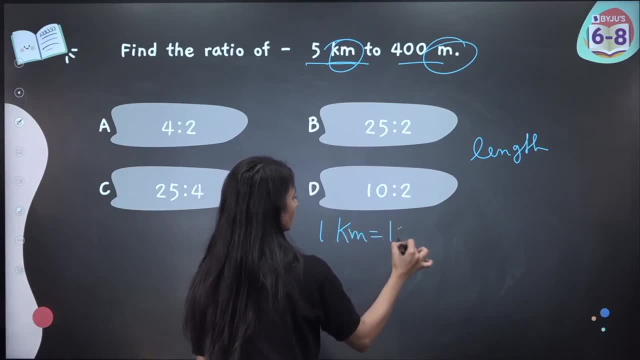 Let's convert kilometre to metre. We know that 1 kilometre is equals to 1000 metre. That's why I emphasized on this thing: length, same kind, same units, Units ko same karo. So 5 kilometre is going to be what? 5 kilometre is going to be 5 times 1000 metre, That's. 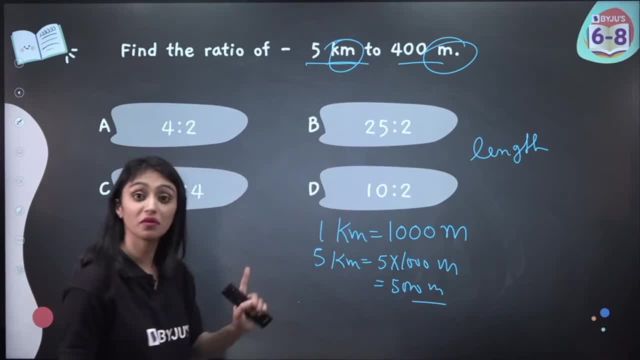 going to be 5000 metre Abhi. toh sko convert kiya hai. Now let's write them in ratios, So 5000 upon 400.. Units are same. toh obviously cancel out hi ho gaya. Ye cancel, ye cancel. 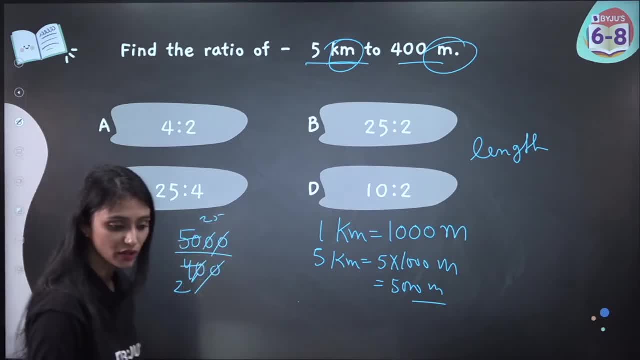 This is 22000, 225000.. Further toh nahi ho raha. We cannot reduce it anymore. Yes, that's going to be option B Aare. yes, na, Gendra, I didn't see that chart. abhi dekha, You were the first. 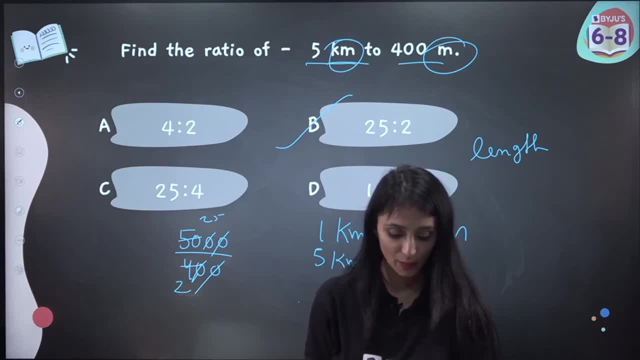 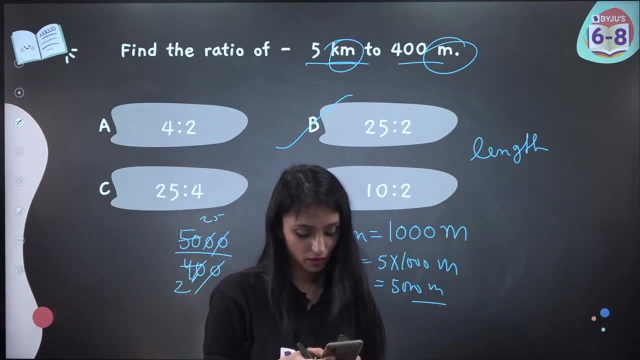 one Chalo badiya Clear Aram Athar Vaisya Bilwasai Shubh Mane Ajayat Clear Vignesh. Mahi Mahi is saying: ma'am, okay, sorry, I missed the comment. No problem, no problem, Sauravi. 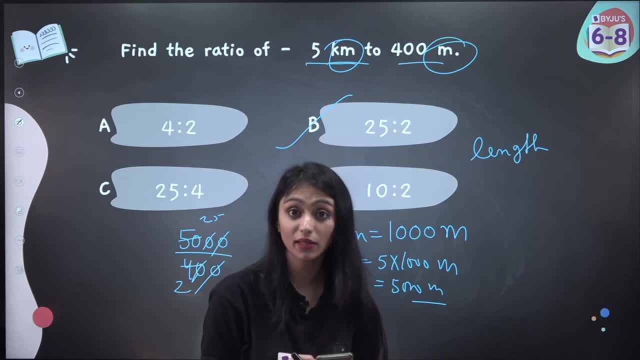 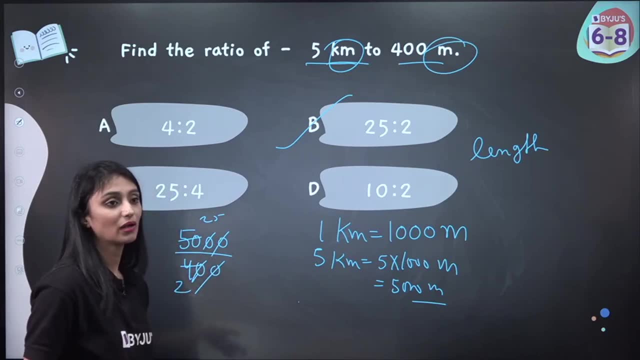 Ma'am, what if the quantities have same units but are of the same kind? You cannot compare them, Mahi. If they are not of the same kind, you cannot compare them Right. How do you? how can I compare, let's say, let's say, if I have to compare height with the amount of 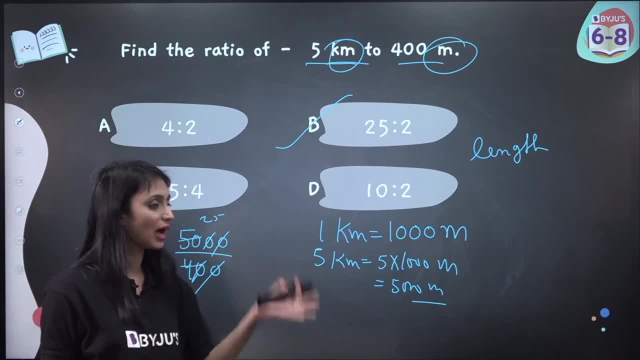 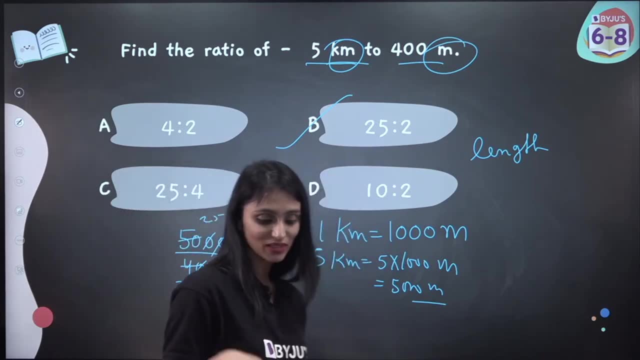 money. There is no comparison. Aap kaise compare karo hi kisi ki height ko with the amount of money? the other person has Right, Comparison toh nahi hai. Comparison toh same kind pe hi ho sakta hai. Yes, Amritansh done Anmol Pro Ek aur cheez. 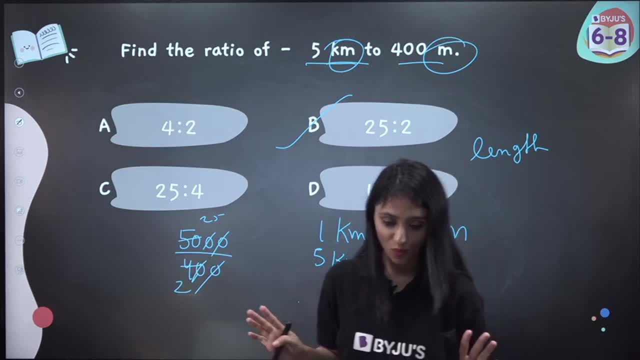 bohot saare mujhe yaha par new names dikh rahe hain, abhi bhi MO, HC, TC, ELCO, Anmol, Pro. Yes, Please, fada vatsa. new students, please first subscribe the channel. I don't know. 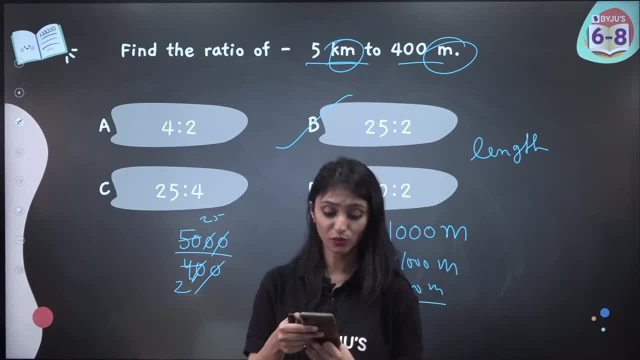 if you are coming for the for my class first time or if you are new to the channel. If you are new to the channel, please first subscribe. and how is this possible? Zyada log session dekh rahe hai likes come. This is not fair. Yes, S Nagendra, they can be compared. Yes, 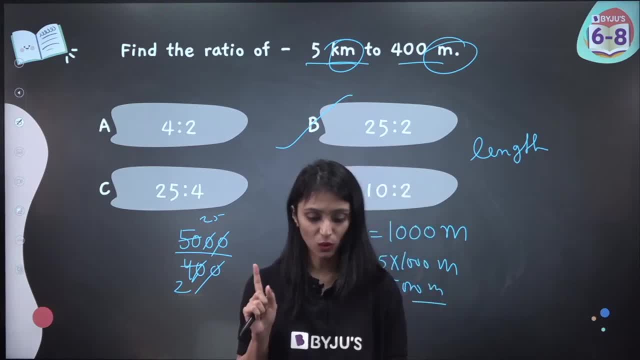 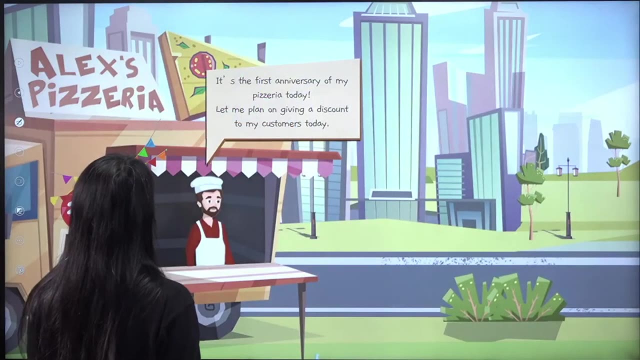 can be compared after conversion. Bilkul mane Ajit: absolutely Only same things. You are old. Meera Gupta. All the new students, please, it's for all the new students. please subscribe Yes and hit the bell icon also. Chalye, let's move ahead. This is the right. 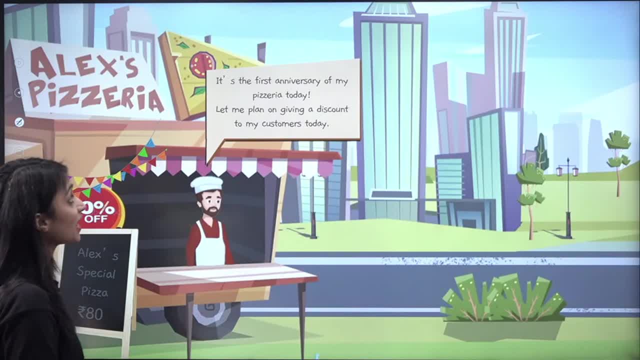 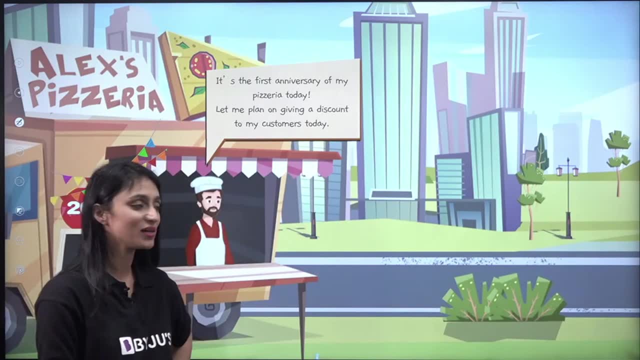 answer. Now, what is this? What is happening? This is the first anniversary of my Pizzeria today. Wow, Let me plan on giving a discount to all my customers. Wow, that's amazing. kitna amazing hai, yaar, yeh Pizzeria. Yes, humare sath toh aisa kabhi nahi hota ki hume discounts. 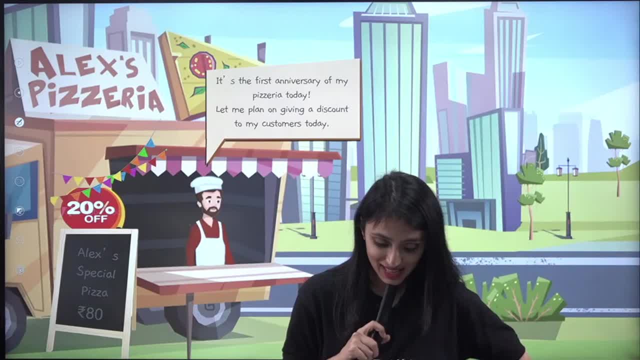 mil jahe nahi. Yes, hi, Naina subscribed. yes, thank you, MS vlog and creation Bitta, I just saw your message. abhi Aisa kuch nahi hai. Varshwata ki kaha fraction use karo? Question me clearly. 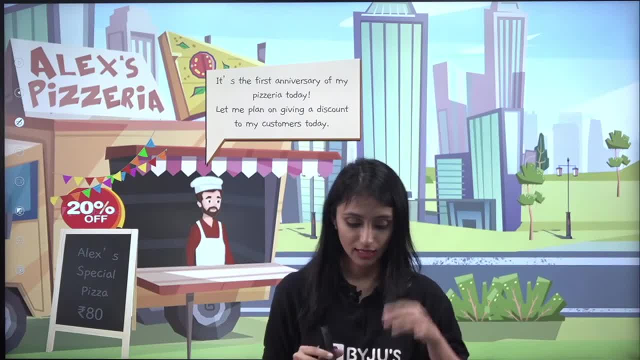 mentioned hota bitta. Abhi we will try out questions na you will understand Chik hai Alex aa hi jaata hai right, And this is Alex special pizza 80 rupees ka hai Areh waa Now. 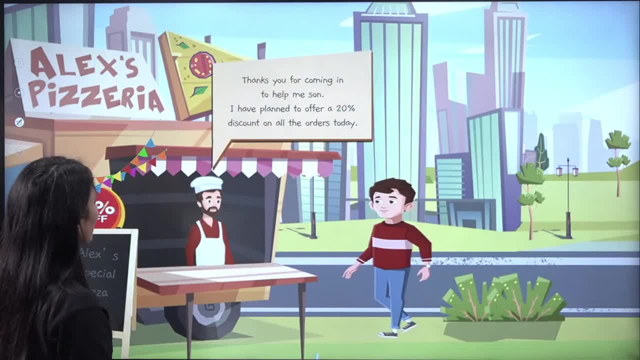 let's see this. So Alex kheh rahe hai, Alex ke father kheh rahe hai. thank you for coming to help me, son. I have planned to offer a 20% discount on all the orders today. 20% discount, hi toh. 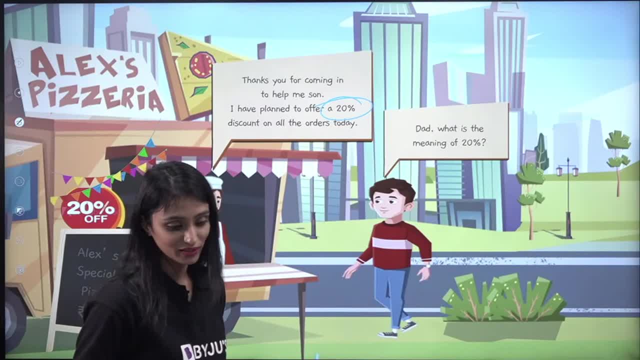 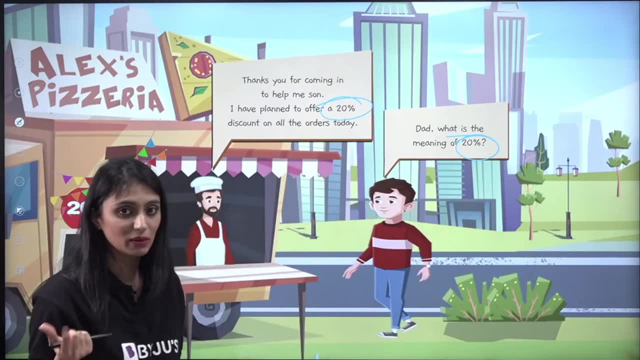 online orders pe milta hai. normally toh aise nahi hota hai. right, 20% discount mil raha hai. Haan 20%, yaar, it's good. He says. dad, what is the meaning of 20%? Alex ko 20% nahi? 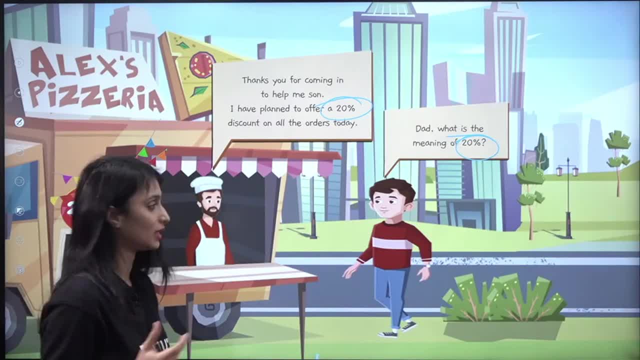 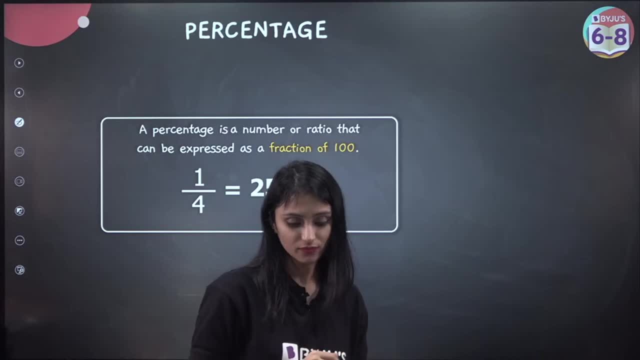 pata. he knows 20,. he doesn't know what 20% is actually. So let's help him understand. Now we will talk about percentages. Yes, no, not much difference. not much difference, Jyoti. So aapne usko, us form me likha hai, sirf form me likhne, ka difference hai aur. 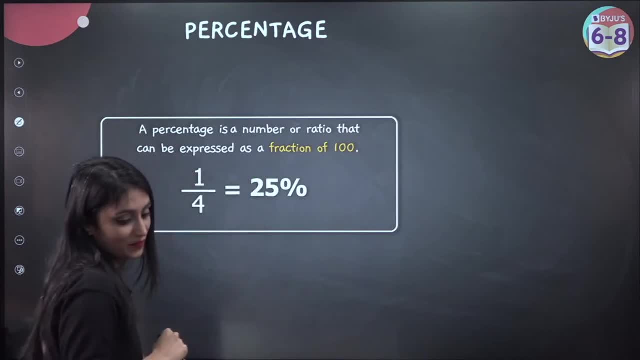 koi difference nahi hai. right, Alright, chalye percentage samashten pehle kya hai. Percentage is a number. it's a number or ratio that can be expressed as a fraction of 100.. Let's suppose, let's suppose hum one by four ki baat kar rahe hai. fraction of 100, kya? 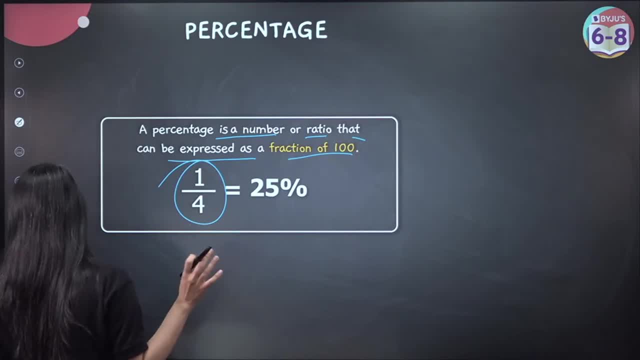 matlab es baat ka As a fraction of 100.. Kya matlab es baat ka? As a fraction of 100, as a fraction fraction of 100 ka Iska matlab ye hai ki a percentage is basically numerator hoga. 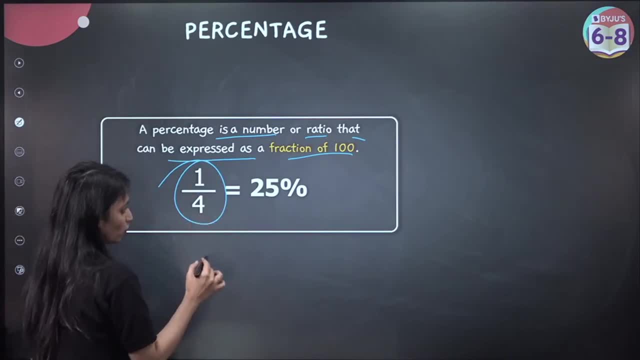 numerator hoga of a fraction whose denominator is 100.. 1 by 4, ko aap 25% likh sakte hain. kaise likh sakte hain 1 by 4, 25%? kaise banta hai? We will understand this in the upcoming. 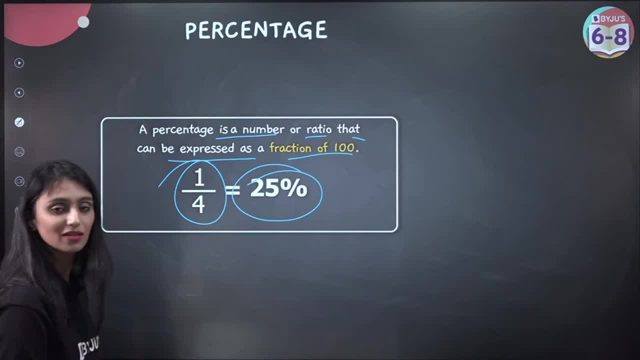 slides: Tanishq, ratio of fraction mein Beto koi khas difference nahi hai, sirf likhne ka difference hai right, Yes, Oh wow, 20% of MRP of pizza. very nice, Ab jese, let's. 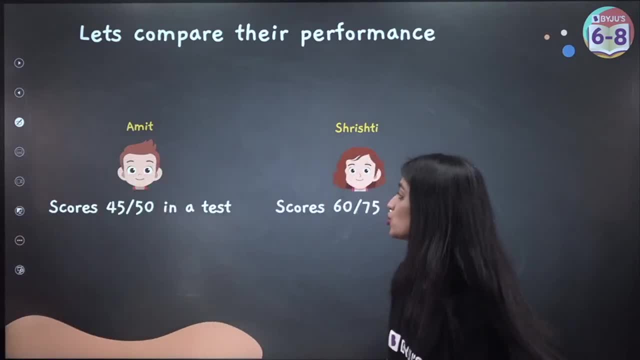 suppose I want to compare the performance of 2 children Like Amit and Srishti. ne score kia Amit ne 45 on 50 in a test. Srishti ne score kia 60 on 75 in a test. How do I compare? 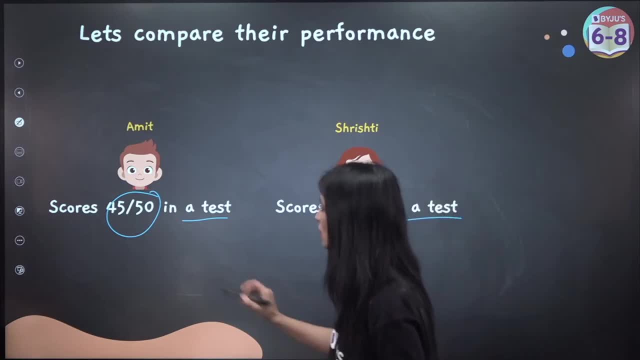 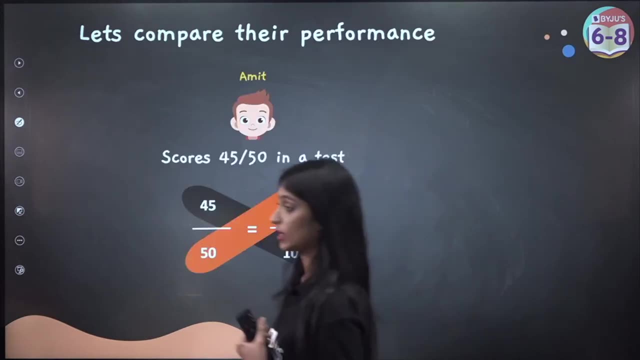 kisne acha score ki hai. Comparison mushkil hai. Reason being yahaan pe denominators bhi different hai, numerators bhi different hai. comparison mushkil hai, and that's where percentage comes into picture. Ye, thoda simple ho jata hai. As I said, a percentage is basically the numerator of. 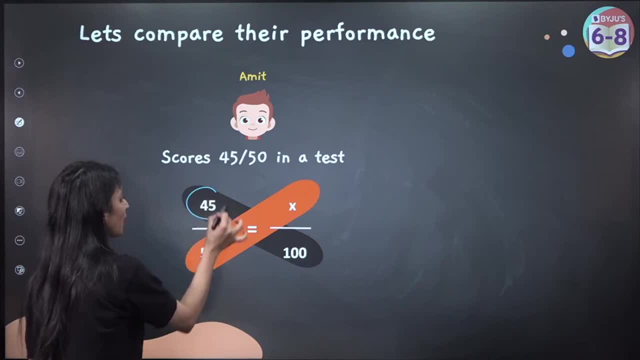 a fraction whose denominator is 100.. To 45 by 50 ko, if I want to write in percentages. so kia hota hai. maine kaha tha it's basically a numerator of a fraction. ek fraction ka numerator hoga whose denominator is 100, right Ab isko simplify, karte hain cross multiply. 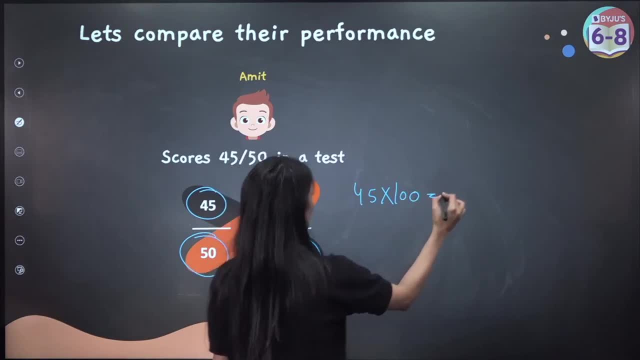 What do you get? 45 into 100 is equals to 50 into x. theek hai Ab hum kya karenge, 50 ko yahaan layaate hain. 45 into 100 upon 50 is equals to x. abhi ho gaya. cancel out. 50 ones are 52s are 45 times. 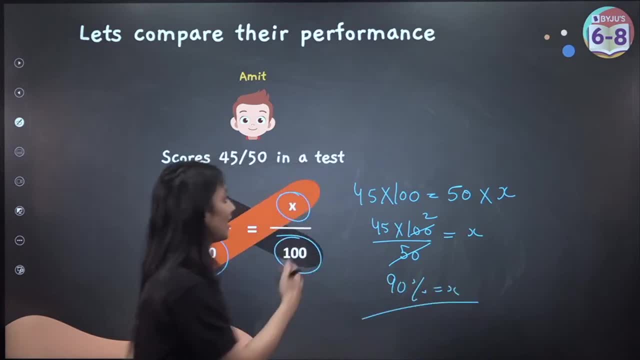 2 kitna hota hai 90.. So yaha x ka value kia hai 90%, Toh Amit kia hai 90% marks. Bilkul. yes, maane Ajit, yes, Arre direct inverse proportions. don't worry, Woh bhi lag gaya yahaan pe 90%. 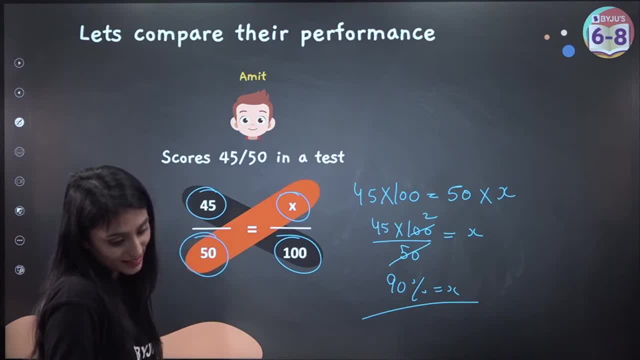 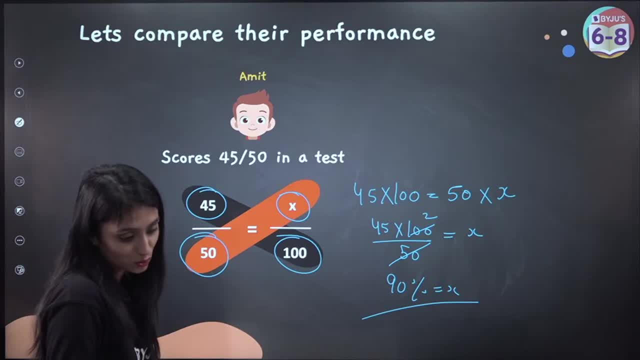 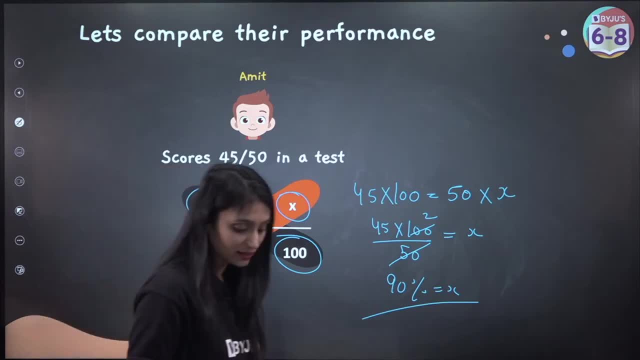 please everyone. Sandhya Robin, lot of new students are joining the class. I don't know if you are coming here for the first time. channel pe new hai ya class me first time hai. please, if you are liking the session, fada bache yaar jaldi se agar session samaj. 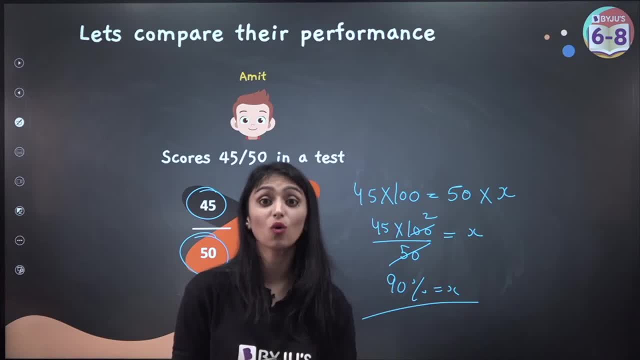 aara hai sare concepts, samaj aara hai jaldi se like bhi karo session ko and, don't worry, practice session bhi lekar aayenge, jisme hain sare questions discuss karenge, NCRT ke bhi. Yes, just like we did sessions on weekends, is weekend bhi karenge. 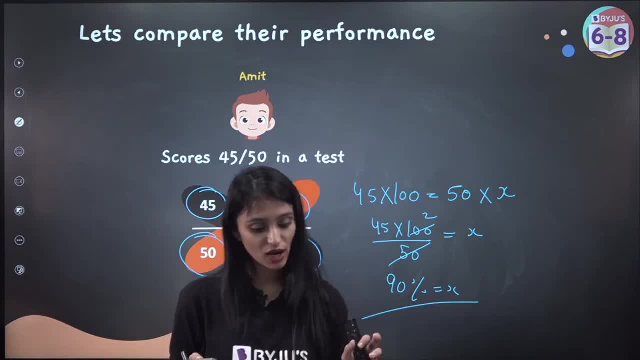 And you know that it's very fruitful. right Sare questions. we can practice. yes, Sonakshi, you can ask pitta, jo bhi nahi samaj aaya. Comparison using LCM also. yes, bilkul, kar sakte hai comparison using LCM. but I tell you one thing: percentage is a better way. 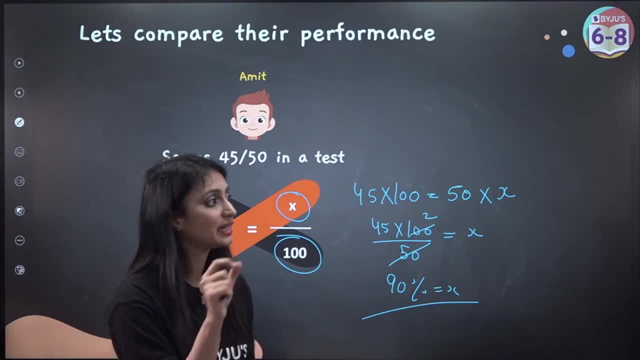 to compare something right, Because aap aise dekhenge, yeh greater hai right. Lekin aap yeh nahi bata sakte. aap check karoge kitna difference hai yeh 5 marks zyada hai kitna. 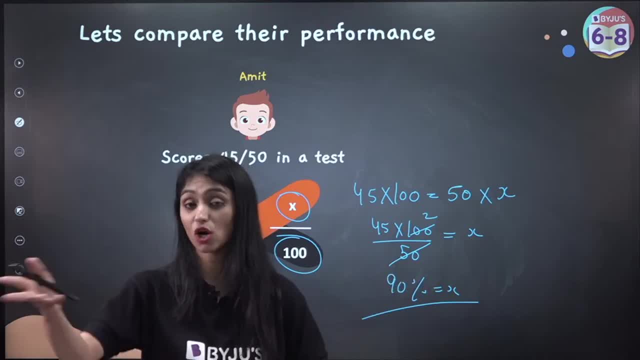 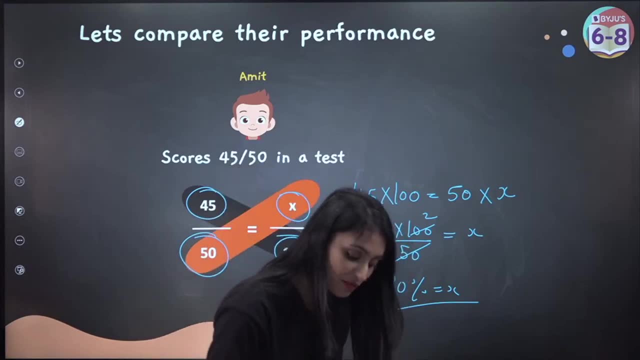 but percentage me usko batana zyada better hota hai. he has got 95%, he has got 90%. aise comparison is much better. Yes, if you are liking the session, if you are enjoying the session. quickly, everyone. 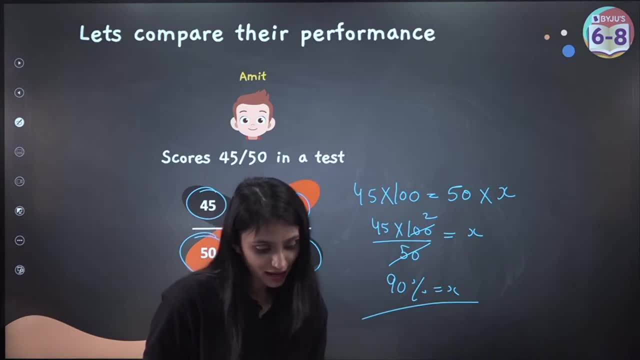 fata fatse, like bhi karo, like karo session ko hi Kailash Chandra Meera Srishti, maine abhi just abhi dekha. I don't know why this is happening with you today har baari mai. 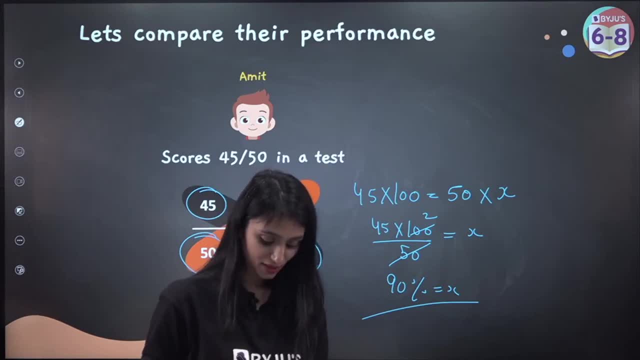 jab dekhti hu, yehi message aata hai. ma'am, you are not seeing my messages. yes, Dipti Bhalla, you can ask hi Nalini Yadav. yes, Mane Ajit, nice, nice Full name, kiska full name. 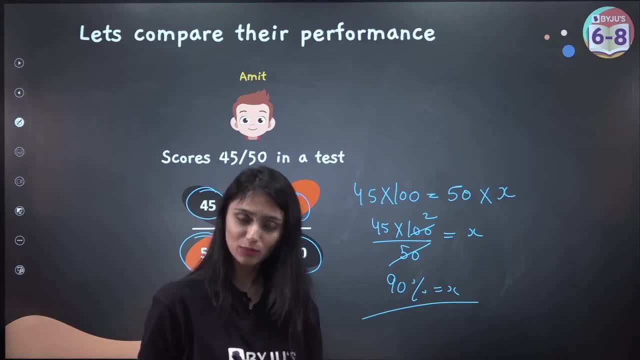 Kaustubh ka. Kaustubh ka full name mujhe kaise pata hoga. toh Kaustubh ko batana padega. hi Priyanshi 1k likes bante hain very nice. thank you, Deju. come on everyone quickly, ma'am will move. 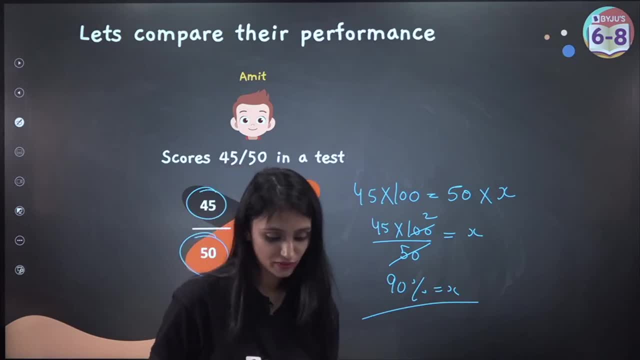 ahead to the next slide only when you will give me 100 likes. chalo fada fatse. My full name? oh, I did not introduce myself. my name is Khushboo Kohli. now don't say, ma'am Virat Kohli, aapke relation mein hai aisa kuch nahi hai? no, not at all. Scholarship wala. 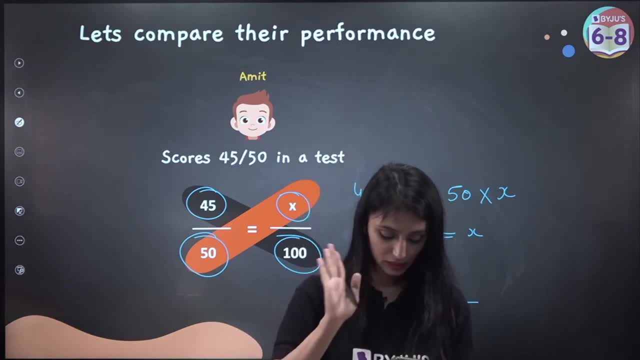 ANTHE ka jo bhi information is not there. no, not at all Scholarship wala ANTHE ka jo bhi information chahiye. end of the session. we will. we will discuss. yes, come on, everyone chaldi se. 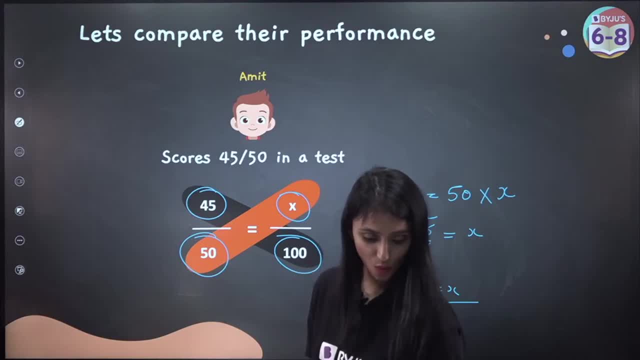 Emo HTC, HCTCLKO Kailash Chandra. thank you, Isse pehle question aata maine isli khud bata diya Bhavya. Come on, everyone fada fatse like the session and jino ne subscribe. 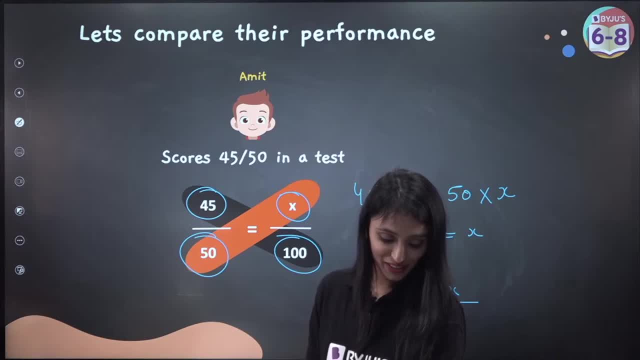 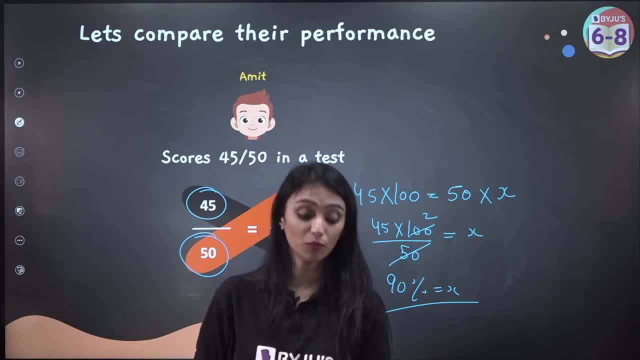 bhi bhi hai. Yes, of course, Nazrana, class 8 ke sessions bhi bhi hai. Now I think Nazrana has come from everywhere. See, agar aap logon ko koi bhi- I think, Nazrana, you are coming here for the first time- Koi bhi doubts hotei. 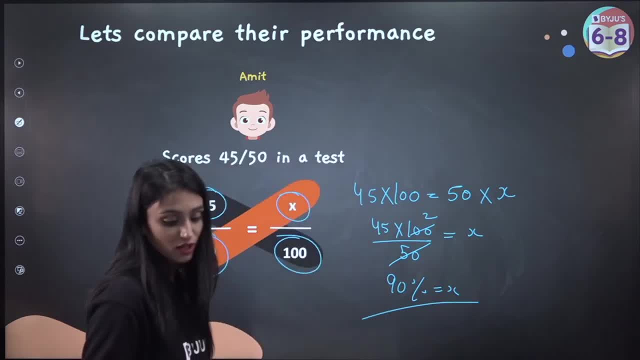 the session ki yeh sab samajh aara hai. achcha session hai. Hi Gaurav Sarana. all the new students please subscribe: 99.5, arey baah, so percentage is a good way, nahi apne marks. 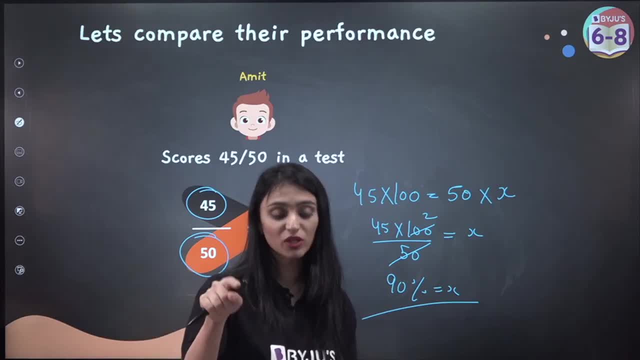 batane ke liye bhi. Abhi aungi Prisha Prisha Raja ki asking, ki ma'am percentage ko decimal mein kaise convert karein. we have that also in today's session. Virat Kohli is not my. 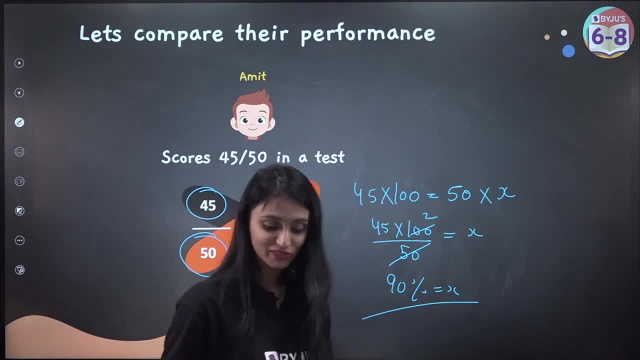 relative iss. se pehle yeh question aata mujhe isli maine pehle bata di: he is not my relative. arey Chalo next chalte hai Shrishti score 60 on 75 in a test Ab isko. 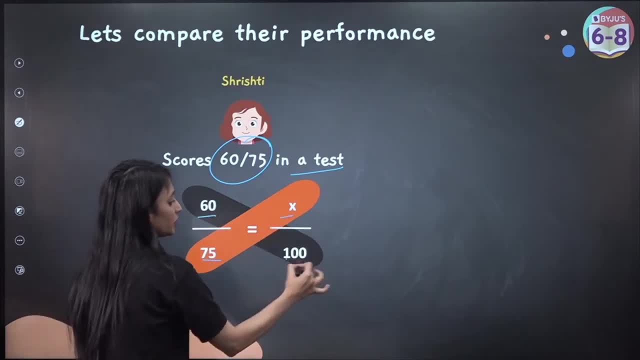 bhi percentage mein compare karke, hum nikaal sakte hai: 60 by 75 equal to x by 100,. right, Chale main iske simple way bhi apko bataungi, kaise kar sakte hai, without writing it this: 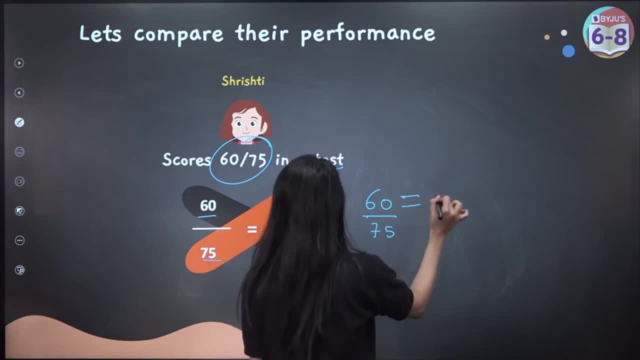 way. So 60 upon 75 is equal to x upon 100,. yeh hai amare paas cross multiply kar lete hain aise. so kya aayega 60 into 100 upon 75, hi rahi nai, tu rakh sakte hai equals. 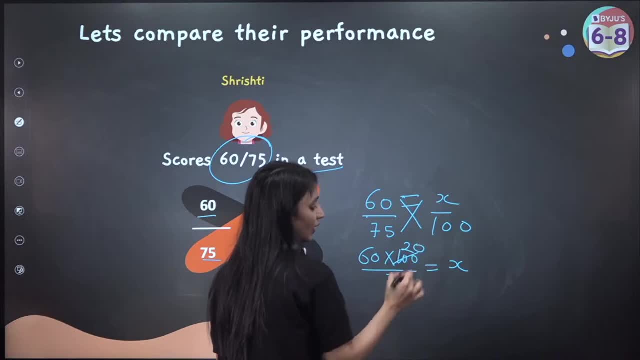 to x. So this is what 5 times 2 and 0,, right, This is 5 times 1,: 5- 5s are 25, 5- 3s are 15, 5- 4s are, and 3- 1s are 3, 20s are. So, kitna aage hai yaha, pe x ka value 20 into 4, that's. 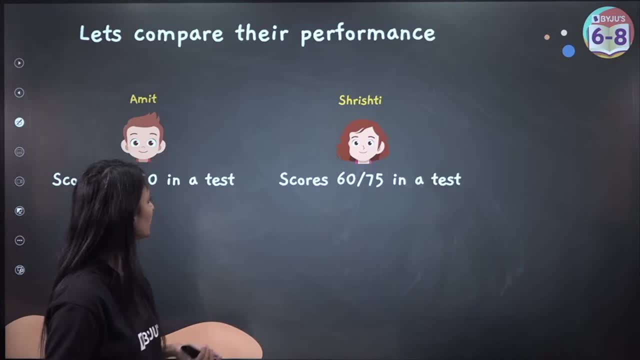 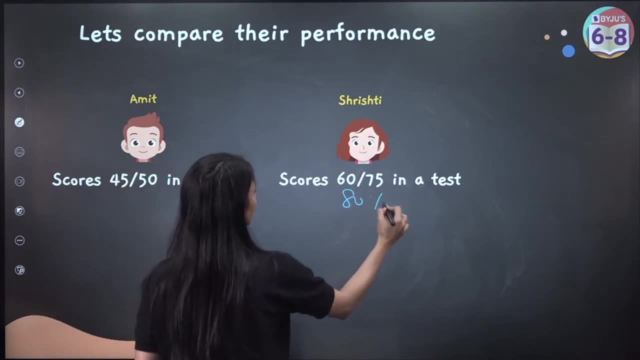 80%. Uske kitne marks aaye, the kitna percent ta percentages. yaad hai sabko kitna aaye tha. that was 90%. Iska 90% aaye tha aur iska kitna aaya 80%. Kitna easily compare. 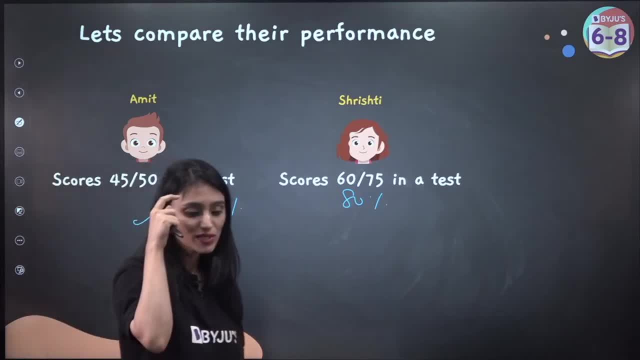 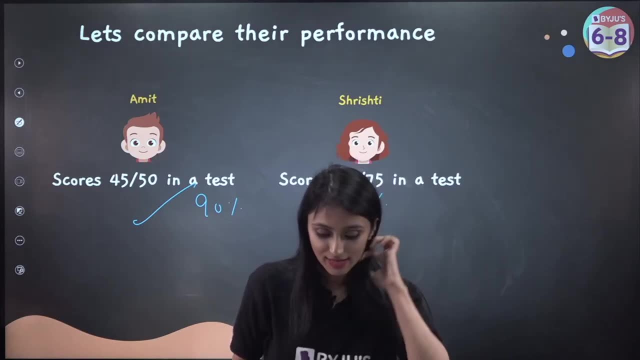 hum kar sakte hai. now we can compare their performance. se iske isne better score kiya. Who said, ma'am LCM, le ke aap check karte? That's a longer way aur better comparison bhi nahi hota, uss case mein. Yes, yes, yes, yes, maane Ajit vilkul Ab hum uss topic par. 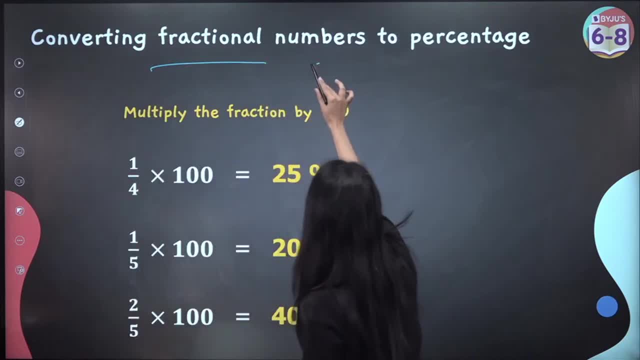 aate hain conversion ki baat kar rehte hain. Convert, kaise kare fraction null numbers ko percentage mein right? Simply, jab bhi aapko fraction se percentage mein jaana hai, fraction se fraction se hume percentage mein jaana hai, to aap kya karenge? simply multiply the. 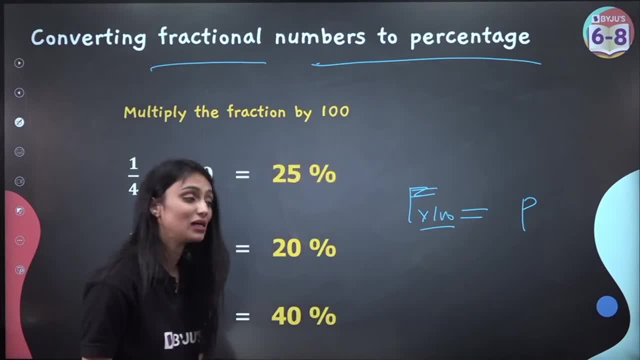 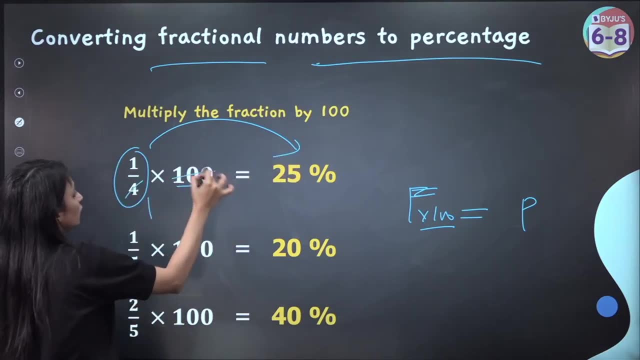 fraction with 100.. Isko 100 se multiply kar dena Jaise mujhe 1 by 4 ko percentage mein convert karna hai. I will simply multiply this by 100.. 4 times 1, 4 twos are 8,. ye kya ban gaya. 20, 4 fives. 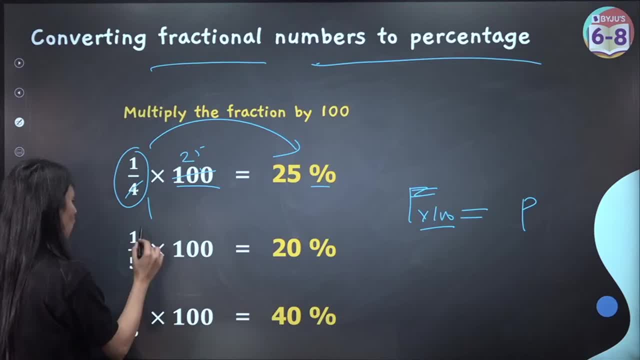 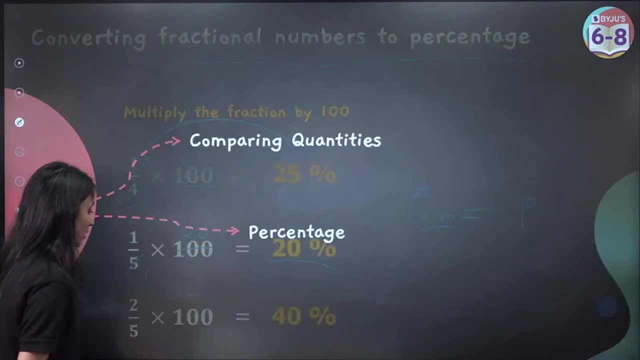 are 20, 25 percent ka symbol lagaate. na, that's it. 1 by 5 ko mujhe percent mein convert karna hai. 5 ones are 5. twos are 20 percent. 2 by 5 ko percent mein convert karna hai. sorry. 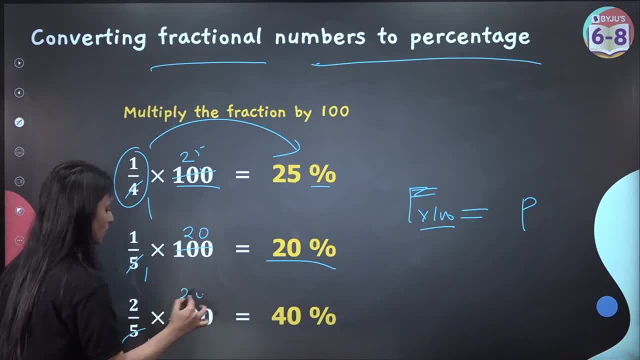 2 by 5 ko karna hai. 5 ones are 5, twos are. kitna aa gaya 40%, simple, kuch nahi hai. fraction se percentage jaane ke liye. yes, abhi aayenge, decimal pe bhi aayenge we. 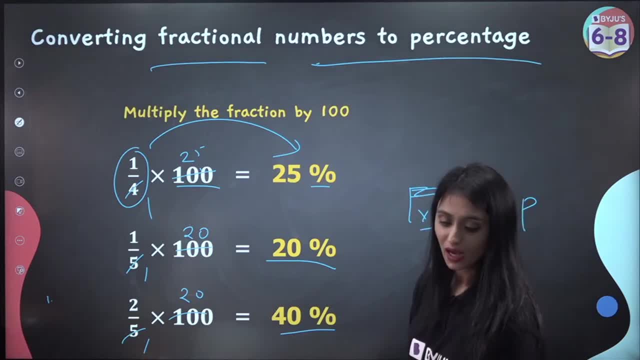 simply multiply by 100, right 100 kyunki hum as a whole leke chalte hai. that's the reason 98.5, arre, waa, waa, Kartik pen colour change karna hai. colour visible nahi. 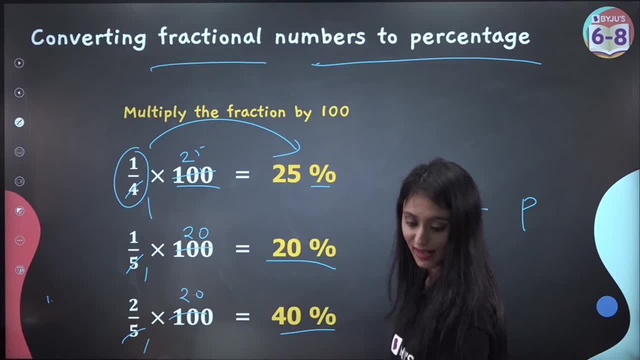 hai. yes, clear, very simple. yes, Anmol Anshy, come on, everyone, sab kuch samajh aa raha hai. yes, likes, likes, likes, like the session also, agar sab kuch samajh aa. 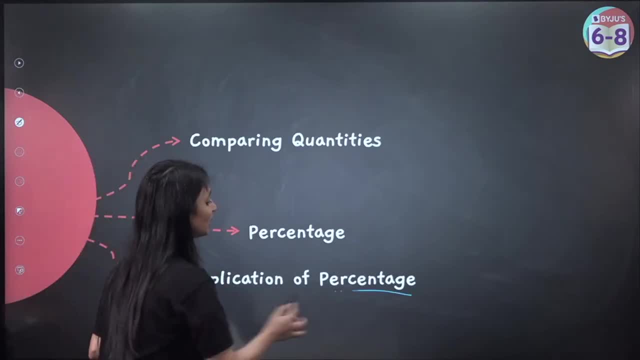 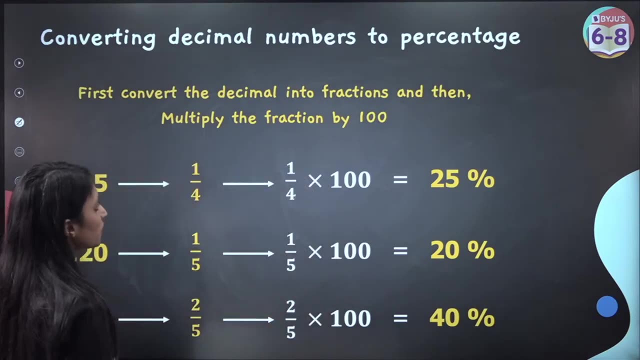 raha hai. chal ye, let's move ahead. now we will talk about the application of percentages. application ki baat karte hain thoda sa aur deep jayenge converting decimal numbers to percentage. first convert the decimal into fraction. simple tarika hai: mirko 0.25. 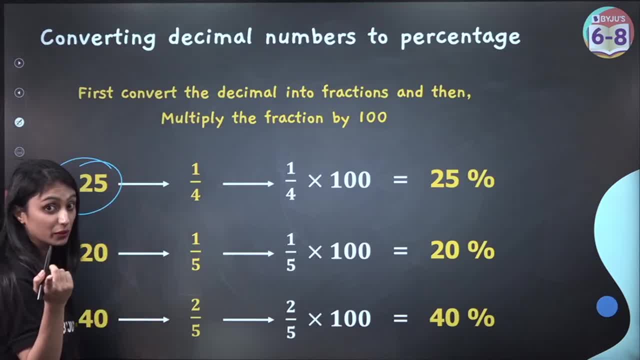 ko convert karna hai main. kya karungi main pehle iska decimal remove karungi. theek hai, dekho, 0.25 ko convert karna tha aap isko simply iska decimal remove karo main aapko. 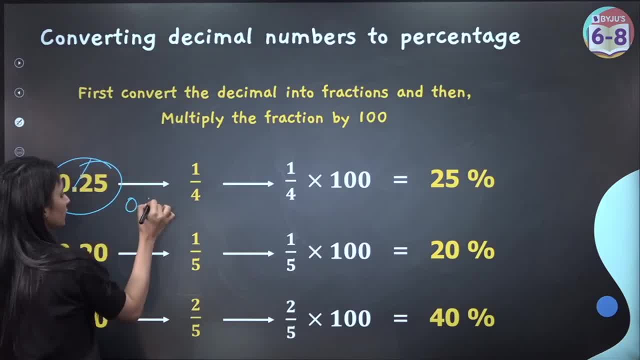 sikhaaya tha, pehle bhi 0.25 ke decimal remove karoge. main haan lagte hoon remove the decimal kitne digits. hai decimal ke baat. there are 2 digits. there are 2 digits. that is why. 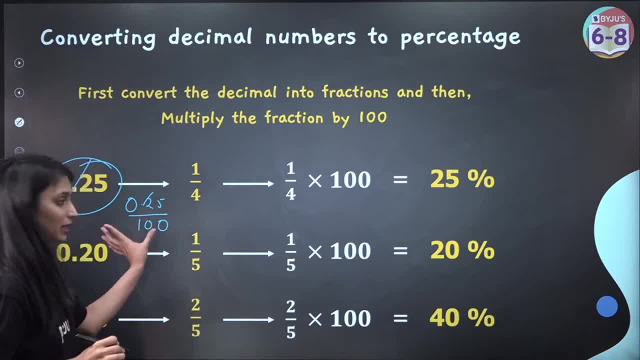 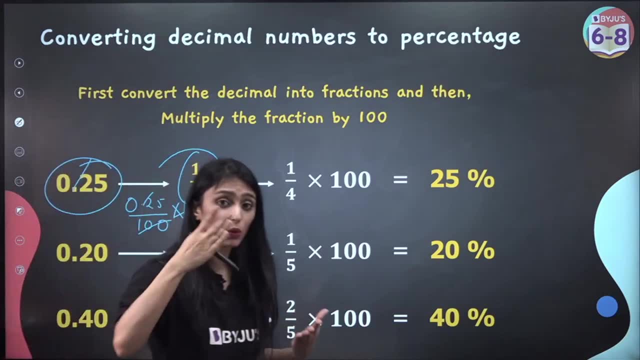 I will write 100 in the denominator. okay, now, simply, simply multiply this by 100, what do you get? 25%, ye karne ki zirat nahi hai har bari ki pehle. we will reduce it and 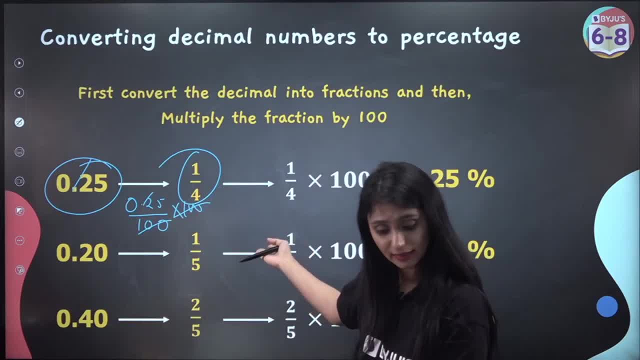 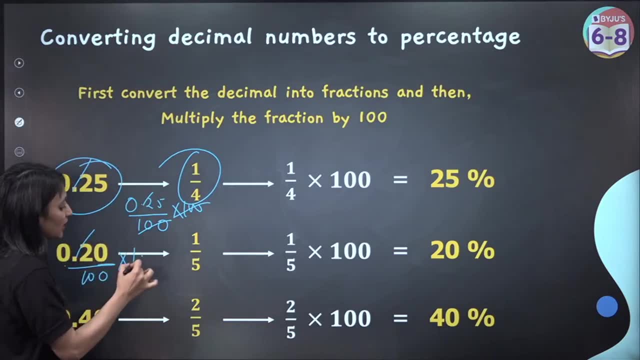 then we convert. you can directly do this as well, so you can do this as well. you can do this as well, right, directly. also, we can do this similarly: 0.20, I will remove the decimal, I will write 100, because there are 2 digits, and simply I will multiply by. 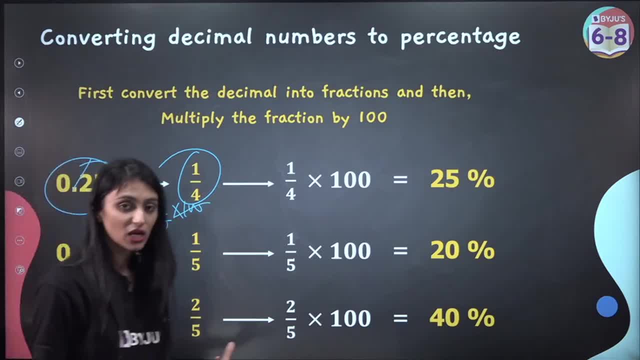 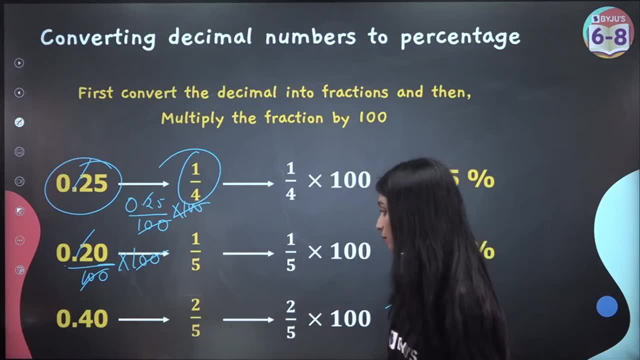 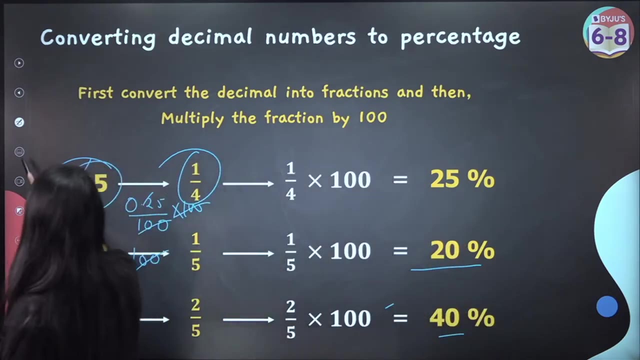 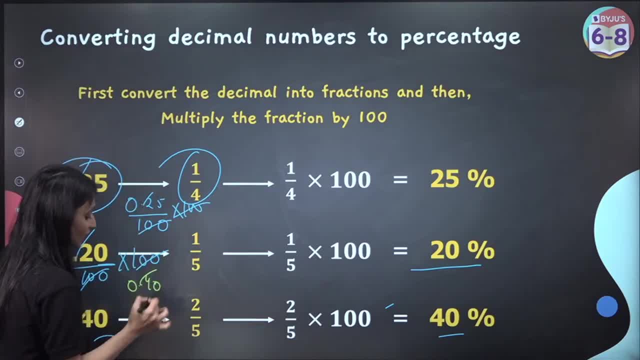 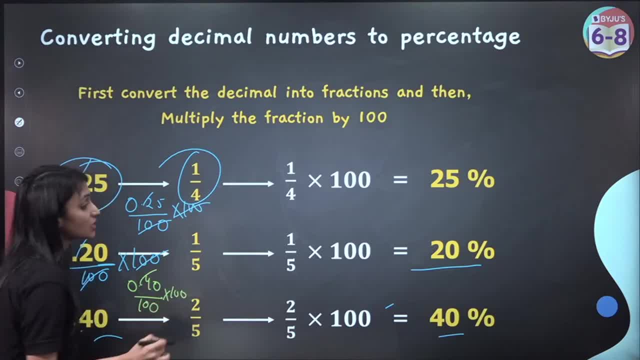 hai agar to mai 0.40 me decimal remove karungi hain. there are 2 digits after the decimal. I will write 100 in the denominator fraction. banyak h dati hai now. simply I will multiply by 100, because whenever we are converting a fraction into percentage, we simply multiply. 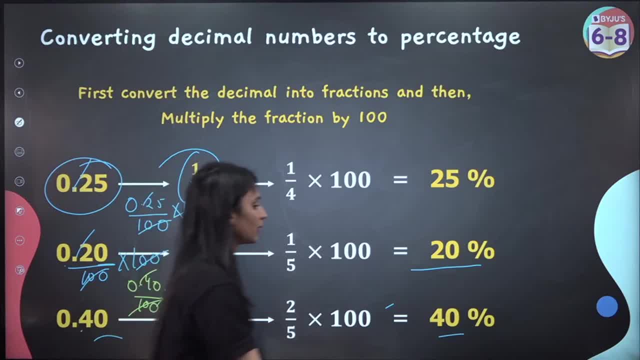 by 100, that's what I am doing here. you don't have to reduce it first and then do it. you can directly do it as well. that is going to be 40%, any doubts? acha tum log ek baat bater. 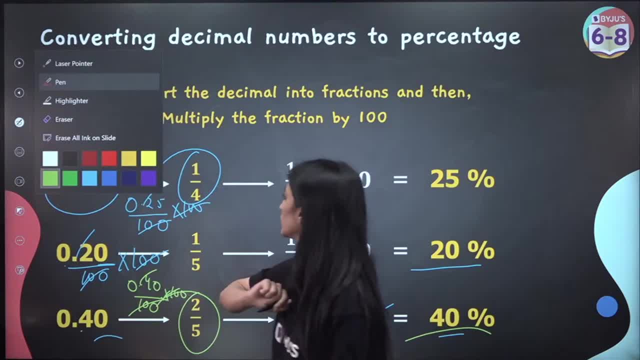 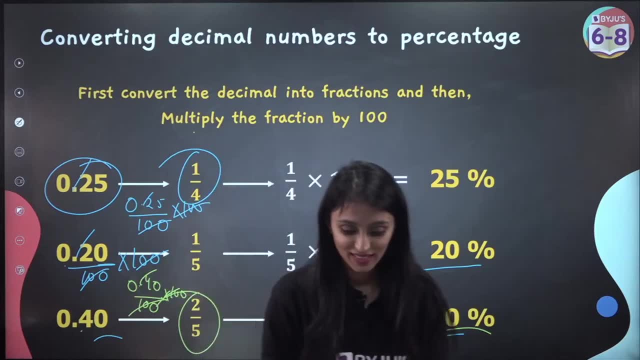 I can use green, yellow, red, blue, yes, white one. the bob lot of new students. yes, come on, fatafatse new students, pehle subscribe the channel screen not visible. kyun hi screen visible. 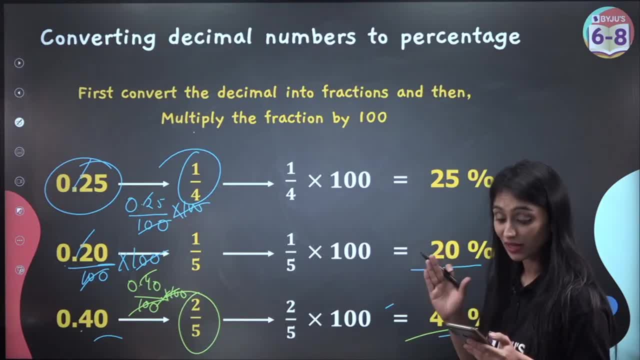 I can see here sab theek se visible hai. so, Naakshi, yes, we have that slide, don't worry, we will discuss it here. I showed you yehi colours hai aur koi colours nahi hai. bahut easy hai, simple. come on everyone, if you are enjoying the session, if you feel session. 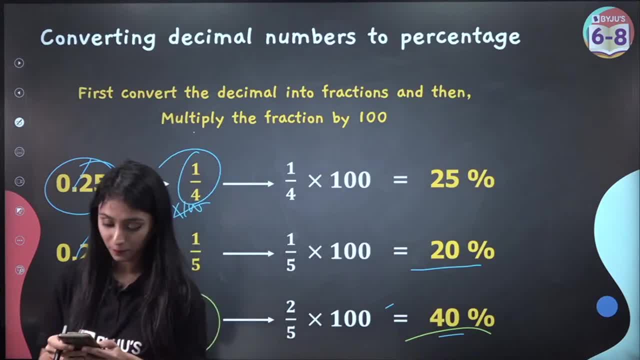 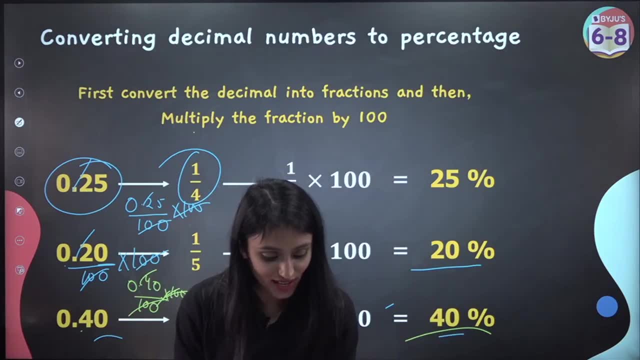 asamjh aara hai, whatever ma'am is explaining. come on, fatafatse, like 200 likes in this session. yes, Aastha Jhita, new student. yes, Aastha Jhita, please subscribe the channel. beta Bhagya, Adaroja, Deva Shree- a lot of people. what if there is? what if there is? 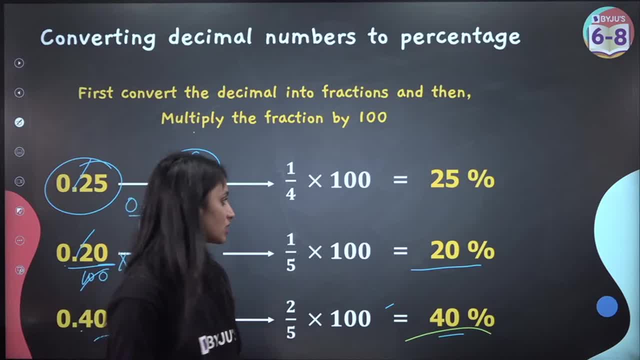 a lot of people. what if there is a lot of people? what if there is a lot of people? ok, Deva Shree is asking: Dev Shree, what if there is one digit after the decimal? koi number le lete hain right, one digit after the decimal ma'am 1.5, hai one digit hai. 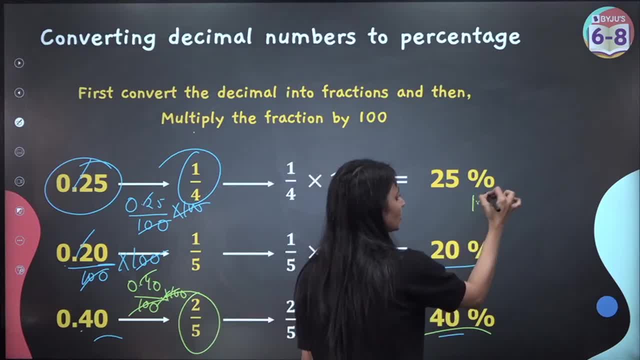 isse aap convert karo decimal mein what I will do as I said. let's remove the decimal. there is one digit, so I will write 10 in the denominator fraction. ban gaya simply multiply with 100,. cancel karo zero. kitna aagya 15 times 10,, 150% clear Dev Shree. 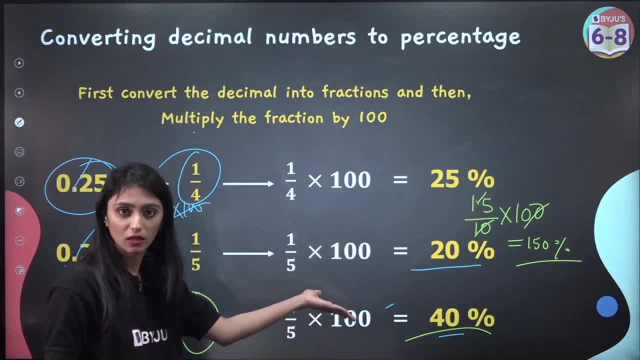 I hope it's clear now. I think it's better for others also because samajh aagya, I think it's better for others also because samajh aagya, I think it's better for others also because samajh aagya, I think it's better for others also because 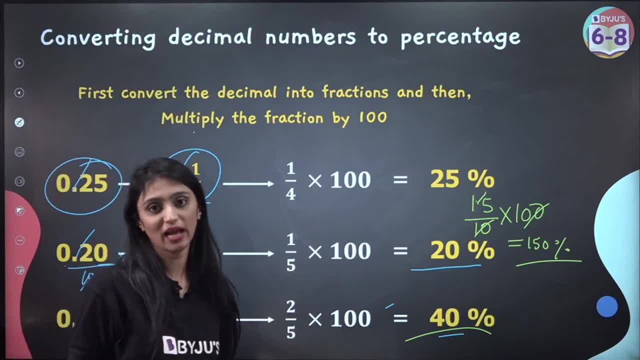 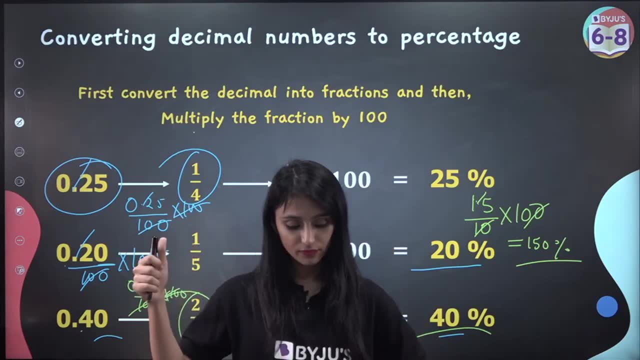 agar ek digit hai apon mein 10, teen digits hai apon mein 1000, 100 se, toh you will have to multiply anyways every time. yes, Mohammad Shafiullah, clear everyone. yeah, just some. 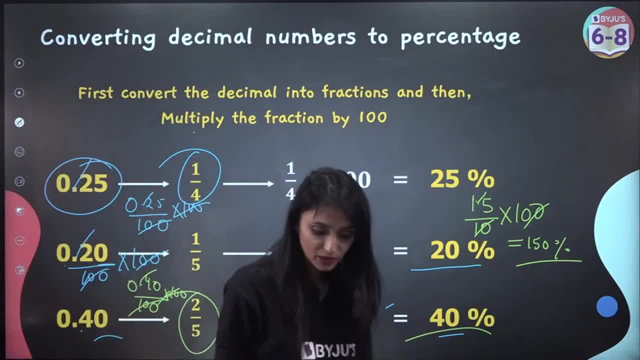 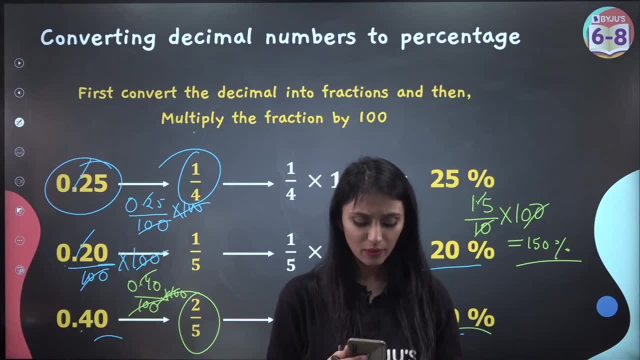 are saying: I don't know why is this happening. some are saying red, some are saying green, pink, pink, toh kena mere pass hai, hi, nahi hi Prachi. yes, Neetu Singh, all the new students. please, Bob the Bob, your name is Sonia. please subscribe the channel and like the. 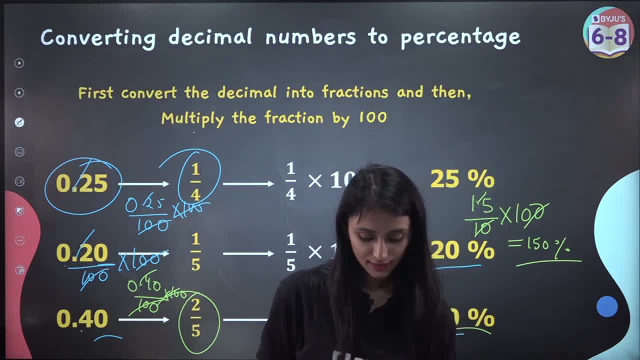 session also. agar aapko lagta hai useful hai session, please do that. please subscribe. subscribe to the channel and like the session also. agar aapko lagta hai useful hai session, please subscribe to the channel and like the session also, agar aapko lagta hai use. 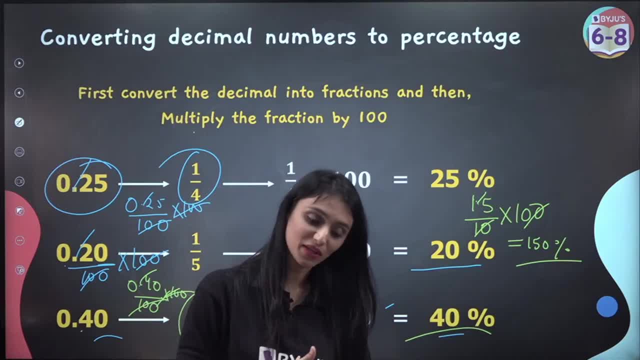 red right, Amritanch, woh bhi kar sakte hain directly. yes, we can do that directly. you can multiply by 100, decimal ko bhi. toh bhi aapka answer, aa chayega. 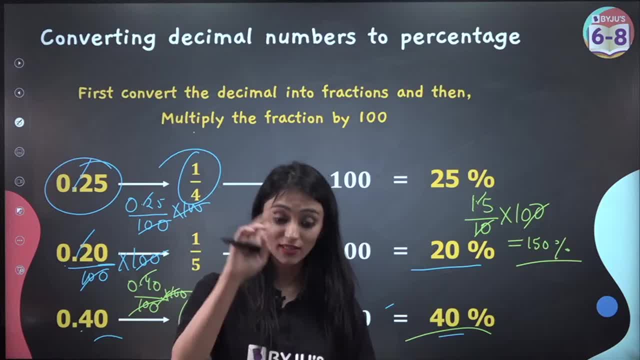 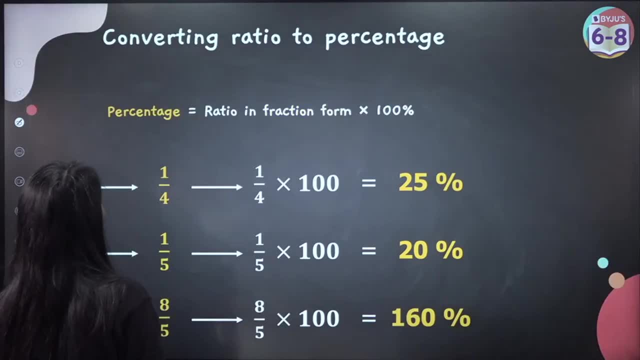 Mamta Sharma. hi Palak, bana Palak in another session. Abhi iss session ke baare mein. Chalye, let's move ahead by Aisana Goodra. Chalye, let's move ahead. Converting ratio to percentage. 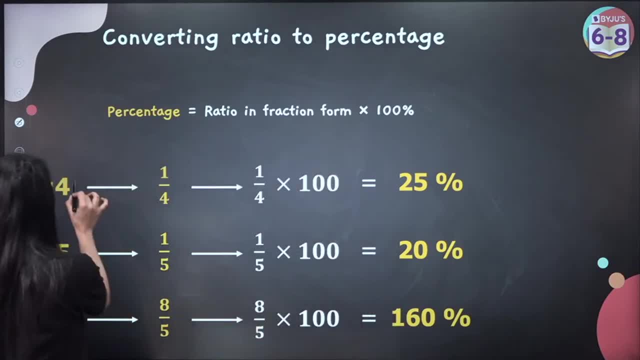 Ab ratio to percentage ko kesa karenge F Hatta fatse dekhte hain. we have 1 is to 4, ab mein kya karu iss 1 is to 4 ka? I don't think red would be win. 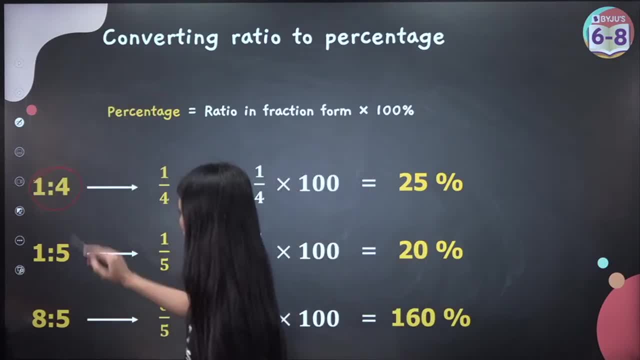 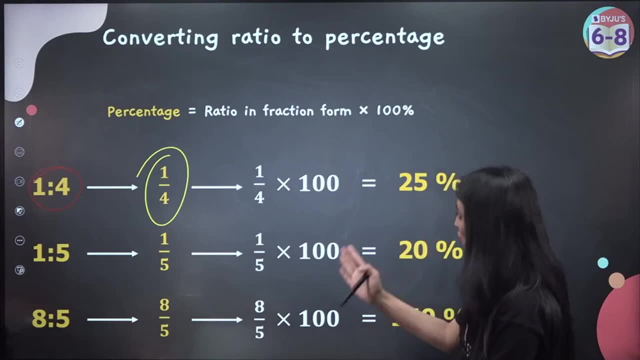 visible here clearly. Okay, what to do with 1 is to 4? First, write it in fraction. you can't do it directly. now Write it in fraction: 1 by 4, now you know the process. Now you know how to convert it. multiply by 100, you get 25%. Let's suppose 1 is to 5 is given. 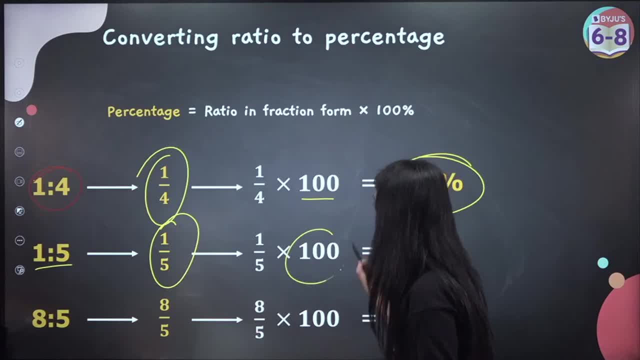 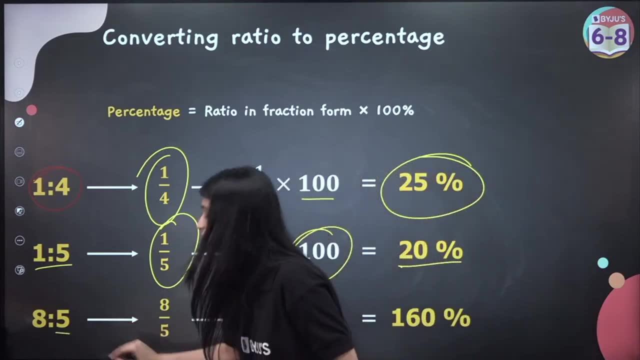 so I'll write 1 by 5,. first I converted it in fraction, then I'll multiply it with 100, same process, 20%. Whatever the ratio is, first convert into fractions. 8 is to 5, 8. 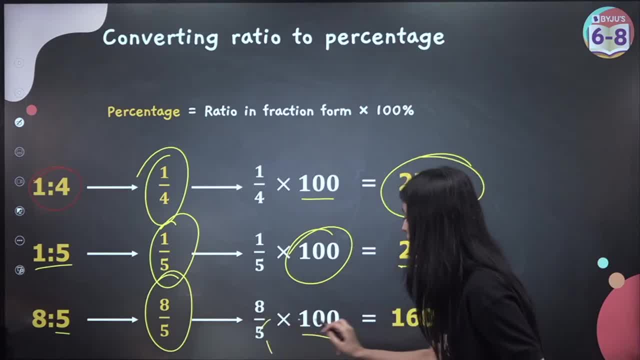 by 5, same process: multiply by 100, 5 ones are 5, twos are, you get 20,, 8 times 20,, 160%. Any doubts? Bitta pink colour hai hi nahi isme. Any doubts? or this is clear, Come on. 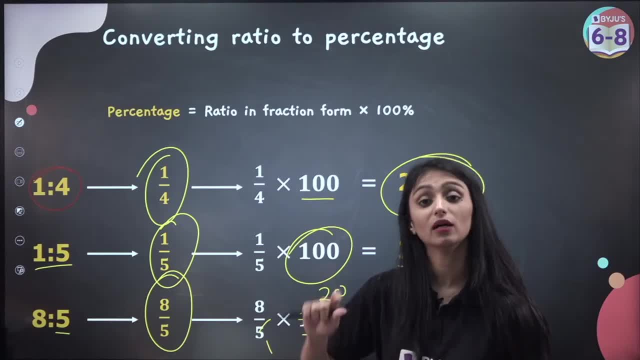 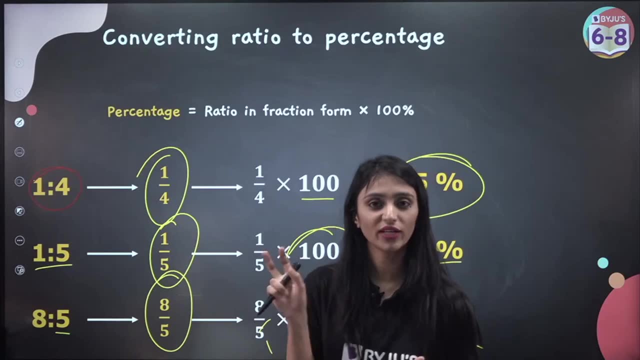 chaldi, se batao Kyunki jyoti 100, complete whole maana jaata hai, just like 1.. For me favourite colour there is no. okay, I'll tell you one thing: koi favourite, favourite mera at such nahi hota hai kisi bhi cheez mein. 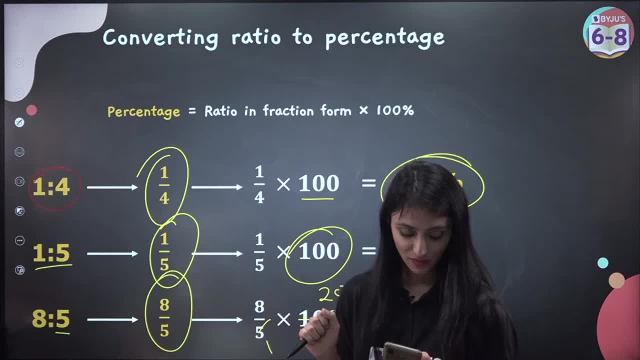 Okay, I'll tell you one thing: koi favourite, favourite, mera at such nahi hota hai. kisi bhi cheez mein: Yes, 3 by 1 ka 3 by 4 nahi hoga, 3 by 1,. kaha likha hai, bitta: 3 by 1 toh. 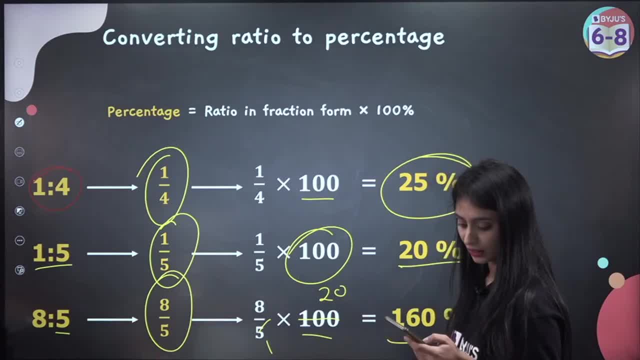 kahi hai, hi nahi, Mona bitta 3 by 1. toh kahi hai, hi nahi? Yes, jimko doubt hai. please aap post kariye bitta chat mein jo bhi doubt hai. Yes, Adi, but regularly classes ke liya. 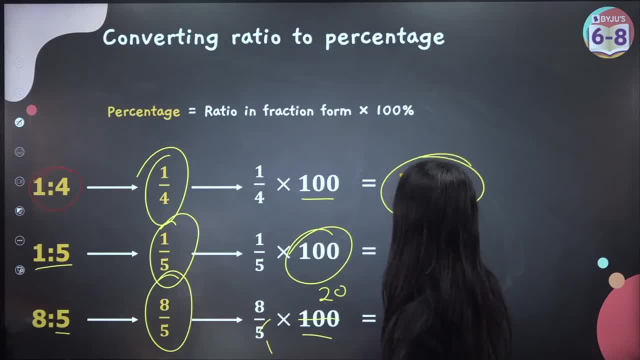 aogay, toh bitta maamko aise hi yaad rahega. Clear hai ratio to percentage. hum kaise jaate hai. Let's move ahead to the next topic: percentage change. Ye bohat baar aad hai. 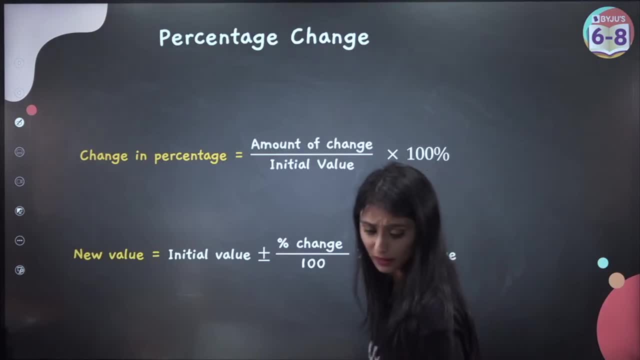 what aata hai word problems, mein Percentage change, Aur bohat baar bachche hi seez ko samajhi nahi paate hain. Dekhiye Darsh office bitta. jisko bhi doubt hai, aap chat mein post karo. 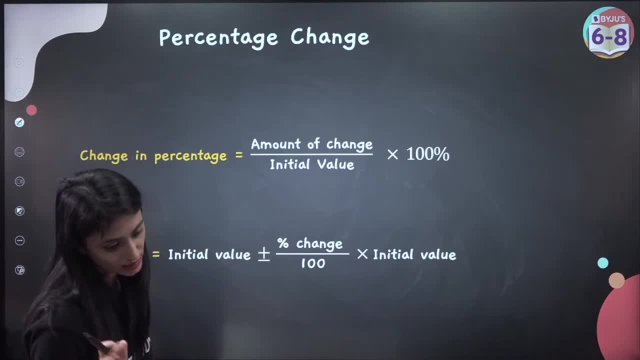 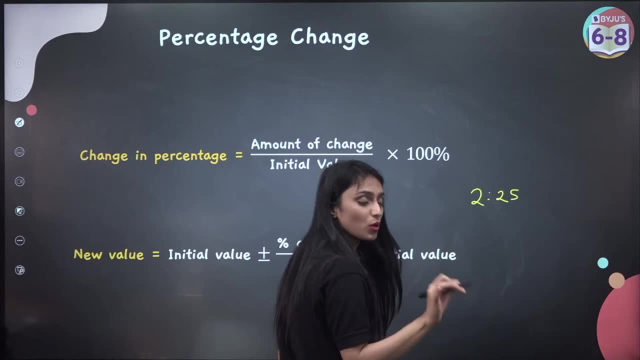 Okay, once I see that, I'll reply. Acha ek question hai kisi ka the bob maam, agar 2 is to 25 ho, toh maam, agar yeh diya ho, toh aap kyaise convert karenge. Same process. 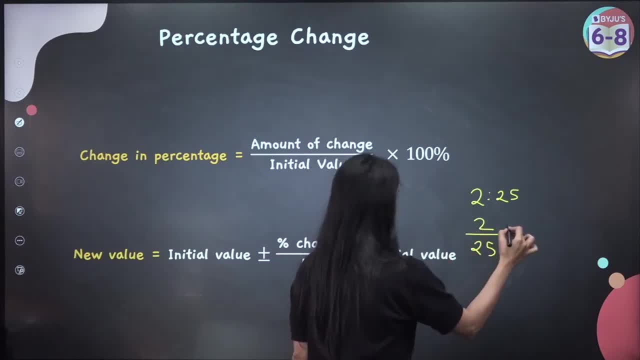 process. yahi hai isko pehle fraction mein likha. likha now you multiply this by 100, right, simple. 25 times 1,, 25 times 4, 4 twos are kya hota hai? 8, so this is 8,, so this. 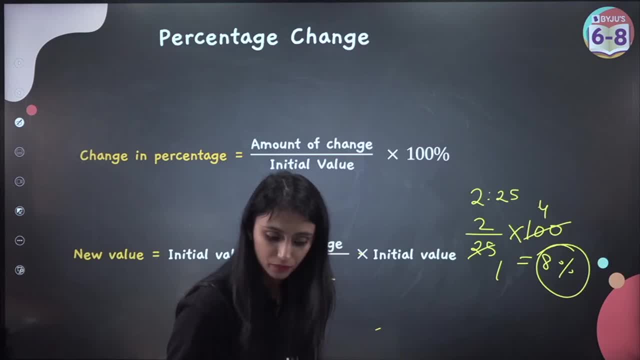 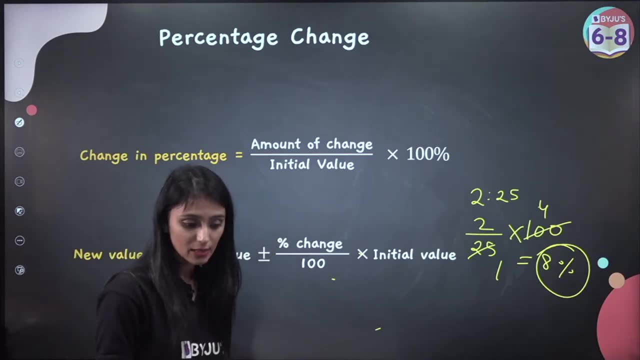 is 8%. now Clear the bob. yes, I hope this is clear, koi doubt toh nahi hai. aap Tabbhi theek hai, sabko clear hai. No directly aap ratios ko beta 100 se ratio ko directly. 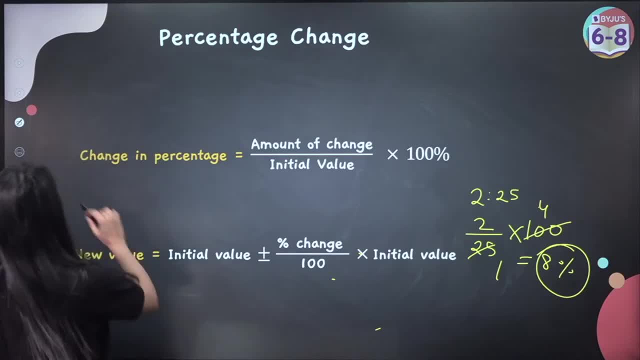 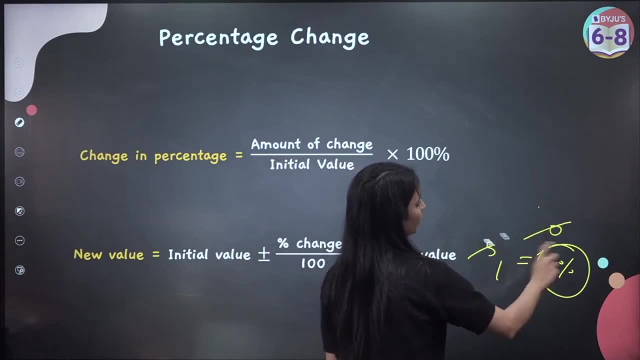 multiply nahi kar sakte hai. malash ka aapko pehle fraction mein convert karna hi padega, you will have to convert into fractions first. you cannot directly multiply a ratio with the with 100, you can't do that right. So you have to convert into fractions first. you cannot directly multiply a ratio with the with 100, you can't do that right. So you have to convert into fractions first. you cannot directly multiply a ratio with the with 100,. you cannot directly multiply a ratio with. 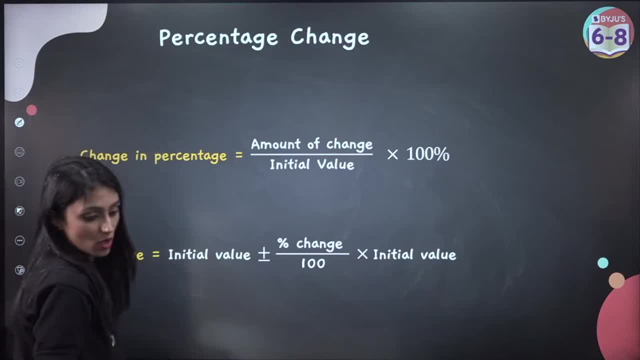 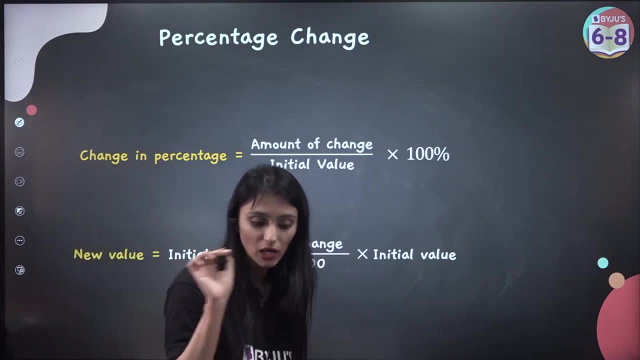 a 100, you cannot directly multiply a ratio with a 100, you cannot directly multiply a ratio with a 100,. ok, Klair hai, Chaliye aagechalte hai. ok, let's move ahead. yes, So stuti, 1 is to 2, is to 3, is to 4,. 1 upon-me sabkha total, lugge aap sabkha total. 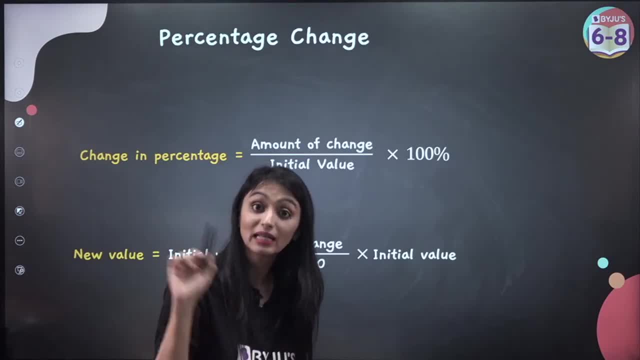 that's going to be 3 plus 4, 7 plus 2,, 9 upon 10,, 1 by 10 into 100,. similarly, 2 by 10 into 100, 3 by 10 into 100, that's how you will find this out. yes, Panna laal jiya. 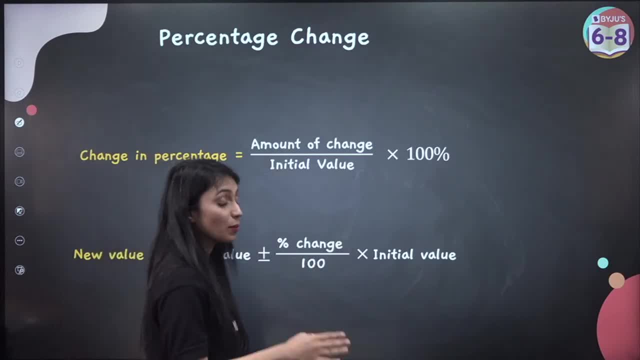 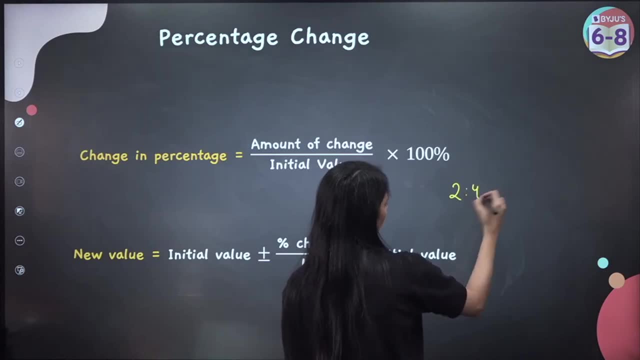 kar gave ir right. kya nahi samajh aaya beta cabatever ratio diyaa vyaa hai usse convert. Let's suppose you are given this. let's say 2 is to 4, you have to convert this into. 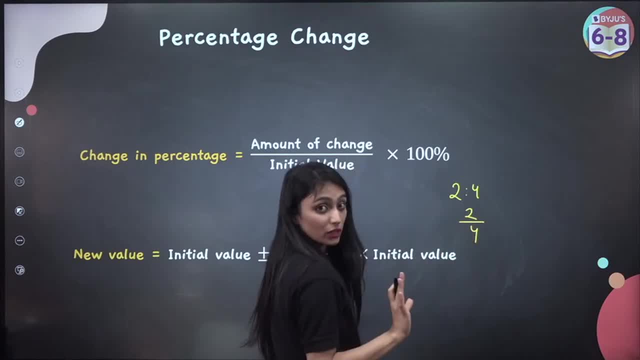 fraction. so first in fraction, I mean in percentage. you will write this in fraction after fraction. how do you go into percentage? Let's do it into 100, simple: 4 ones are 4, twos are 8, what is this? 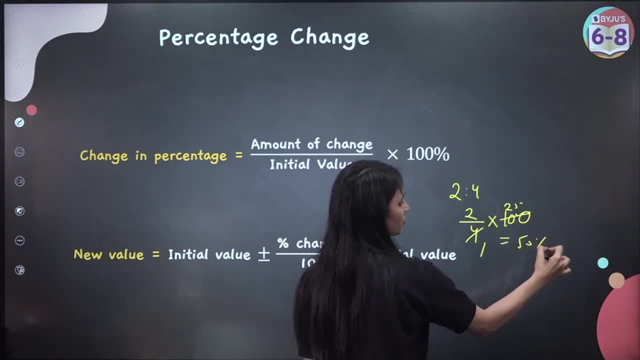 20,, 4, fives are 20,, 25, twos are 50, percent is made. So what you have to do? First you have to go into fraction with ratio, and from fraction only you have to go into percentage simple. 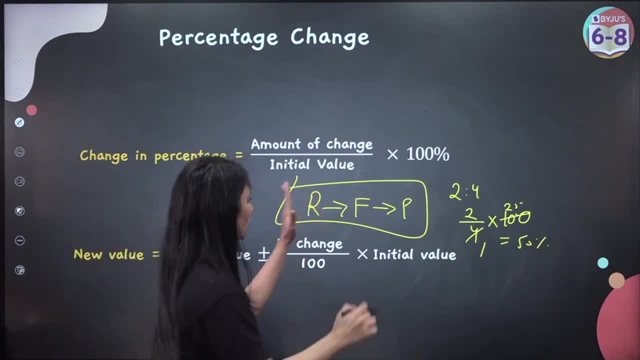 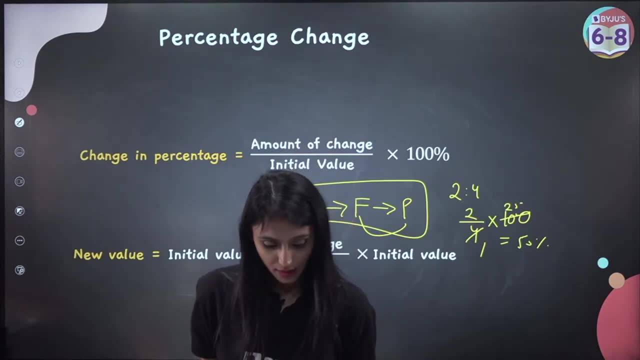 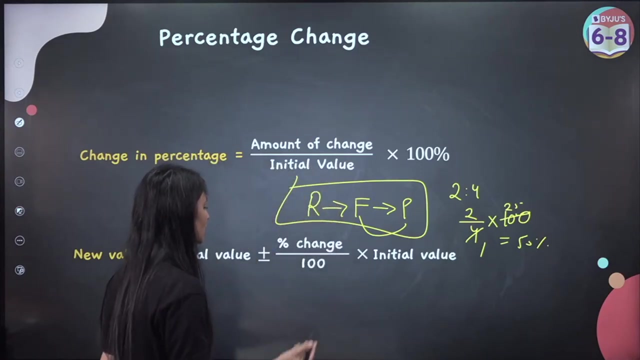 R F P, keep in mind R F P, and if there is no ratio, then only F P. it is simple: nothing. R F P. yes, Any doubts? Or this is clear, Yes, yes, when you are talking about the percentage of your marks, let's suppose in your math. 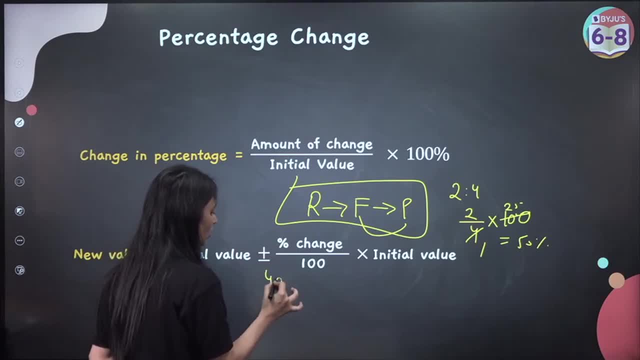 let's take an example. let's suppose you have 40 marks in your math and the total of all subjects is 20.. The total, whatever is the total mark means it is of 100 marks. and suppose you have 5 subjects- English, Hindi, Math, Science, SST- the total of all of them is 500, there is a 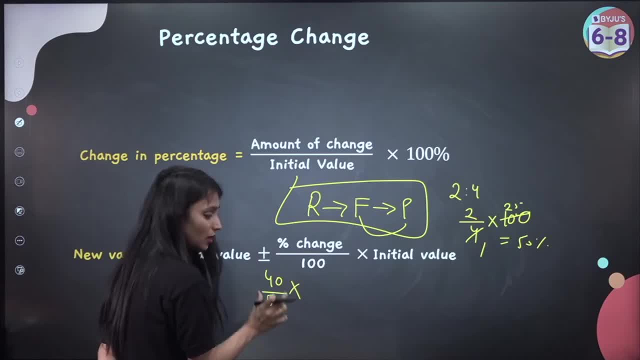 paper of 100 marks. Now, if you take out the percentage of math, then what will you do? Total below, above the marks of math into 100. Calculate it, you will get the percentage of math right. So 0 is cancelled. 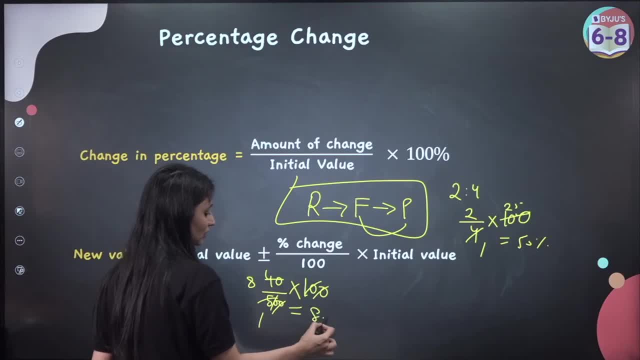 This is 5 ones, 5 eights. Oh, oh oh. such dirty marks, such dirty marks. 8 percent marks. right, This is my fail, this is a state beyond fail. Yeah, Is this clear? Is it clear to all? 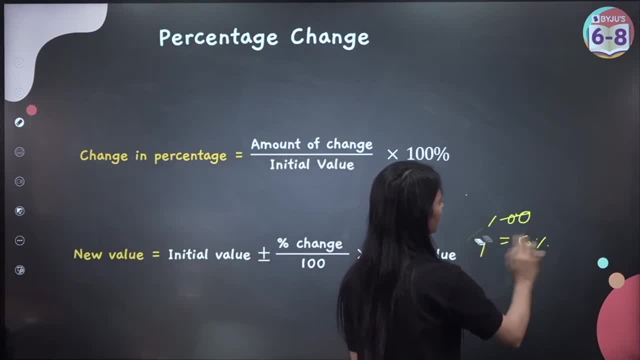 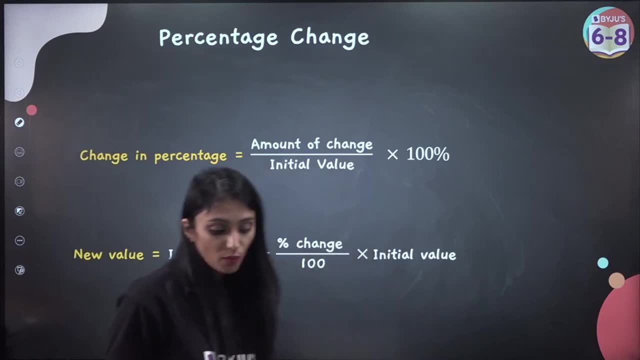 How to convert RFP. How to convert? You will go to the percentage only with fraction. you will not do it directly. Yeah, Yes, Nithila Napoleon, I can see a lot of new students over here. The new students. please subscribe because you join late session. 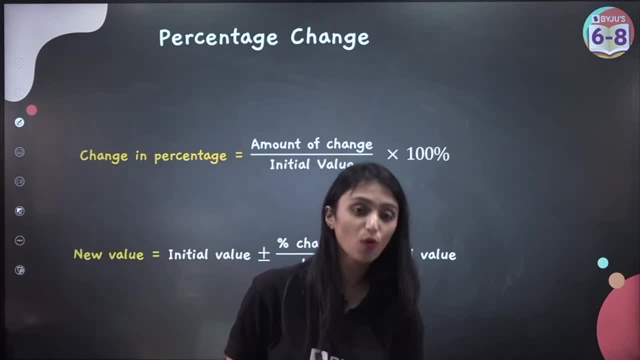 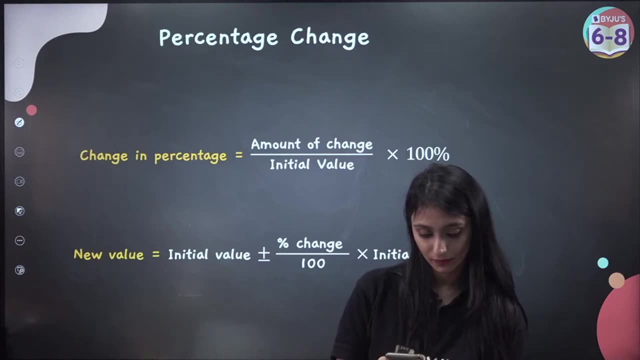 So what happens is that you miss out on a lot of things. then it becomes difficult for you also to understand, because all the things are linked right. Yes, Malishka, Pooja Yadav, Pooja Yadav, Put it on charging beta. there is no other option. 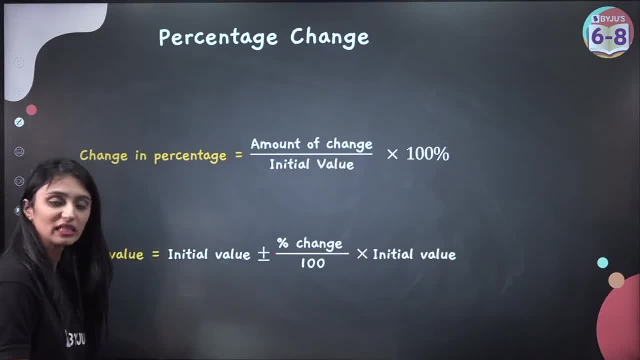 Come on, let's move ahead. Change in percentage. If you have to take out the percentage change, then what do you take out? Let's suppose. let's suppose like in your first term, the marks came in math. let's suppose. 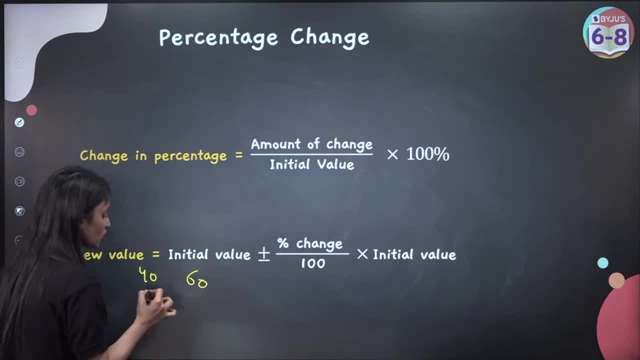 40. In the second term yours came 60. So how much change has happened? Change of 20 marks has happened. right, The change that has happened. we will write the amount of change above The initial value. the initial value means this: 40,. we will write it down. 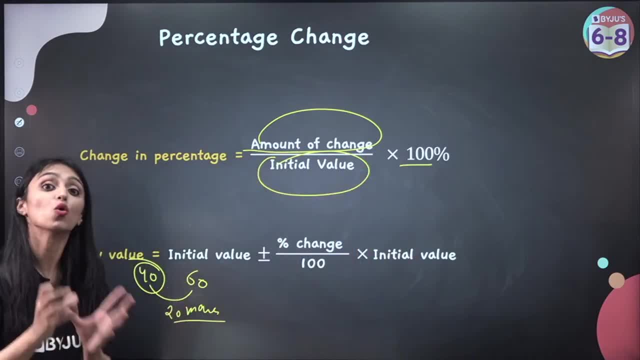 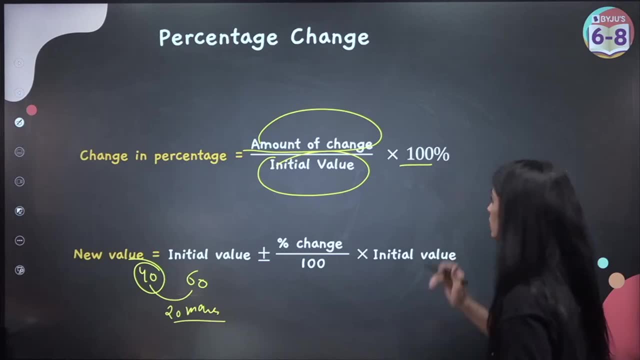 In 200%, you will get how much change has actually happened Genuinely, how much percentage change has happened right. To understand this better, let's suppose in the first year, in the first year, the washing machines which were sold- let's suppose that was, let's suppose that was 8.. 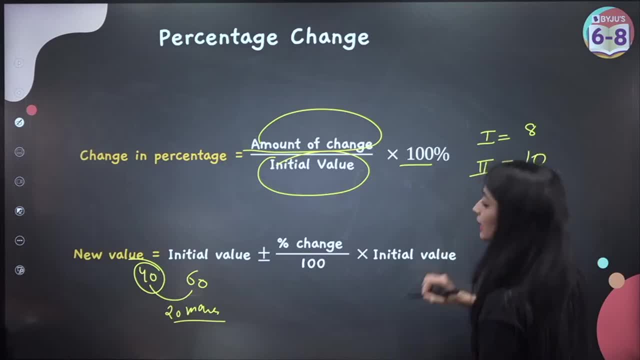 In the second year washing machines sold were 10.. So how much percentage? we know that washing machines have sold more, right, So we are getting benefit in this case, But how much increase has happened? How much amount of change has happened? 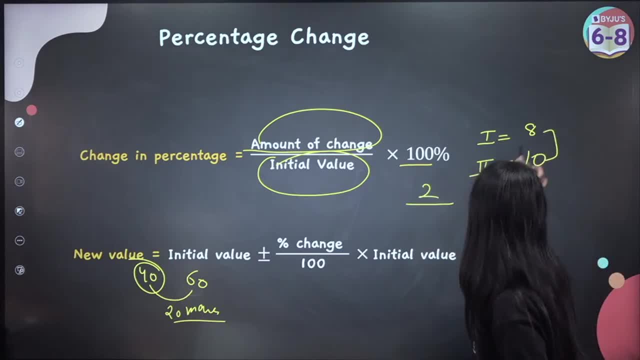 How much is the change Of 2 washing machines? So I will write the change above. I will write below: initial value means 8 in 200.. That's how you can calculate the percentage. So it has come 25%. 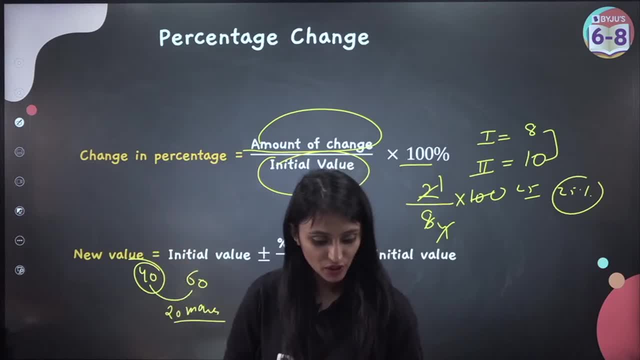 25% increase has happened in our sale. Yes, Prisha Rajak, thank you, Sonakshi. Yes, Prisha, same ways. Yes, Initial value means, means. what is the first one? You consider the previous one as initial. 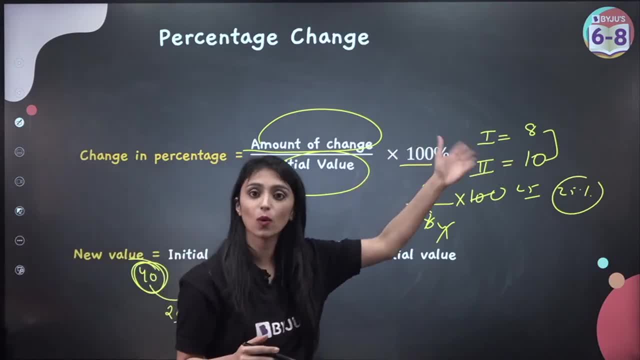 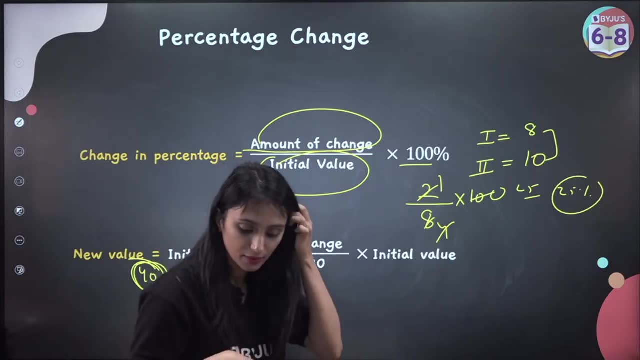 Like the marks which came in the first term, that is initial value. The sale which happened in the first year, that is initial value. Yes, Prisha, same ways, son. The method will remain same. Yes Shall we move ahead. 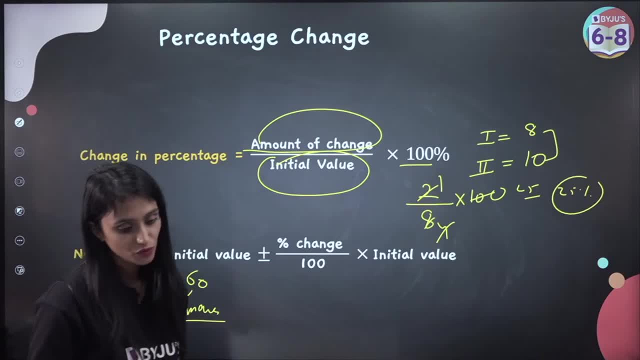 Yes, Which full video. Perimeter area will also come. Yes, Maisha, which full video. Alright, let's move ahead. New value: Now let's talk about whose New value. So what is new value? If you are talking about taking out new value, you have to take out new value. 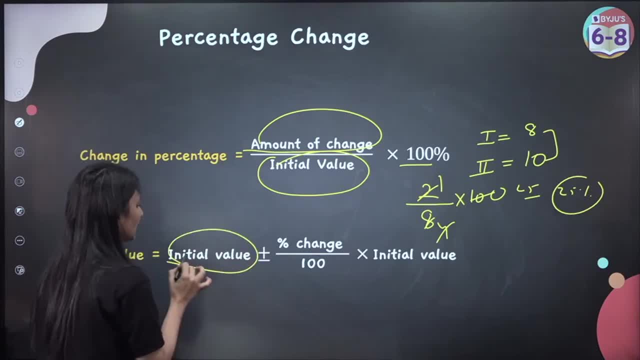 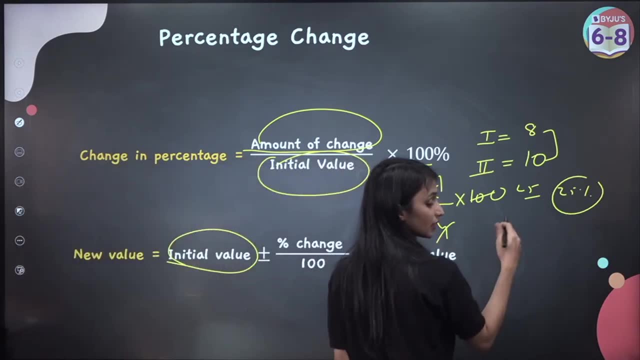 Okay, Now let's suppose whatever is the initial value, if you have to take out new value of any thing, right, Let's assume. let's consider a case: Cost of any object. cost of any object: in the first year it was 1000.. 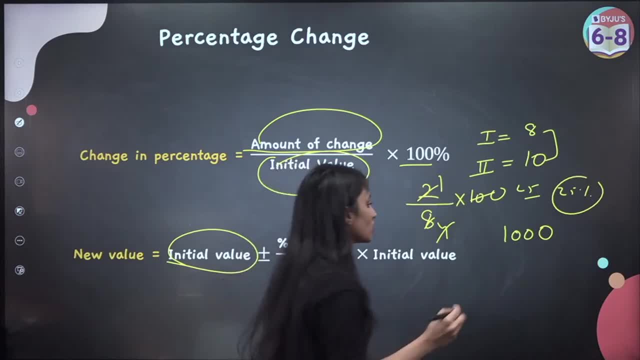 Right, Now. it has increased. it has increased. it has increased by 25%. Now this has increased by 25%, Right, Okay, Now it has increased by 25% in cost. So what is its new value? How will you find its new value? 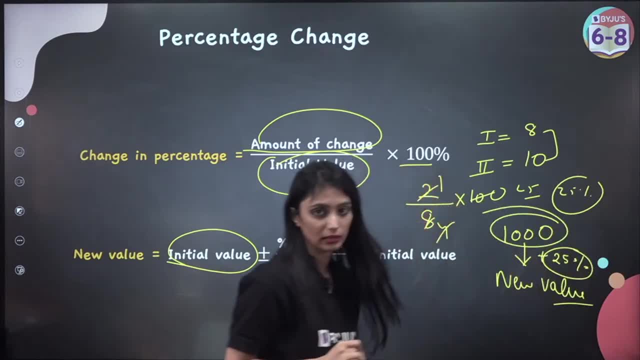 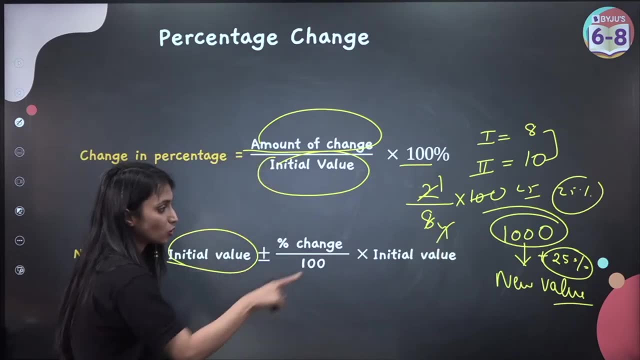 You will say, Ma'am, first let's take out 25% of this, Let's find out 25% of 1000.. First you will take out 25% of 1000, right? So how much percentage change is there? 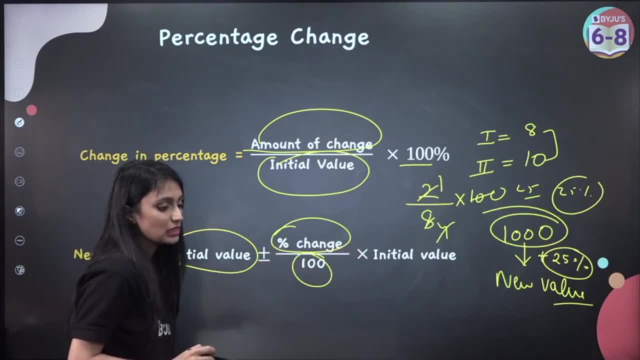 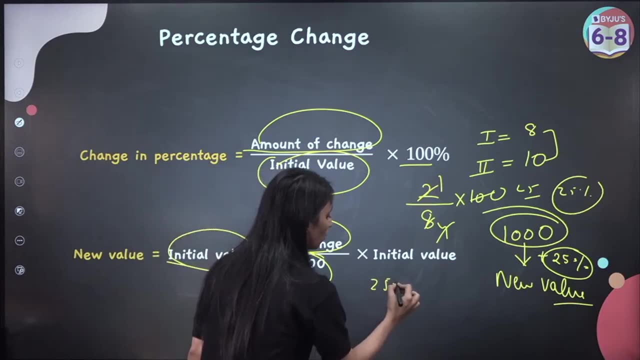 25% right Upon that 100.. See, whenever percentage symbol has to be removed, then we do 100 upon Right. If 25% has to be written normally in fraction, then what will you do? Just remove this percentage symbol and write upon 100.. 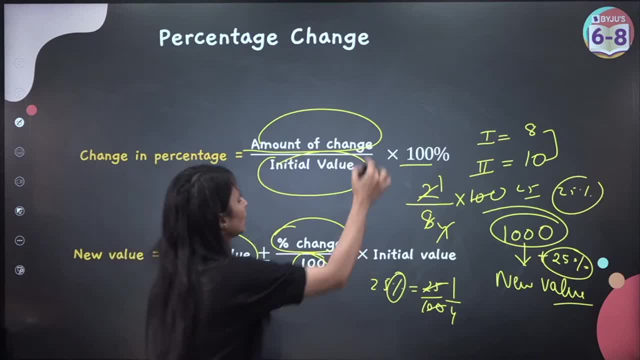 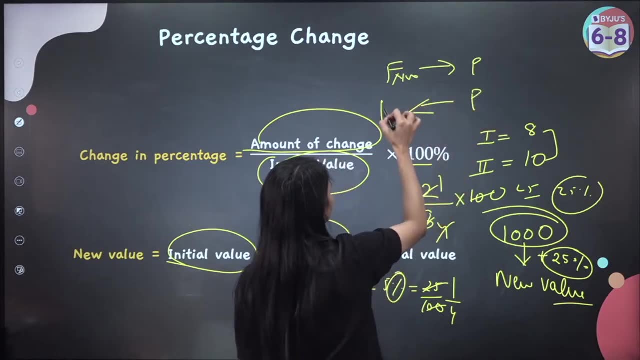 This becomes 1 by 4.. To go from fraction to percentage: From fraction, when you go in percentage, you multiply by 100.. To go from percentage to fraction, To go from percentage to fraction, what will you do? You will divide this by 100.. 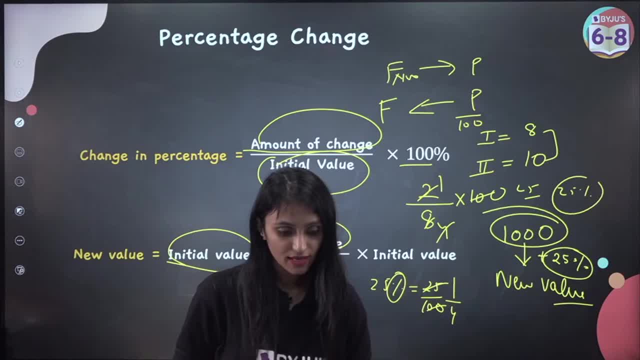 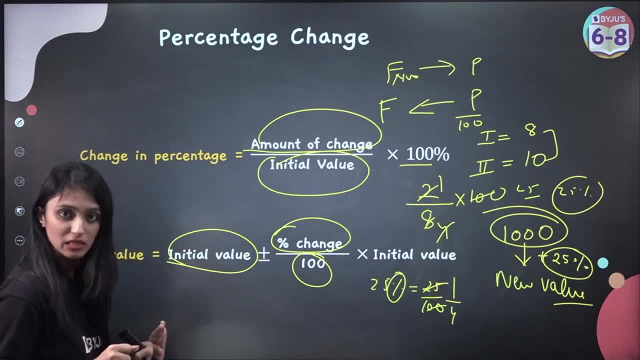 Opposite of it, Right? Yes, Yes, Rizwan, Is everyone clear? Yes, What we are doing here is how to take out percentage change first. In any thing, You have sold 8 washing machines in the first year. 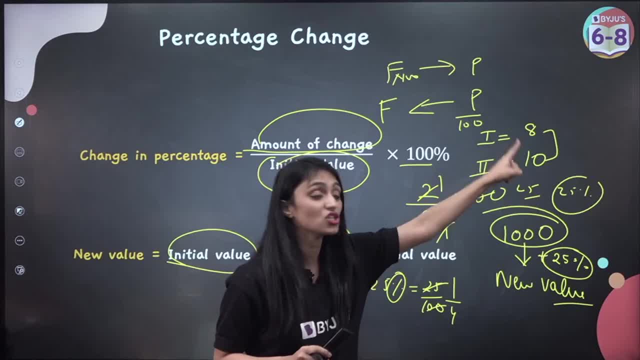 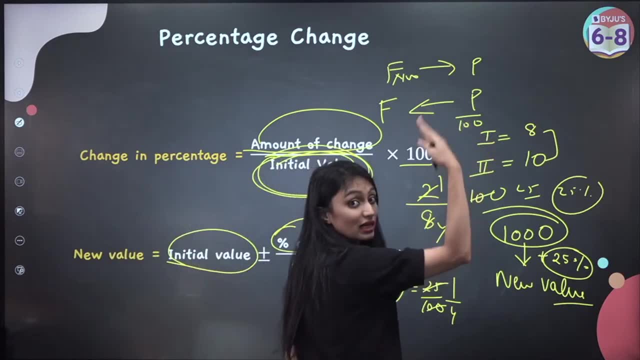 You have sold 10 washing machines in the second year, Right? So how much change has come in this 2 washing machines? This is change. So always put change above. Put initial value in upon. Initial value means what is in the first year. 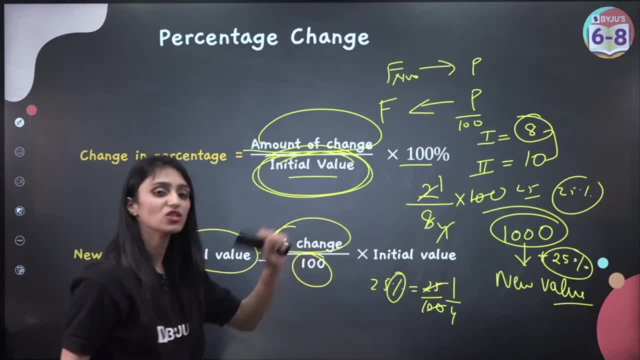 It remains initial Upon 8 into 100.. So percentage change has come. Let's take it out like this: This change can be increased or decreased, Right, And no change at all can be done, Right? Yes, everyone. Thank you, Arpita. 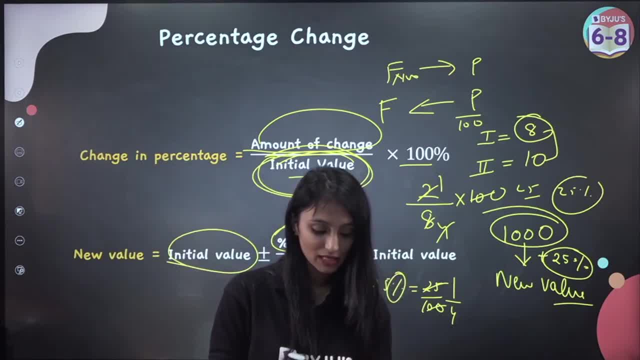 Please, everyone. If you are liking the session, please, please, please. It is fun. I am understanding everything, So please like the session too. And how do we take out new value, The percentage change that has come? first, put it in fraction. 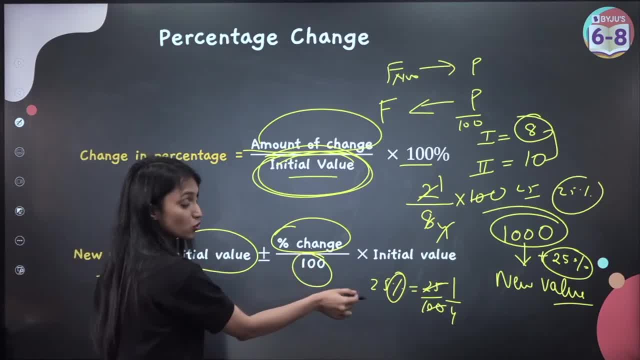 Upon 100.. Into initial value, As always. Right When it comes, add the initial value in it. Correct When it comes, add the initial value in it. How much is 25% of 1000? 250.? 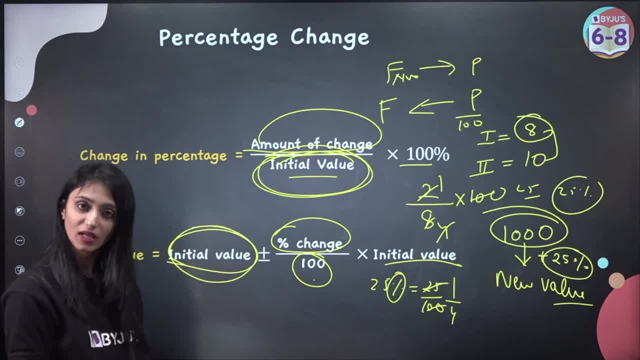 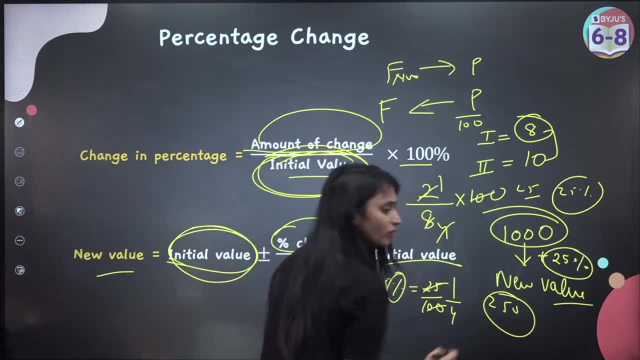 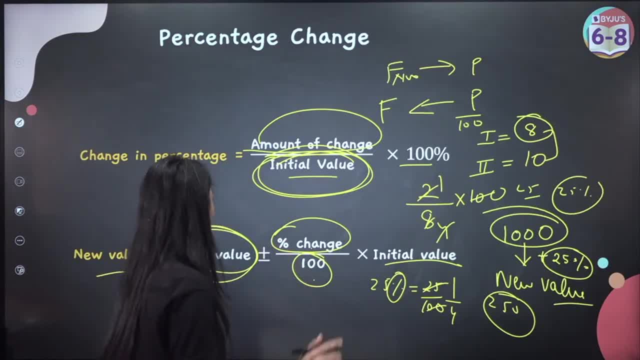 The percentage change has come. How much it has increased? It has increased by 250 rupees. So what will be the new value? What is the initial value? 1000.. Plus, how much has the change come? It has come in 250.. 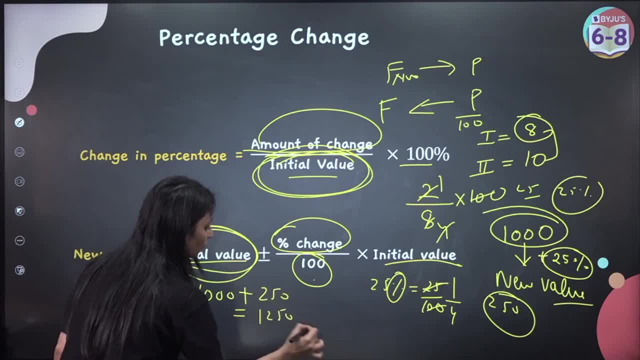 So this is going to be 1250.. Let's find it like this. This is one. the entire formula is given once. You don't need to write it once, Right, What you can do is first you find out the change. 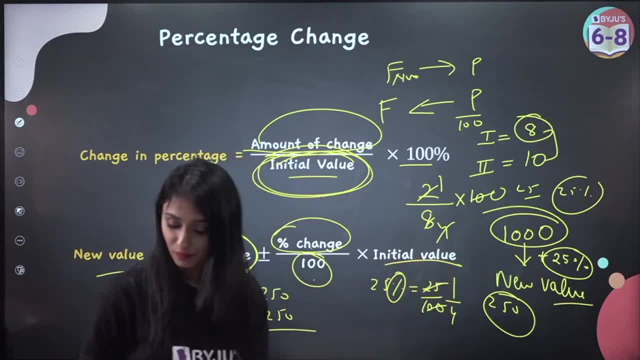 If anyone has not understood yet, then I will just break this. Don't look at this formula. Right, This percentage change will increase, Right? What you can do is first you find out the change, First you find out the change. 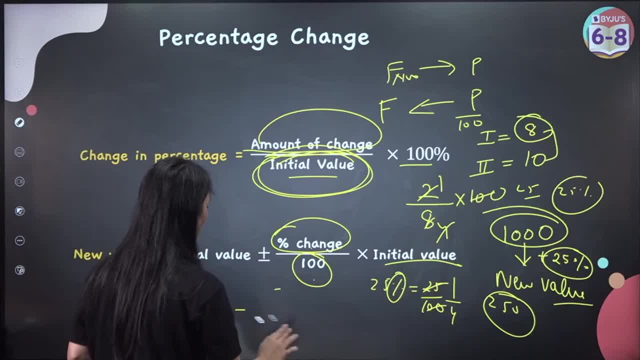 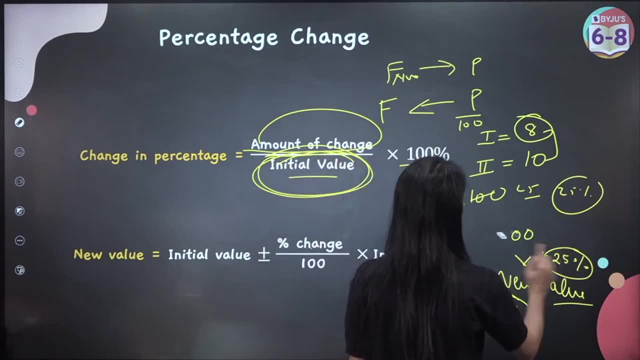 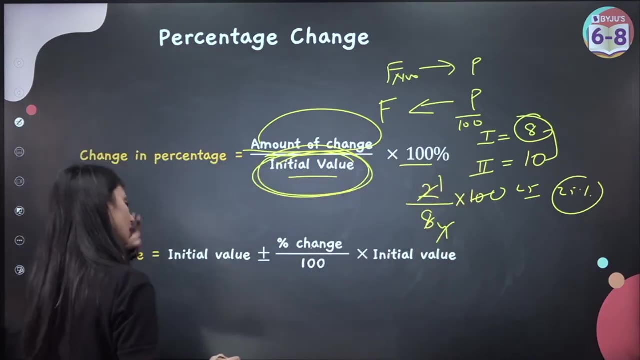 Who didn't understand yet. so I will just break this. Don't look at this formula Right. This percentage change can be increased or decreased. I will just show you. Let's suppose. let's suppose if we are talking about a mobile, the cost of a mobile is 20,000 this year. Now that cost increases. 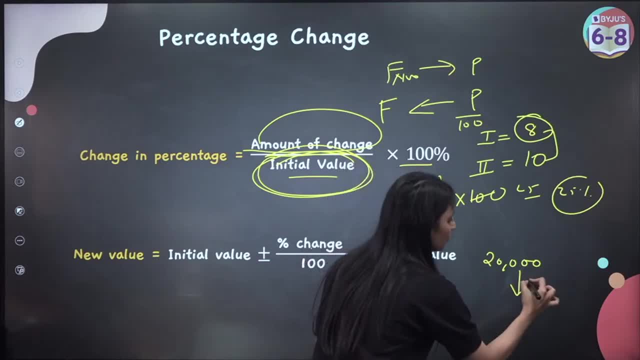 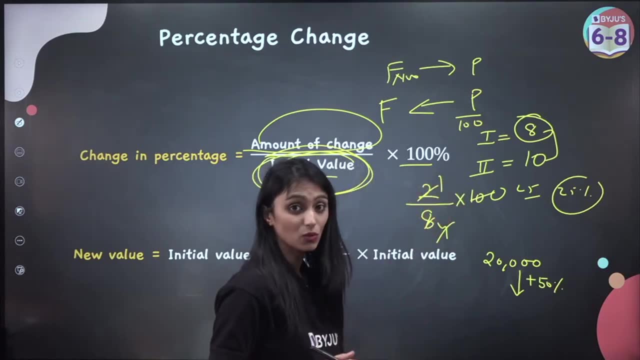 after some time. How much does it increase? Let's suppose it increases by. let's suppose it increases by 50%. What will be the new cost? First you take out how much has increased, First you take out the increase. So 50% of 20,000.. We are doing this, How much is the? 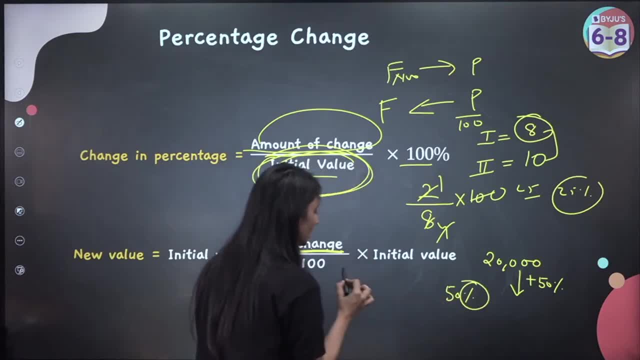 change Percentage, change 50%. As soon as we remove the percentage symbol. what do we write? We write 100.. Is it clear? First tell everyone. Is it clear? Quickly? Arushi, 10th class, it's on weekend, Don't worry. 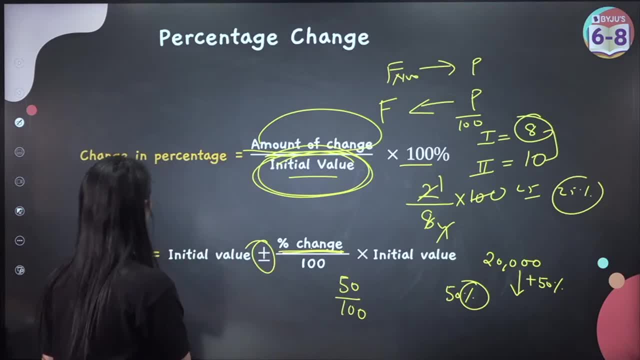 That plus sign, Son. we are showing this plus minus. You forget this formula. The formula is confusing you. We are showing plus minus. It is not necessary that the price increases every time. Sometimes the price drops too. So for that minus sign is also. 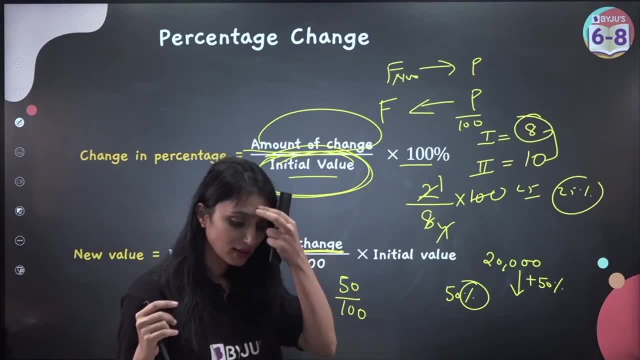 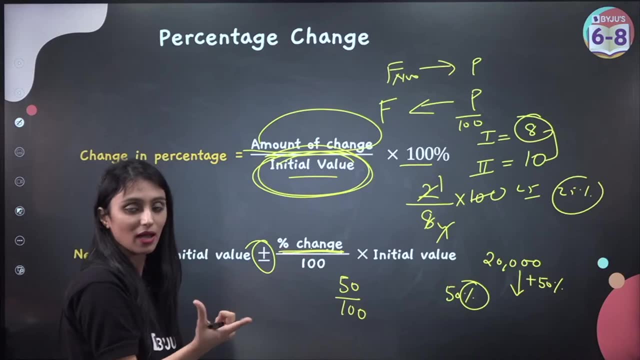 applied for decrease, One plus and one minus, That anything can happen, Right. So percentage symbol, because it cannot remain. This is 100,. this is a normal value. What is the percentage doing in between? You can calculate the same values only As soon as you remove the percentage. 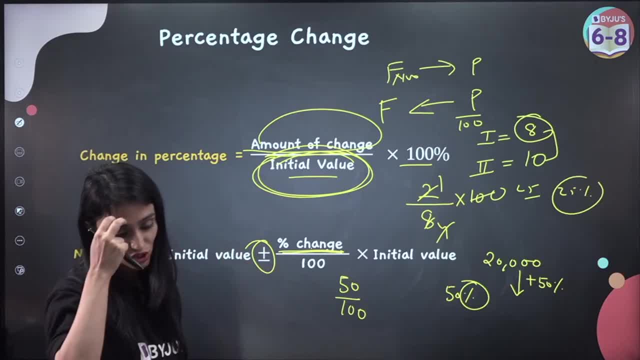 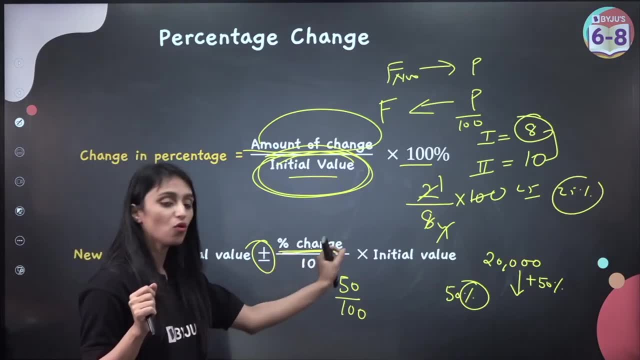 100 will come in the upon Yes, Yes, Srishti. I just saw it. I just saw it: Yes, Dhanya, Yes. So what we are doing here is: first we remove the percentage symbol. When you remove it, you write 100 in the denominator. 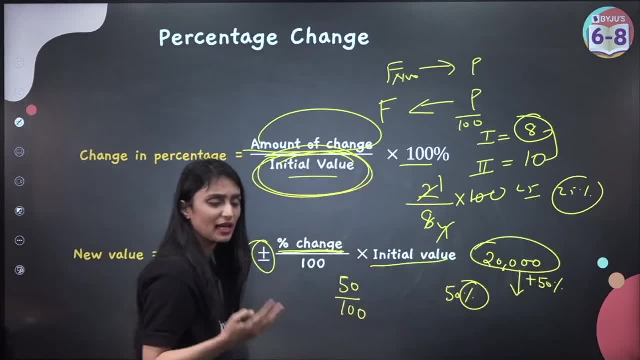 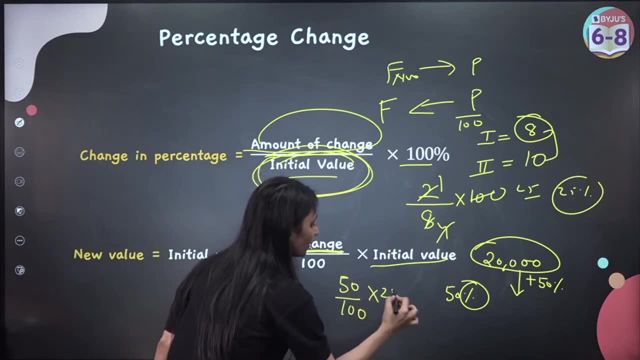 into initial value. What is the initial value? That's 20,000.. Anyways, ye 50% kis ka hai 20,000 ka hai, So we will calculate this on 20,000 only. So 50% of 20,000 is what That's. 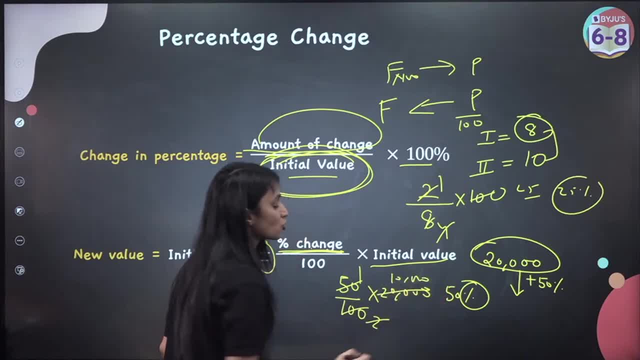 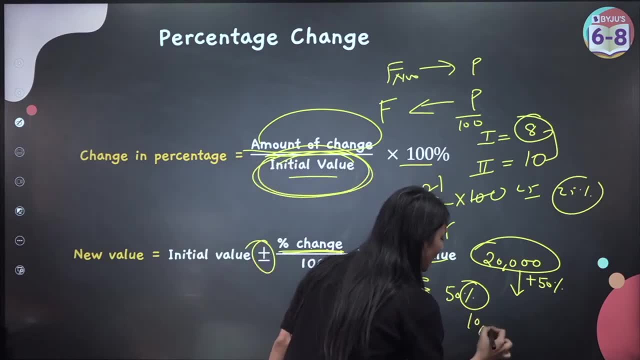 exactly half of it. Right, That's going to be 10,000.. So that means the value of this mobile phone has been increased by 10,000 rupees. Right Increased by 10,000 rupees. Right Increase kitna hua hai By 10,000 rupees. So what is the new value? New value. 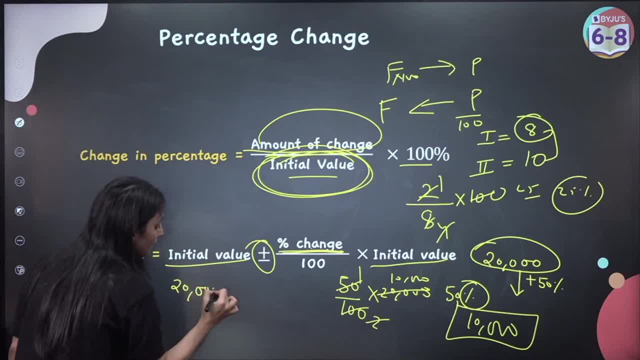 is going to be initial value, that is 20,000, plus the increased value, that is 10,000, that's going to be 30,000.. Ye symbol se confused: maton Plus minus means it can be plus it. 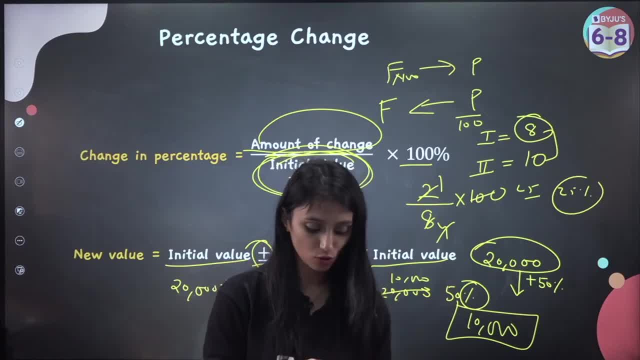 could be minus also, depending ki aapka ye increase ho raha hai, ye decrease ho raha hai. Any doubts or is this clear? Come on everyone. Yes, Namrata, I have explained again Kiran similar way: avishi and devishi: simply multiply by 100, you will get 57%. Yes, Malishka, 630,. 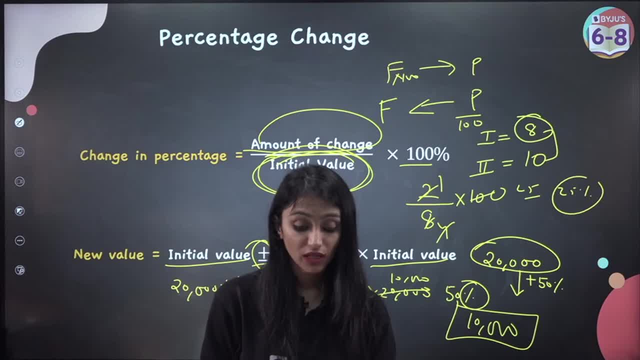 630 grams upon 3.5 kg. Kg mein nahi pehle hu se convert karo grams mein Right. Convert karo grams mein phir into 100 karna Aise, Because 100 as a whole liya jaata hai Srishti. 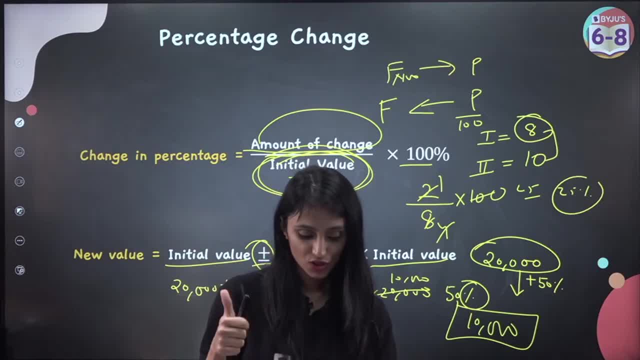 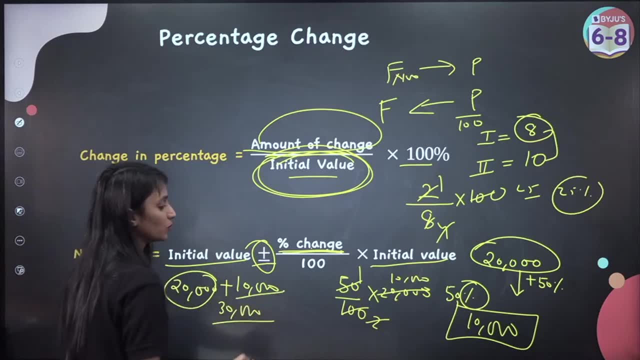 as a whole liya jaata hai amesha Understood. New value, All right, Acha Laksh, new value. kaise nikaalte hai Beta kisi bhi cheez ki purane value, mein new value, purane value, mein increased value, add karoge to ye aajayegi New value aise. 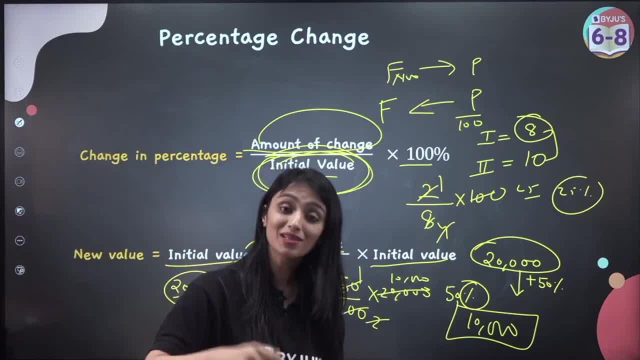 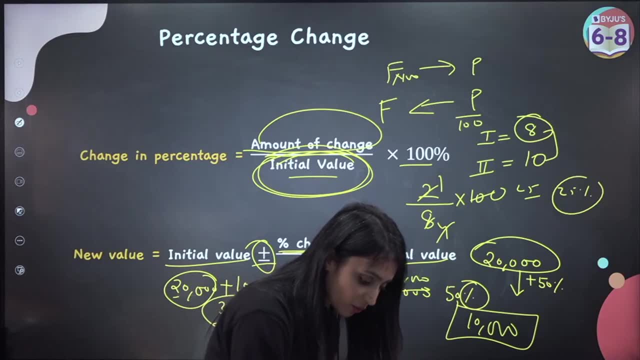 nikaalte hai Formula se confused maton, Don't look at the formula. Main aapko uska reason diya hai, why we are doing this. Laksh, abhi clear hai. Yes, come on, everyone Sab kuch. 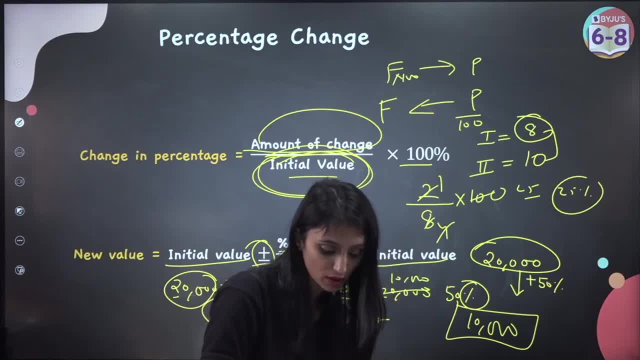 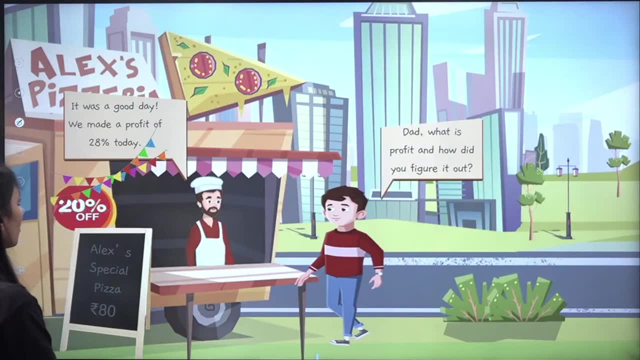 clear hai To thumbs up zo chat mein. Yes, understood, Chaliye, chaliye. Let's move ahead. Move into the next topic: profit and loss. Okay, Now father says it was a good day, because 20% discount diya and they had a profit of 28% ka profit bhi hua. Now Alex says that what? 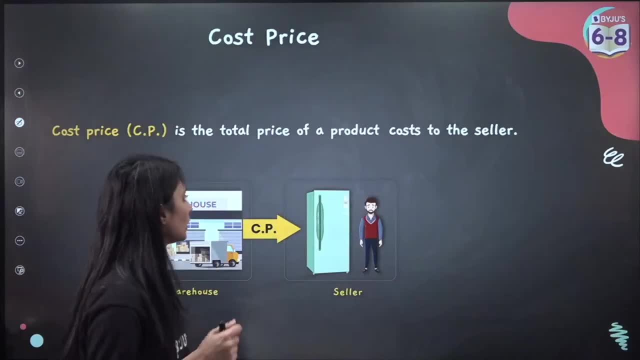 is profit. and how do you figure it out? Profit hota kya hai Aur nikaalte kaise hai? So first cheez, isme aati hai. cost price, That means CP, Cost price kya hota hai? It is the total. 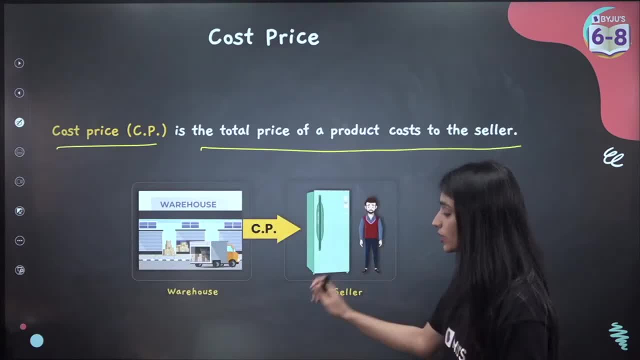 price of a product cost to the seller. Ek product ka jitna cost jo seller ko cost karega Aapne jaake. let's suppose aap shop pe gaye. you go to a shop and let's suppose you bought. 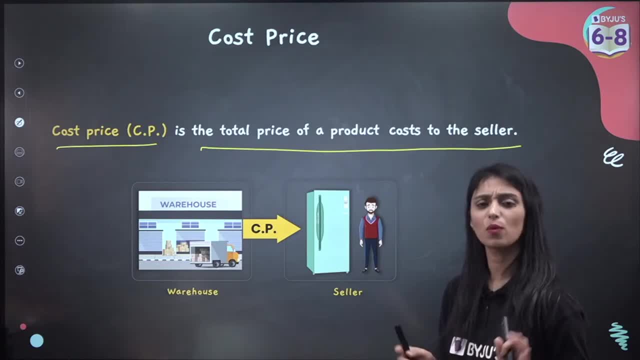 a mobile phone, right, You bought a mobile phone. let's suppose it was for 10,000 rupees, right? So for you that was what Let's suppose. abhi, yeh wala case nahi lete. Let's suppose 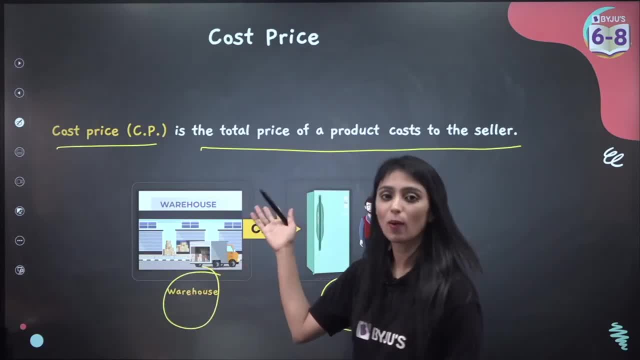 yeh seller hai, yeh ek warehouse pe gaye. yahaan se yunne ek mobile phone liya. Bohot saare liye hongi, but am ek ka case consider kar rahe hain To inko jo cost, let's suppose. 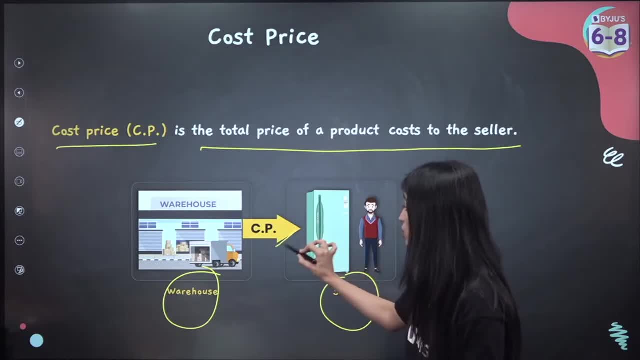 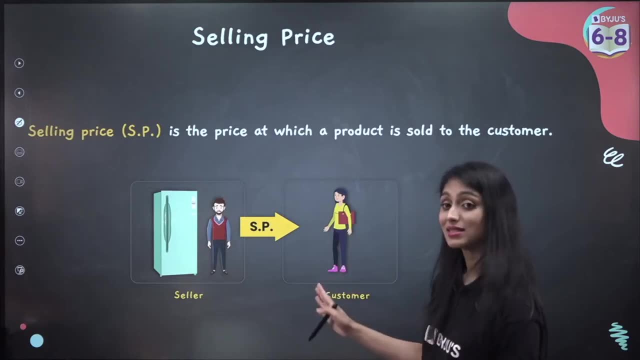 wo 10,000 ka tha. that 10,000 was nothing. that was the cost price for this product For this seller. Yes, Inke liye ho gaya yeh cost price. Now, abhi yeh seller ne kya kia. 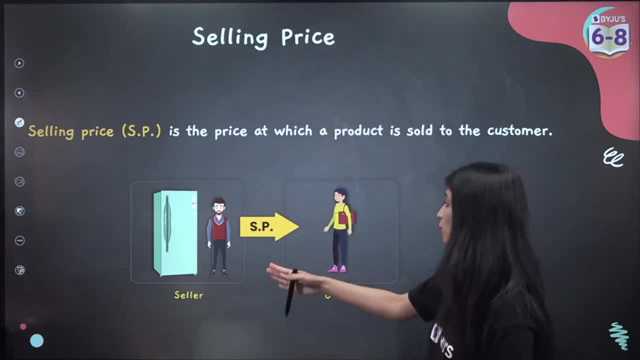 Inone aage. let's suppose yeh wo refrigerator tha, not a mobile phone. yeh aage kisi customer ko inone sell off kia To wo. kya banega customer ke liye? For him it was the selling price. 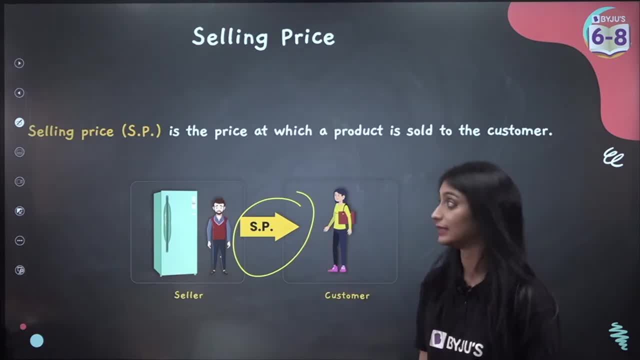 But customer ke liye wo ban gaya cost price because inone us price pe kharida hai. So the price at which a product is sold to the customers, for the seller, this is the selling price, because he is selling it. Yes, How do we take out profit and profit from a product? 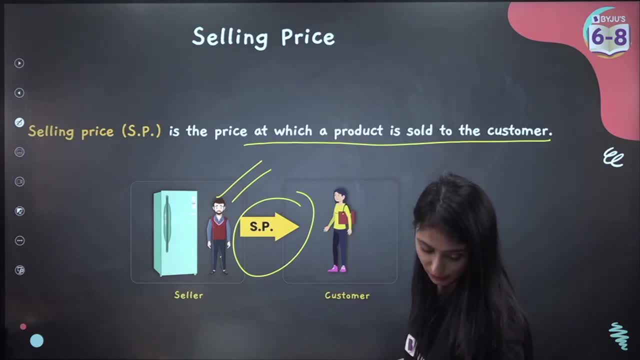 Abhi, abhi, abhi, abishi, abishi and devishi, we will do that. we will do that, don't worry. Okay, so cost price: whenever cost price is lesser than the selling price, jabdi less. 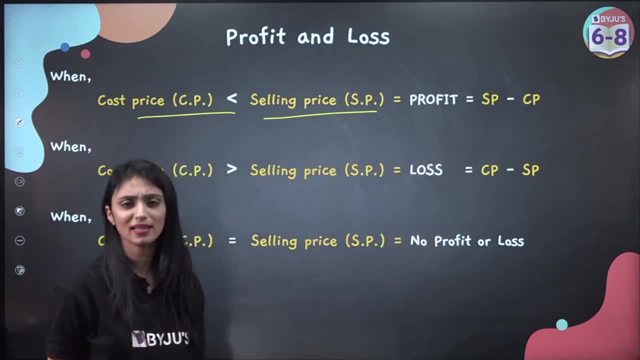 hoga. we say obviously, agar cost price selling price se less hai, right, Ek shopkeeper ne koi cheez 10,000 ki liye hai aur customer ko 8,000 ki aap sell off karne hain, it's going. 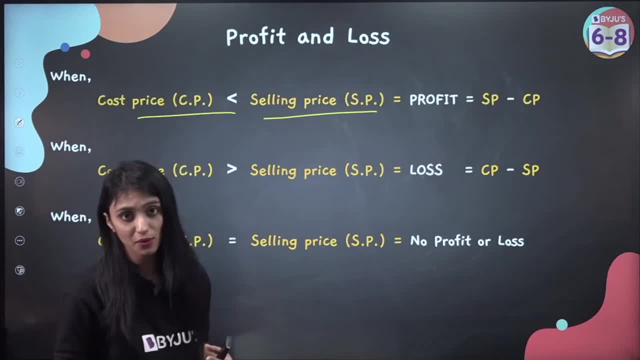 to be what? I'm sorry customer- ko aap 12,000 ki sell off karne hain. 10,000 ki cheez it's going to be a profit. so selling price minus cost price, But agar 10,000 ki cheez he is. 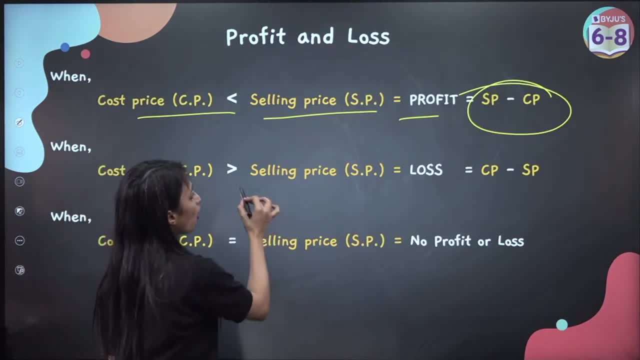 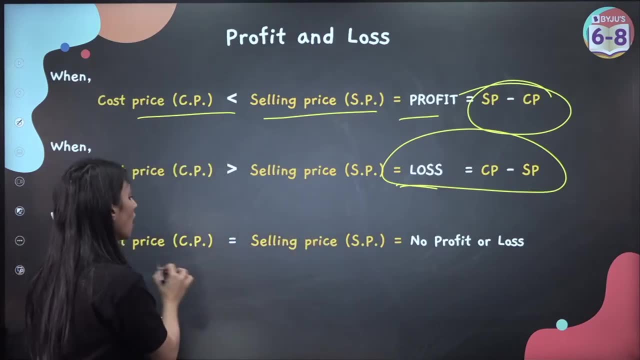 selling at 8,000, so that's going to be a loss, which is which is cost price minus selling price. Just remember this thing: yeh to normal scenario jo aap relate kar sakte ho. Aur agar dono hi equal ho jaye: 10,000 pe hi khareeda and 10,000 par hi he is selling. 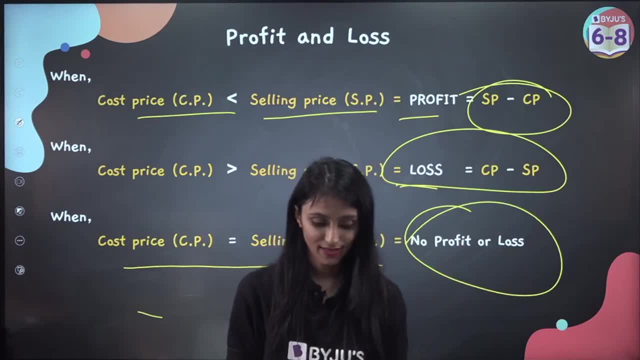 it. so, in that case, no profit, no loss. Yes, Yes, yes, yes, maane ajat, Okay, yeh to aap, aap paise mein discuss kar rahe hain: Gain or profit? same thing. yes, shagun, same thing. 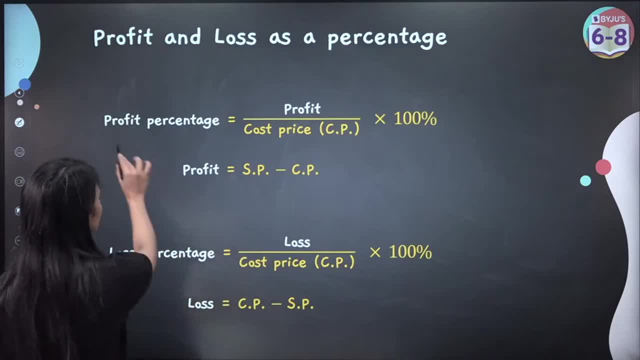 Chalye profit percentage kaise calculate karte hain? I tell you one thing: profit percentage ho or either it is loss percentage. We always calculate both of them on cost price. only cost price par hi calculate karna hai. So profit upon cost price into 100, percentage. 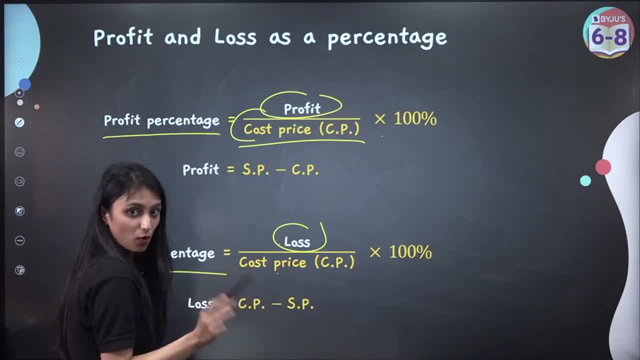 hai to into 100.. Again, loss upon cost price upon cost price hi hai into 100, kyunki percentage hai right. Aur profit kaise nigalta hai Selling price minus cost price? loss kaise nigalta hai Cost price minus selling price? I hope this is clear. koi doubt nahi hai, isme So. 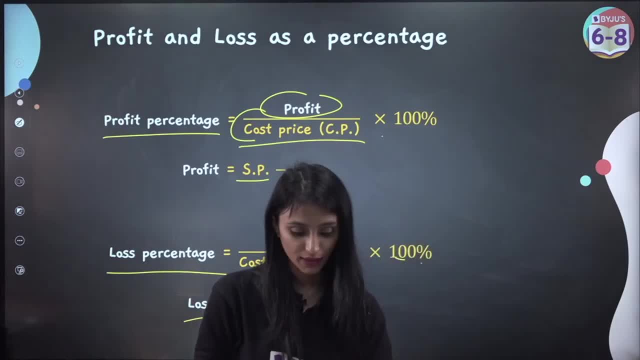 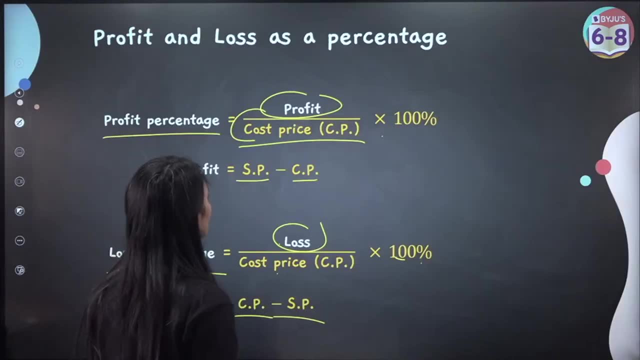 very soon. very soon, Sonakshi, don't worry, Karenge saare session, saare topics aayenge. Yes, who is saying Hindi? Dilshan Raza Bita, jab bhi aapka selling price, cost price se zyada. 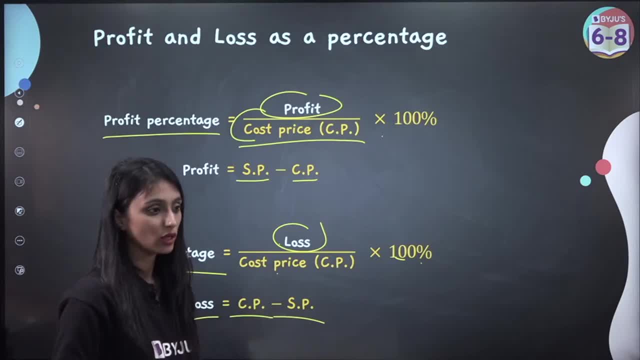 ho jayega right 10,000 ki cheez aapne khud khareedi aur aap 12,000 ki isko bech rahe hai. to definitely selling price zyada hai. to aapko profit ho raha hai right, Aur agar 10,000. 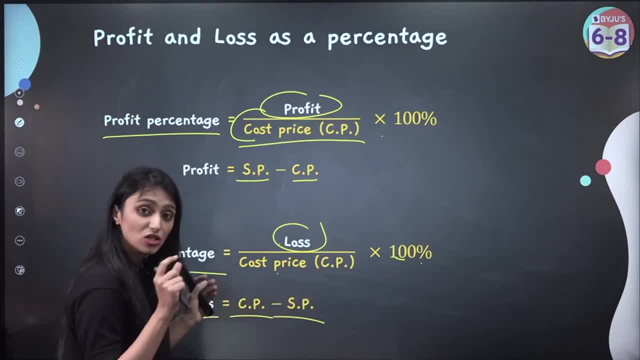 ki cheez, aap 8,000 ki sell off kar rahe hain, to aapko loss ho raha hai. Jab bhi inki percentage nikalni hogi to cost price par hi calculate hogi upon cost price, So you have to calculate. 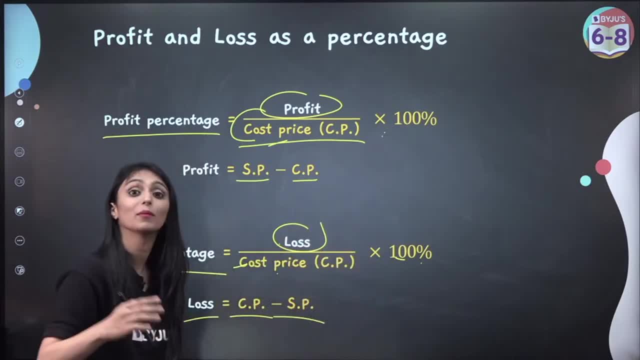 here only upon me, cost price, hi aayega in 200 karenge kyunki hume percentage me change karna hai, right? So this is the thing, Chali. let's move ahead. let's try out this question. 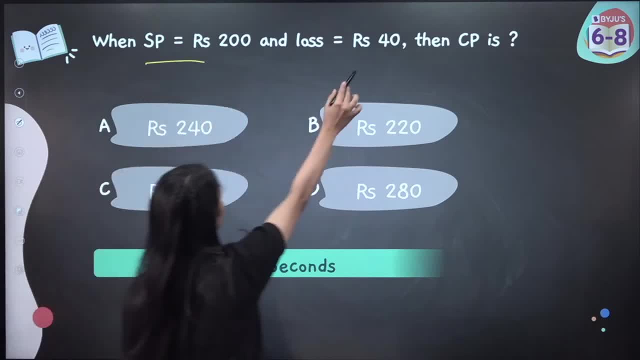 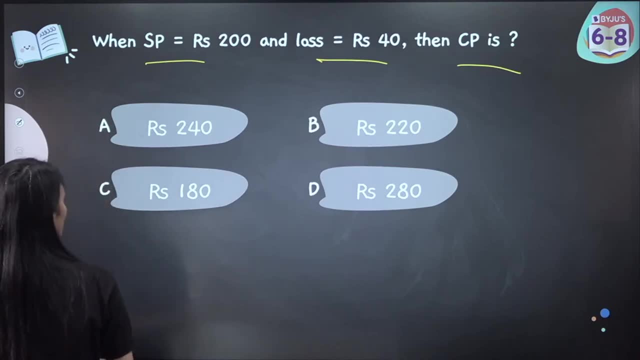 When selling price is equal to rupees 200 or loss is rupees 40, then what is the cost price? Come on, quickly calculate it. you have 30 seconds to answer this. Yes, try karo question jaldi se and let me know your answers in the chat. Kya answer aa raha hai? It's a simple. 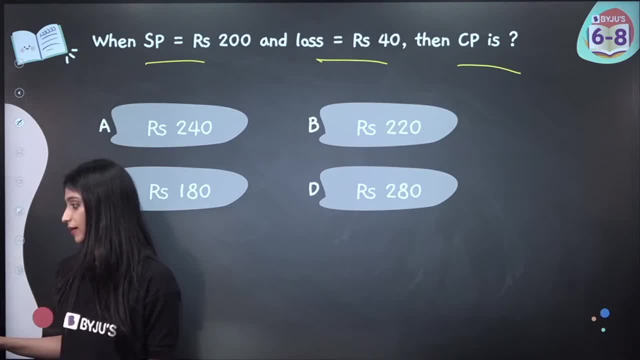 question. Yes, I can see answers here Right. so selling price 200 hai humare paas, aur cost price kitna hai and loss ho raha hai 40 rupees ka. So cost price kya hoga? We know one thing: loss. 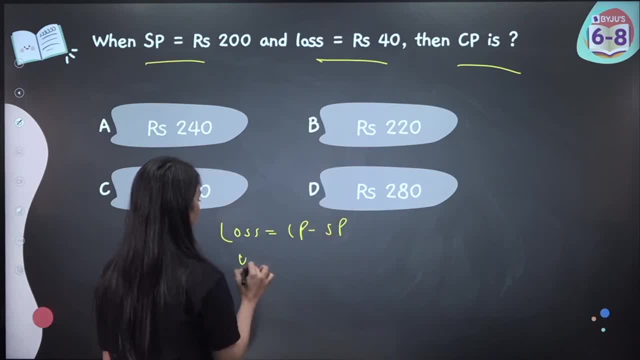 kya hota hai? Loss hota hai. cost price minus selling price. So what is loss here? That's 40.. Cost price: hume nikalna hai, and selling price is what? That's 200.. So cost price: 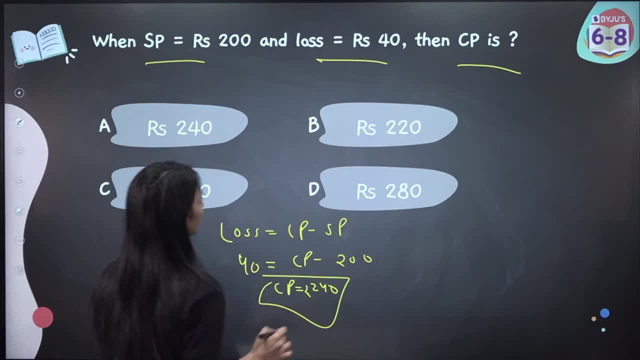 kitna ho jaga is case me 240 rupees, right? So 240 is going to be the answer, option A. So all of you have given the right answer. very nice. Now we move ahead to our last. 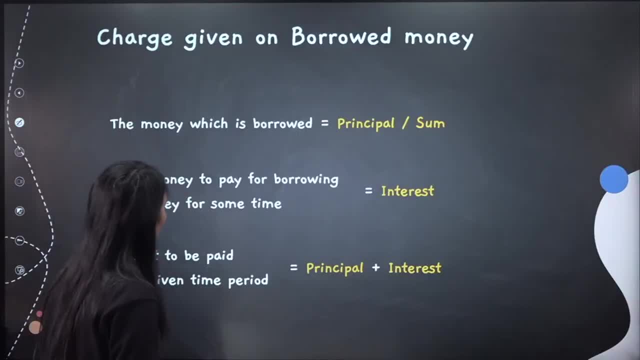 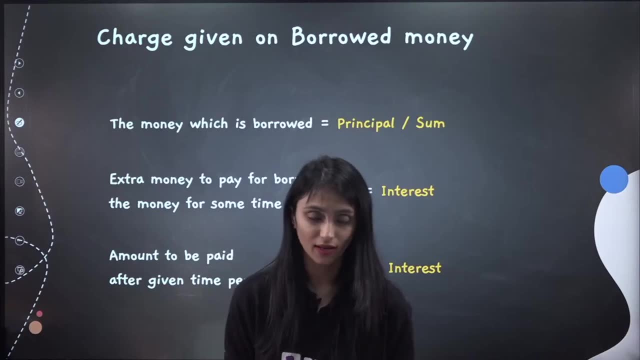 topic. that is simple interest. So jab bhi, let's suppose hum kisi ko, let's suppose aapne kisi se paise borrow kiye hai, aapne kisi ko paise diye hai, let's suppose aapne mutse. 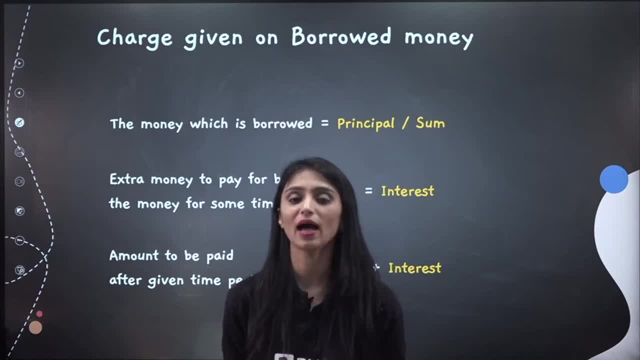 paise, borrow kiye 1000 rupees right And you say ki mai aapko, I will return this money to you after 2 months. How, what benefit am I getting in this? Mujhe kya benefit ho raha? 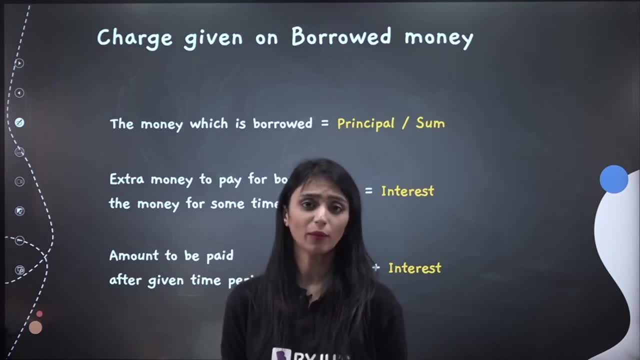 hai, Aap mutse paise le lete hai, aur aap mujhe 2 mene baad usko return kar rahe ho. I am not getting any benefit. So I say ki mai aapko ispe interest charge karungi, right Matlab mai aapko ye keh rahe. 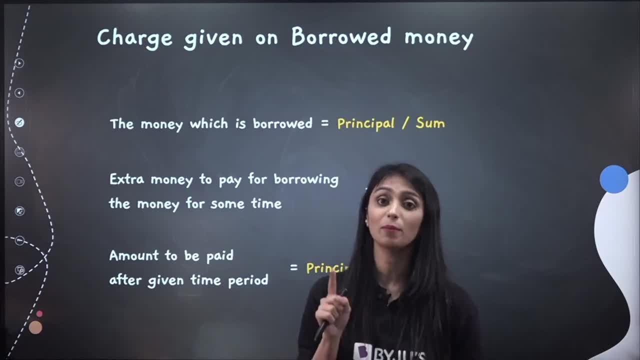 hu ki 2 months baad aap mujhe doge theek hai. aap mujhe 2 months baad doge, but aap mujhe 1000 nahi, aap mujhe 1100 rupees doge. So us 2 months mein maine aapse 100 rupees. 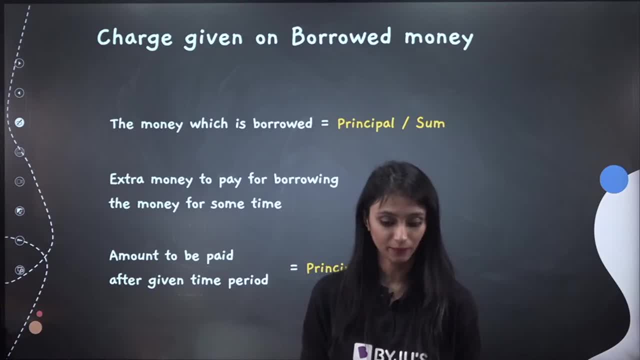 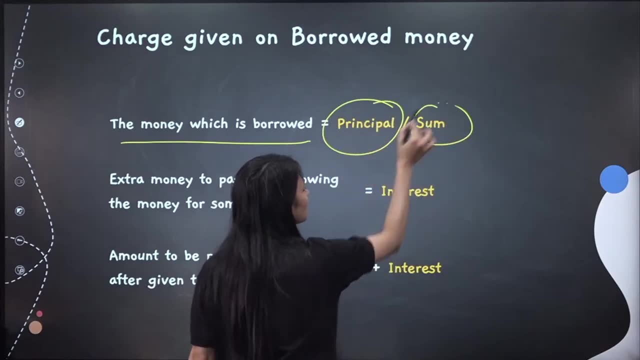 maine aapse 100 rupees aapse basically earn kar liye. Ye benefit hai mujhe. that's what we are doing here. So the money which is borrowed, usse hum kehte hai principle mathematical terms mein: yaa, phir sum theek hai And extra money paid for borrowing. So the money. 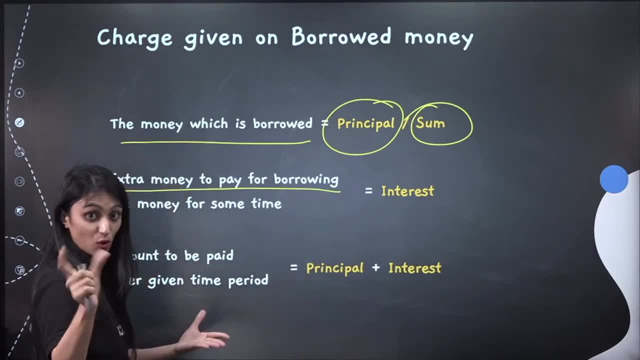 which is borrowed usse. hum kehte hai principle, mathematical terms mein: yaa, phir sum theek hai And extra money paid for borrowing. Jo aap extra money pay karte hai mujhe, main aapko 100 rupees bola, right The money for the same for some time. that is interest. 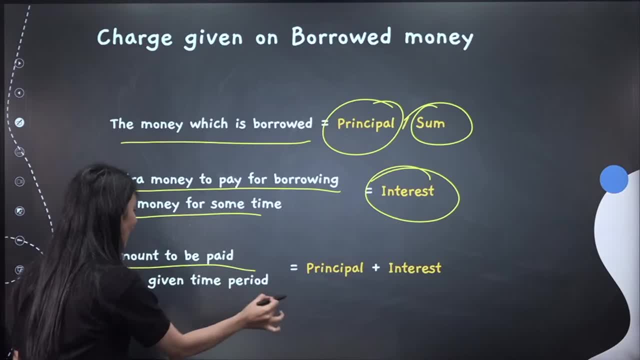 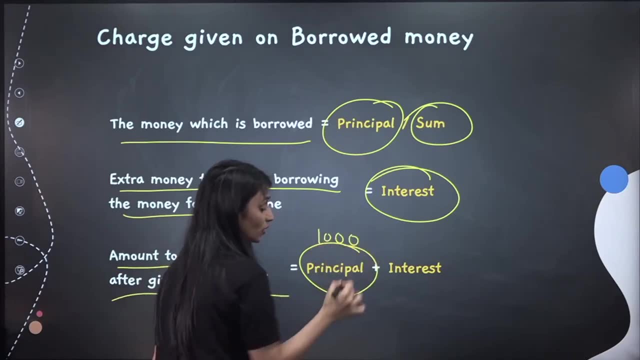 Wo 100 rupees was the interest, Aur jitna amount aap at last pay karte hai. at last pay karoge aap mujhe 1100 doge. That means you will give me the principle amount also, that is 1000, jo aapne mujhe borrow kiya. you will give me the interest also, which I 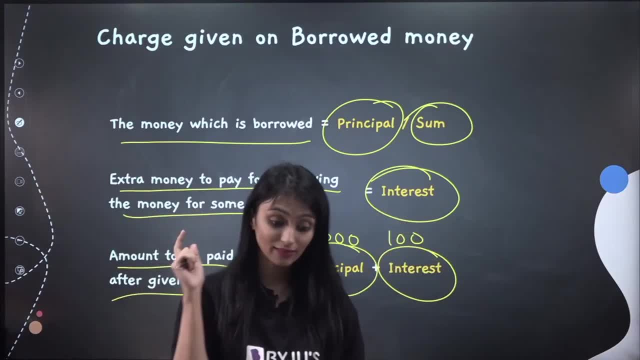 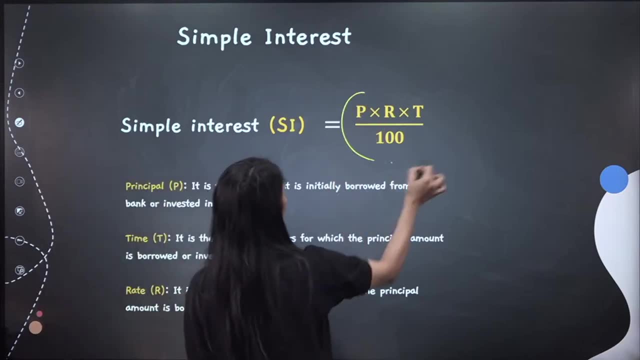 asked for, that is 100.. At the end, aapne mujhe 1100 diya. that's the amount Correct, absolutely right, Mani Ajit. Correct, absolutely right, Mani Ajit. So simple interest ka formula: kya hota hai? P into R, into T upon 100.. So principle is: 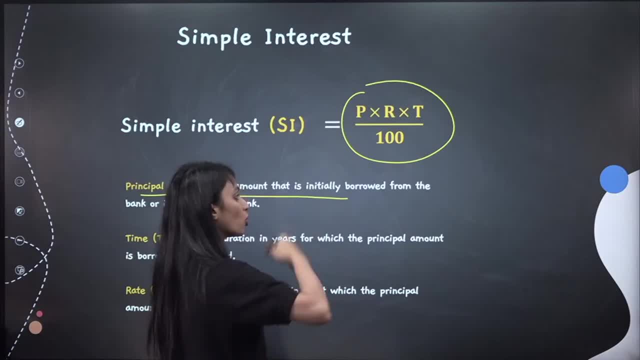 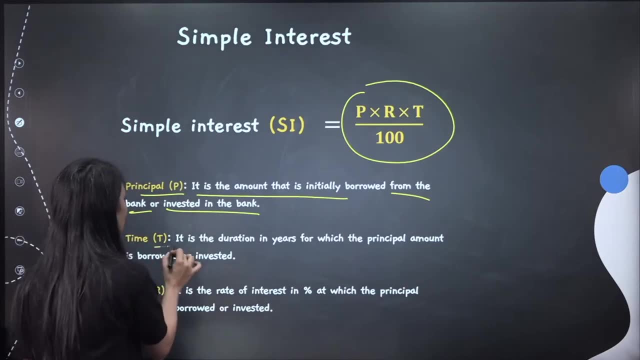 what It is, the amount that is initially borrowed- jo initially borrow kiya kya from the bank or invested in the bank, right Bank se bhi ho sakta. it can be from a person also Time, jitne time period ke liye, jitne duration ke liye. aapne kara, it can be in years. it. 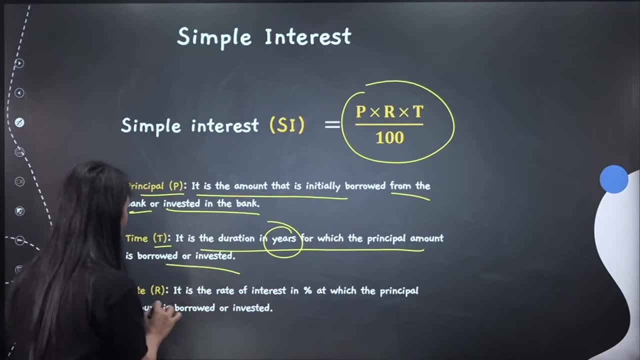 can be in months also. aisa nahi hai right Rate kya hota hai, Jaisa maine aapko charge kiya right? So it is the rate of interest in percentage mein hota hai, at which the 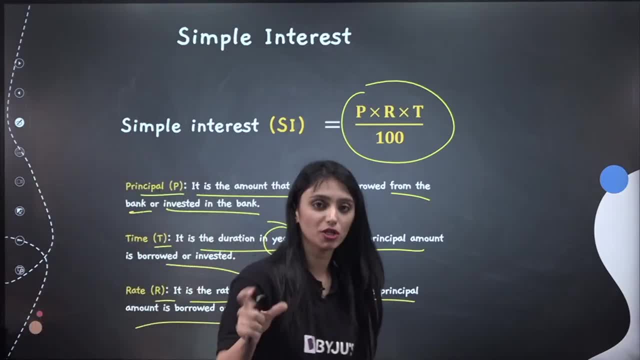 principal amount is borrowed or invested, So kuch rate of interest hota hai. jaisa, let's suppose, maine aapko bola 1000 rupees right Aur maine aapko 2 months ke liye kara. 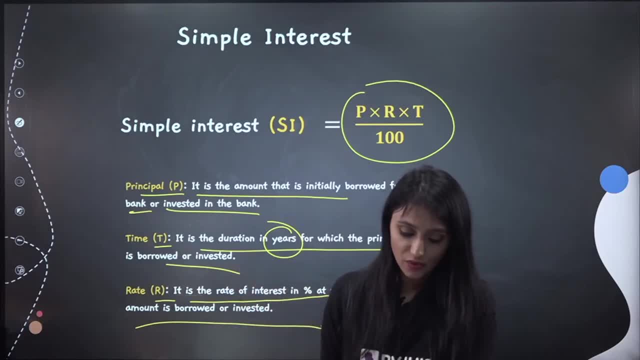 right. Is it for 8?? This is for grade 7,. this is for grade 7, right, Aur maine aapko 2 months ke liye kara to rate of interest. kuch bhi ho sakta hai. it can be 2%, 3%, depending bank. 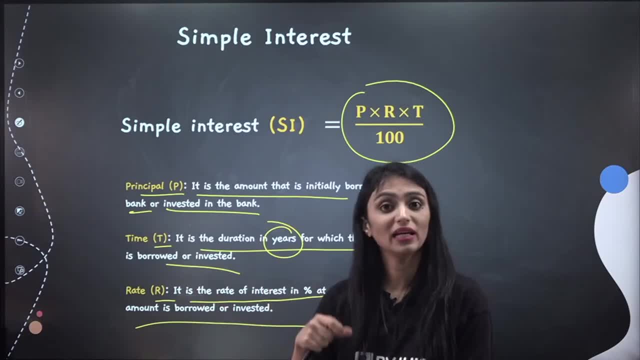 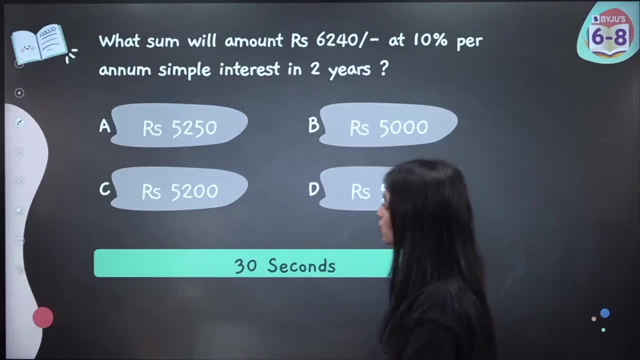 ki. basically, kya conditions hai, depending jis kisi aapkar kisi you are borrowing it from a person to us person ki apna, kya hai accordingly ho sakta hai? rate of interest? Let's try out this question based on the formula. 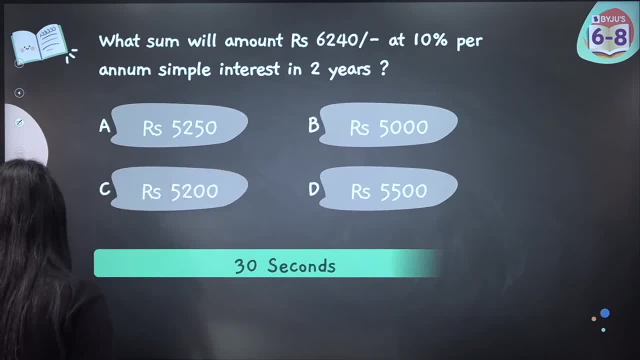 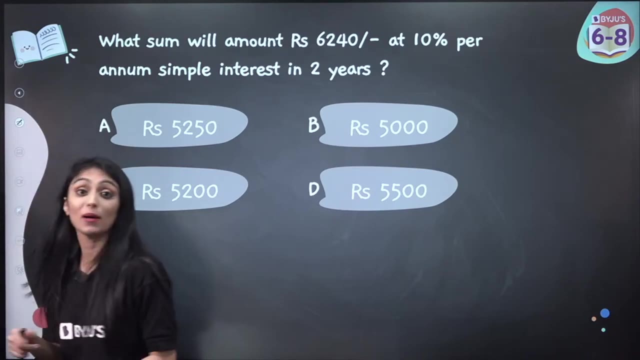 What sum will amount to 6240, right, 6240 at 10% per annum, simple interest in 2 years, and we have 30 seconds to answer this question. wo formula? use kariya and try this out. fattah vatse, Use the formula and try this out. iske baad menti hai. come on, everyone Iske baad. 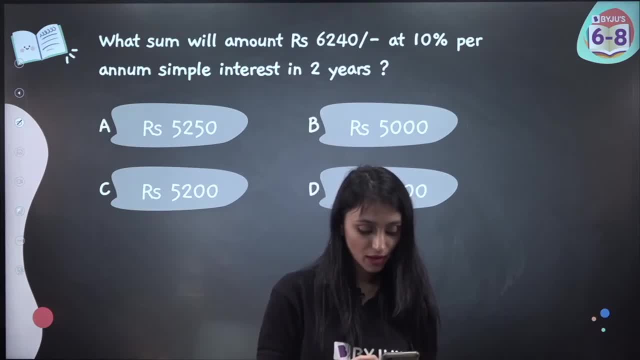 menti karenge ham log P N R. P x R x T x 100. dania P x R x T. P is principal, R is rate of interest, T is time matrix. so these are 2 hundred. So if you use this formula, you 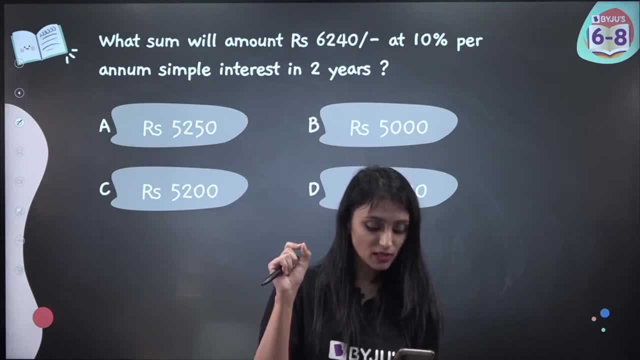 rate of interest. t is time period S, Nagendra. that is not for compound interest pitta, that is for amount, Amount minus principal karoge. toh you will get the compound interest Prathna. this is not for 8 pitta, this is for grade 7.. 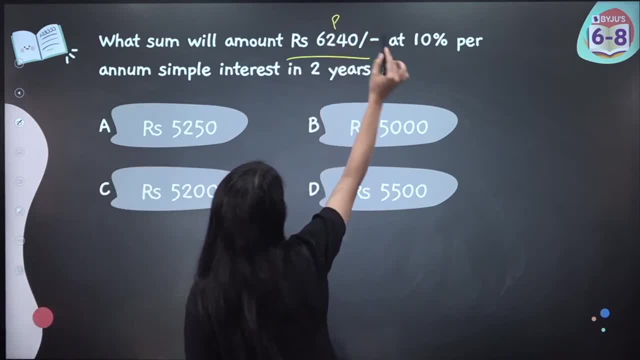 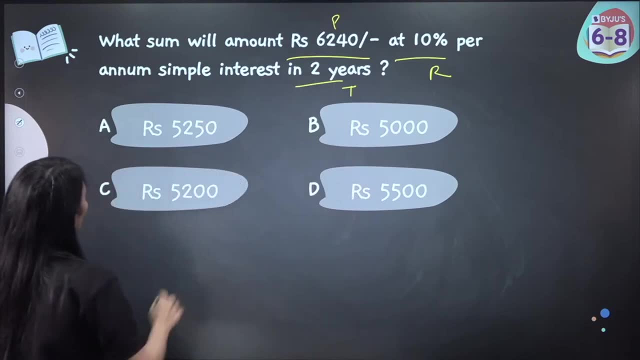 Okay, let's try this out. This is what. This is. principal right Rate of interest is what? 10% Anam simple interest time is 2 years. We have to calculate the amount too. I'm sorry, This is the amount and this is the. we have to calculate the sum. So amar ko kya pata. 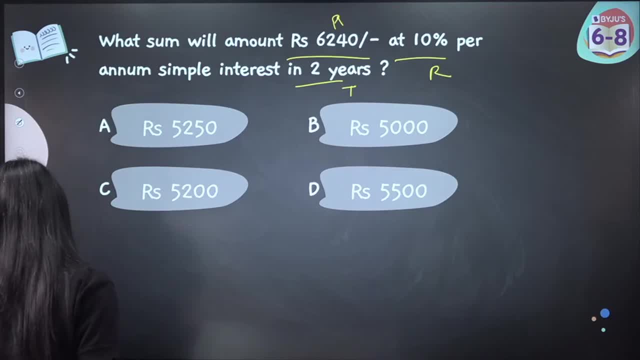 hai. We know hume sum find karna hai. yaha pe right, We know. let's suppose wo amount jiske hum baat kar rahe hai, sum ki. let that be x. So simple. interest kya hota hai P into? 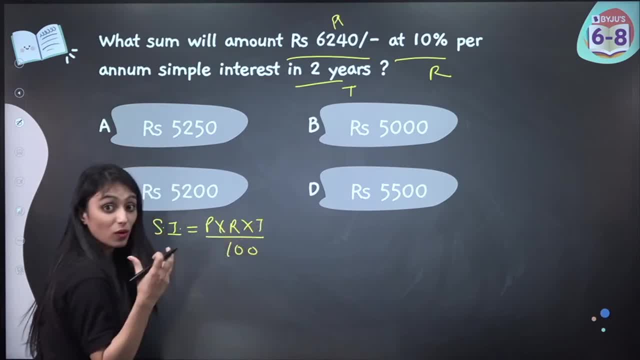 R into t upon 100.. We don't know what the principal is, what the sum is. Hum isko le lete hai. let's suppose x Rate of interest is what, That's 10%. Time is what? 2 years? 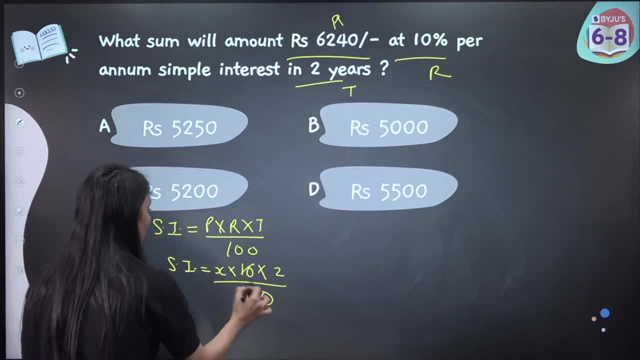 upon 100.. Thik hai Ye, clear hai ye, kya aagaya Cancel out ho gaya. So, simple interest, aap ke paas aagaya X by 5.. Simple interest aagya x by 5. Amount, kya hota hai, Finally, jo amount aata hai. 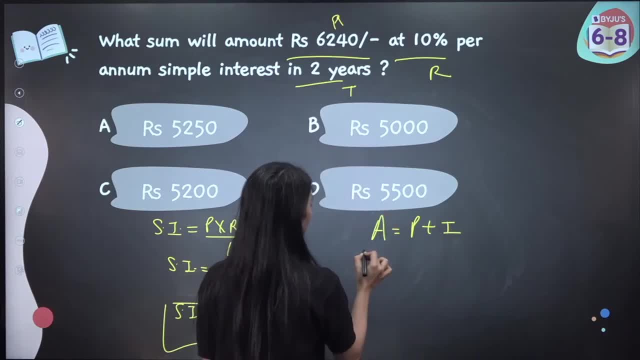 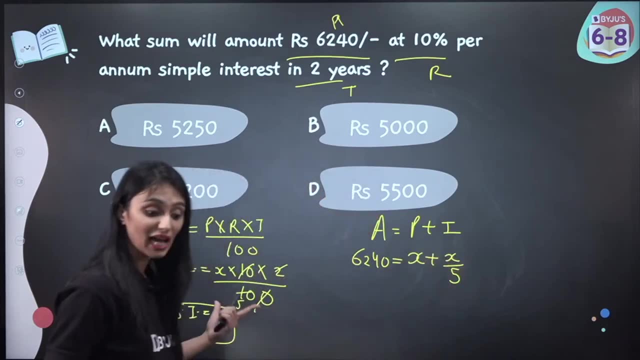 wo aata hai principal plus interest Aur amount kitna kya ho aapko 6 to 40.. Principal kitna tha aapka X Aur interest abhi humne kitna nikaala X by 5.. Yaha, se we can calculate. 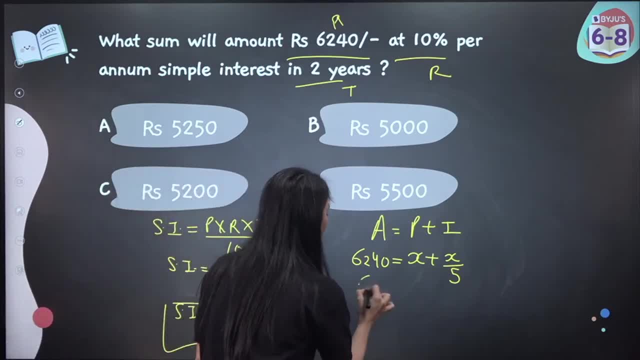 the x. Yes, I can see answers in the chart very nice. So here this is 6 to 40. Ye ban gaya 5x plus x upon 5. That's going to be 6x by 5.. So 5 ko yaha le jaate hain, 6 x by. 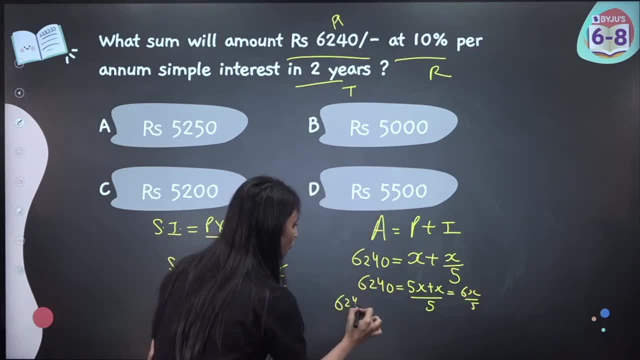 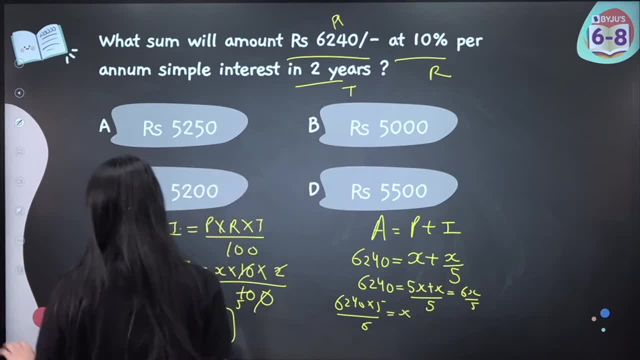 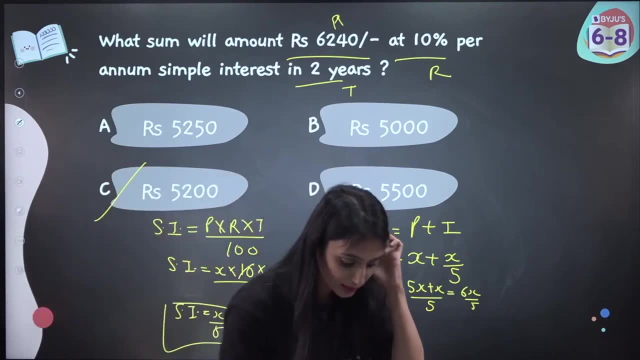 hain 6 to 40 x 5 upon 6.. What is the final answer? Calculate kar ke kya aar rahe 5200.. Option C: That's the right answer. That's the sum 5200.. Yes, Amrita, I think you've. 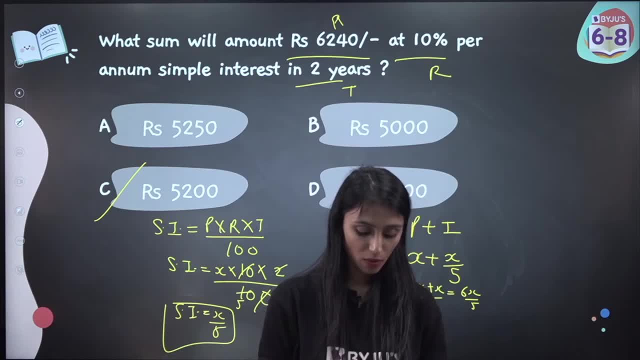 just joined Students jo late join kar rahe hain, first time aa rahe hain, they don't know about these classes. please first subscribe kariye channel ko: Niripta, Dilshan, Shaghun, Amrita Janhvi, Siti, Song and Dance. please subscribe the channel. hit the bell icon also. 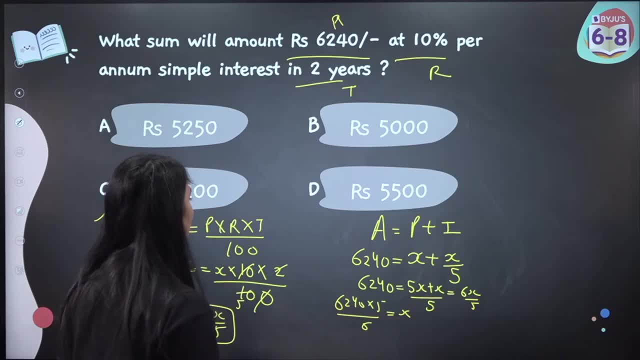 Aapko notifications mil jaayenge Amrita Janhvi Siti Song and Dance. please subscribe aapko notifications mil jayangi. you will not be missing on any of these sessions. then 5200 is the answer. Now quickly quickly go to menticom. yes, everyone chaldi se fatta. 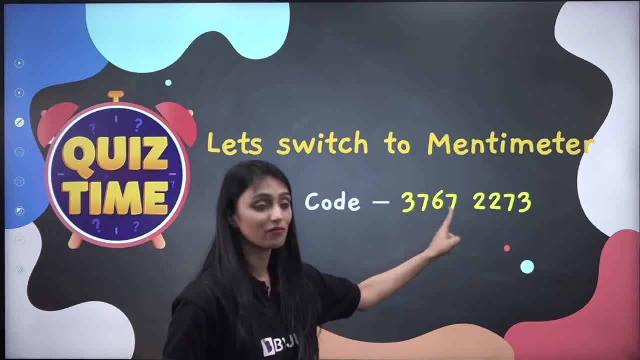 fatte menticom pe jao use this code: 37672273,. this is the code. quickly go to that join karke. let me know in the chat ki ma humne join kar liya hai. meanwhile I will also switch. 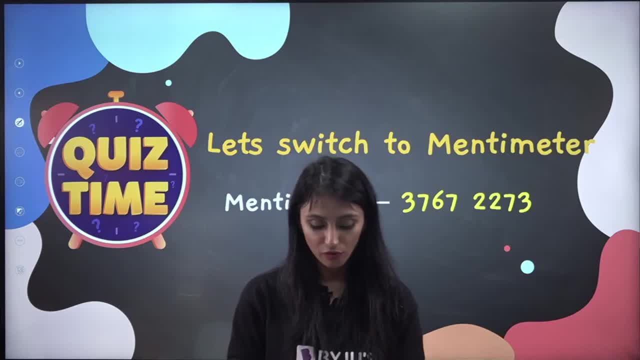 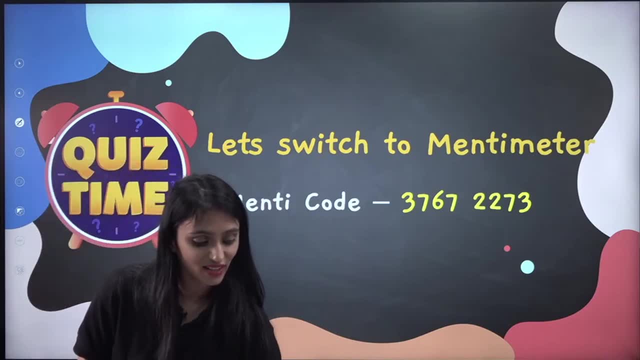 the screen. Alright, so I will be back in another 3-4 seconds. okay, quickly, aap to tak join kariye using this code. Yes, Esna Kendra. I know I know next session hai, but menti ke baad we will join, Alright. 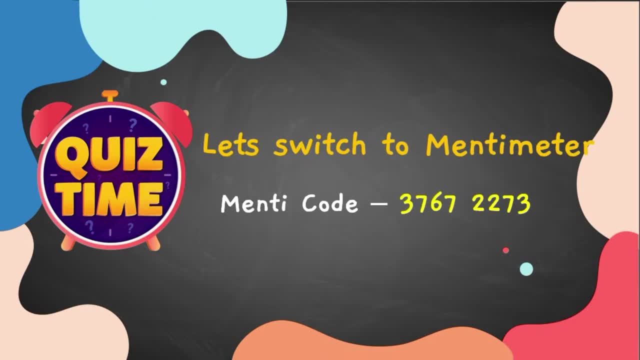 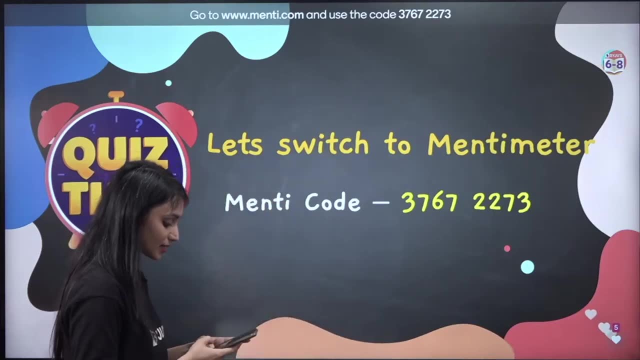 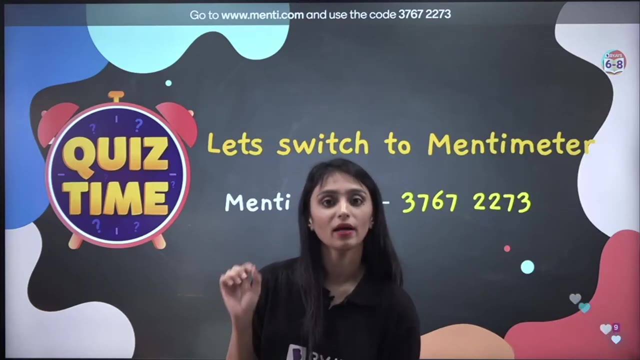 Hey, everyone quickly join kar liya. sab mein join karke Dilshan. it is very simple, just go to menticom. go to menticom and use this code. aap se code mangayega 37672273. 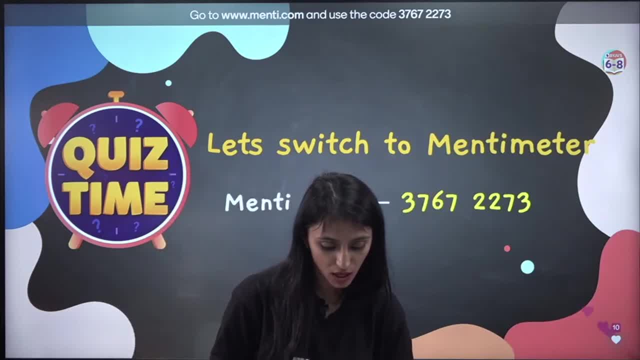 aapko put karna hai, aapko ish join kar payenge. Yes, Aram Jaha Amritansh joined Dilshan Raza. I hope samajh aage hain. Yes, Aram Jaha Amritansh joined Dilshan Raza. I hope samajh aage hain. 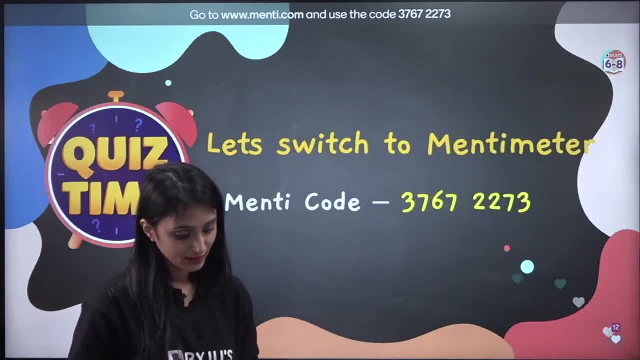 jo first time aaye hai, class ke liye menti kaise join karna hai. Yes hi, Anjula Esna Kendra joined. So students who are coming for the class for the first time, please subscribe and if you are enjoying the session also, sabkuch samajh aaya session mein to please. 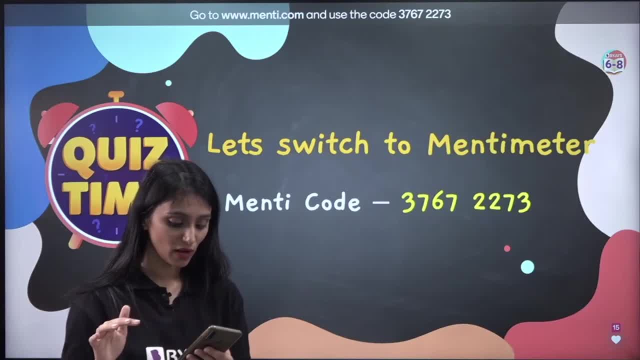 like bhi kariye session ko. Come on everyone, Farawatse. yes, yes, yes, Pawan Gamer, I am waiting, I am waiting. Farawatse, join karo aur chatne mujhe batao. yes, Mona, join, light Yagami. 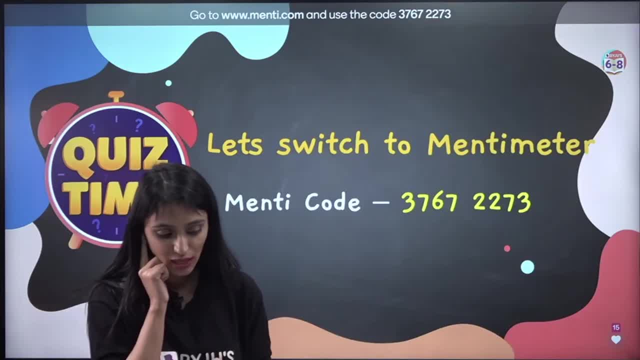 Gaming hi, Aapko bhi new students hai. please channel ko subscribe karlo, because aap log bohot sara sessions aap aise miss kar dete hain, because aapko nahi bata, ki yaha par kaunse sessions. 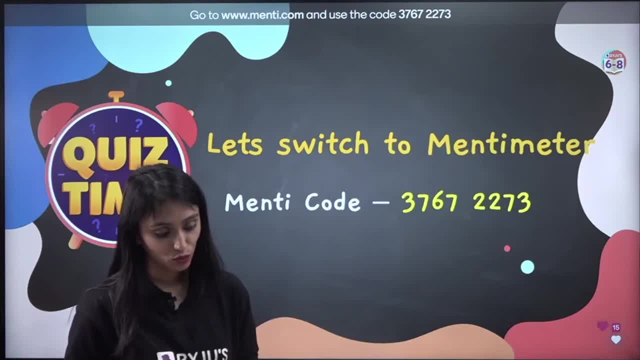 hota hain. kab hota hain? Yes, Ramavtar Bhati, I am good. how are you First time right In my class or first time to the channel? Ananya Singha, Esna Kendra, yes, Yes, mujhe. 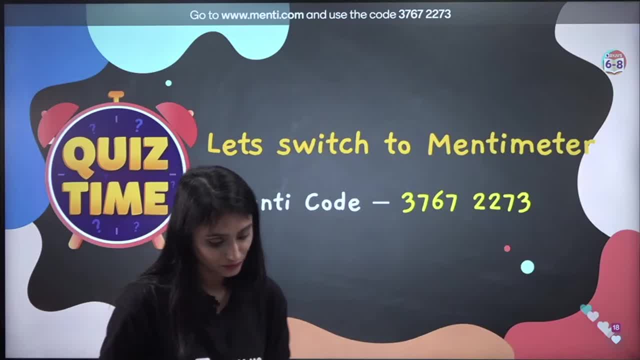 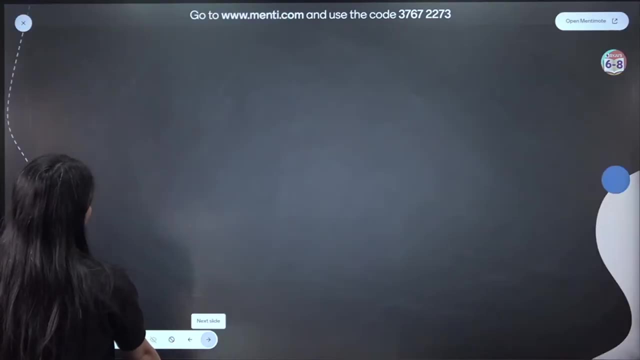 bhi 8th class bhi karna hai. ye menti karke, we will start with class 8.. Yes, Pratiksha, yes, Anvi, ready Start kare. Chaliye, let's get started. Alright. so 5 questions hongi hai menti mein total and. 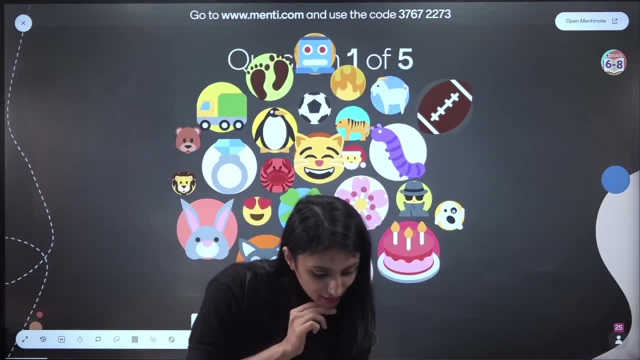 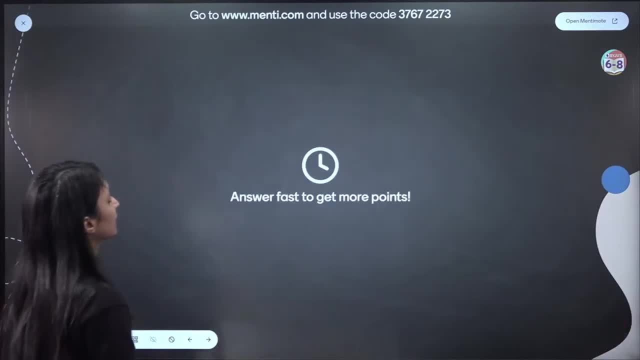 I can see some students have joined. yes, hi, Sanjay, jaan, Avni, everyone, jo bhi new students hai. please channel ko subscribe karo, because, as I said, bahut saar sheethe aap log miss out kar dete hain. phir Okay, let's take a look at the question Priya was preparing. a cake. She mixed 3 cups of flour, 2 cups butter and 1 cup of butter. She mixed 3 cups of flour, 2 cups butter and 1 cup of butter. She mixed 3 cups of flour, 2 cups butter and. 1 cup of butter and 1 cup of butter. She mixed 3 cups of flour, 2 cups butter and 1 cup of butter. She mixed 3 cups of flour, 2 cups butter and 1 cup of butter. She mixed 3 cups of flour and. 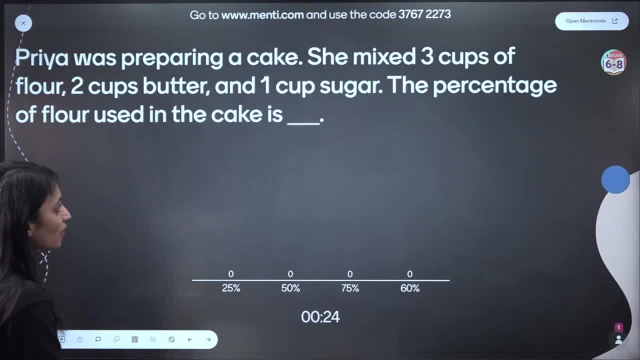 1 cup of butter and 1 cup of sugar. The percentage of flour used in the cake is Kitna flour ka percentage use. kiya hai 3 cups flour, hai 2 cups butter, hai 1 cup sugar, hai Chaliye. 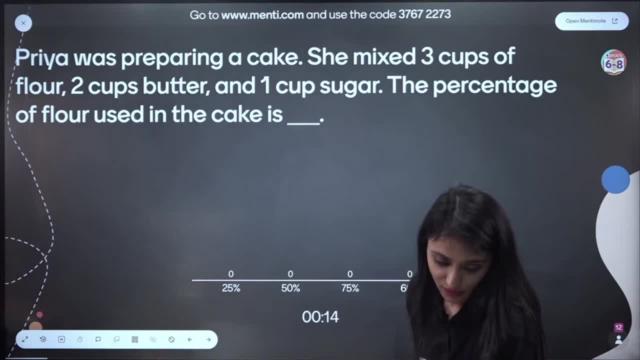 fata ftse Reise star? are you asking me bitta or are you telling me Yes? Kartavya hai Anita Ritika. Grab Coming first time Ram Aftar Bhati. So please, new student, bahut saare. 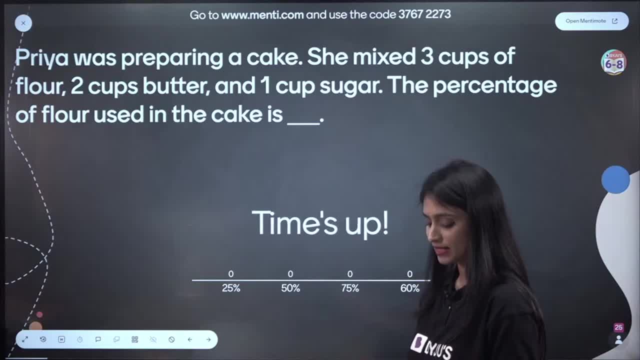 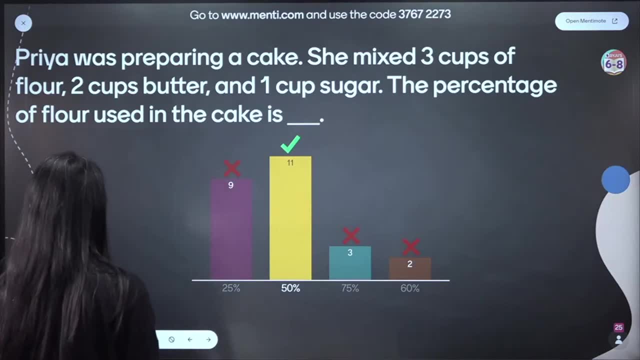 session. aap log aise hi miss kar dete hain. Entire session almost over ho gaya tha. please subscribe kare. Ankur Bhuvan. yes, 50%. this was a simple question. what happened in this? it was simple: 3 cups. 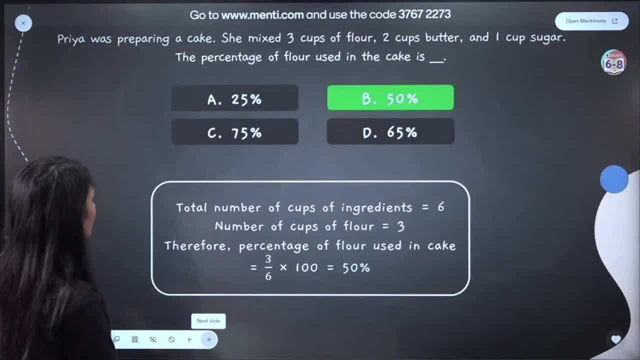 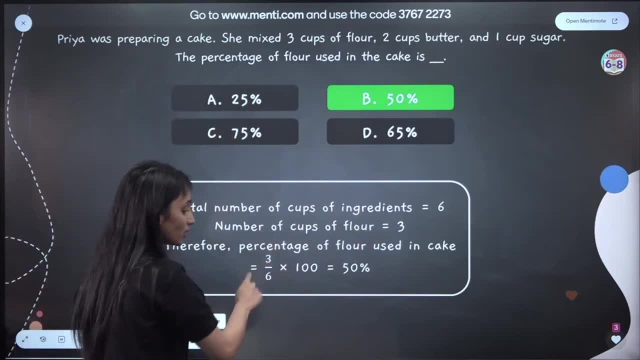 flour, 2 cups butter, 1 cup sugar. so, while using all of them, what is the total ingredient? 2 plus 3 plus 1 is 6, we have to get the flour, so 3 upon 6 upon total, into 100, because the 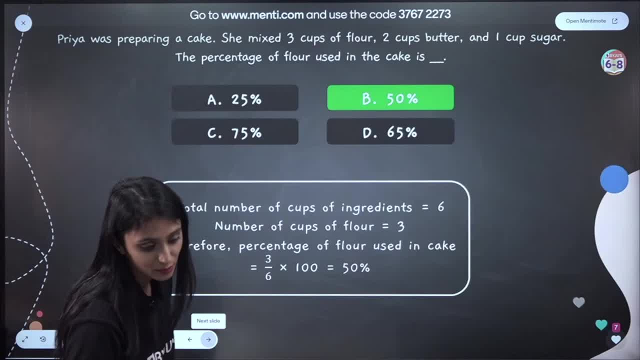 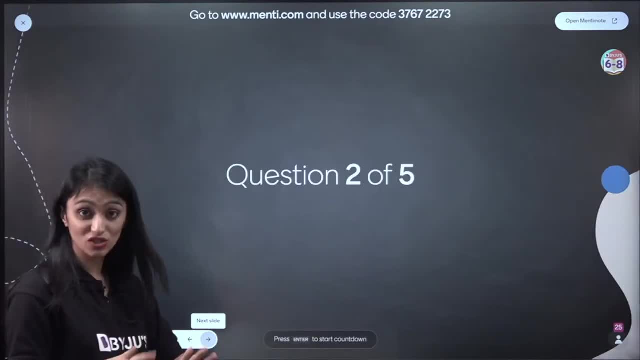 percentage is like: this is 50%. that's the answer. it was simple. Anjula Jodhallyan new right: subscribe kiya pehle, subscribe kariye beta, agar nahi kiya toh and session samaj. 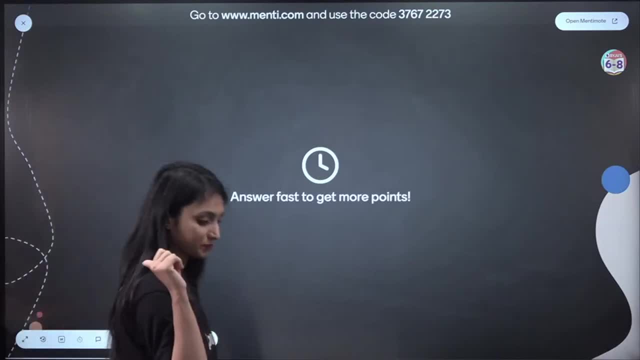 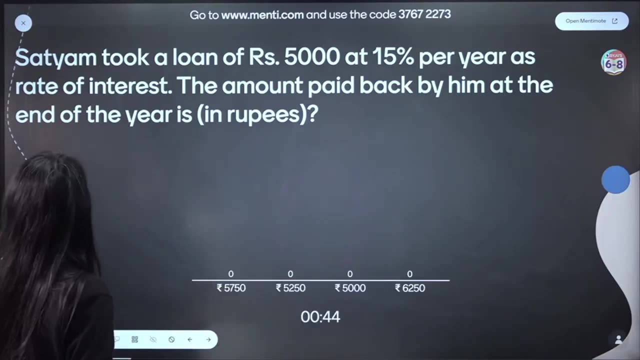 aara hai. I think you just joined, agar lag raha hai. useful hai, toh please like bhi karo session ko arey. koi baat nahi, mona, it's ok, chalte rehta hai. alright, Satyam to took. 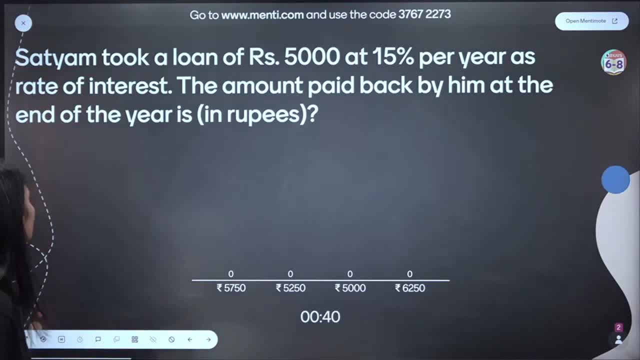 a loan of rupees 5000 at 15% per year as rate of interest. the amount paid back by him at the end of the year is in rupees. in rupees kitna aayega Loan liya 5000 ka. 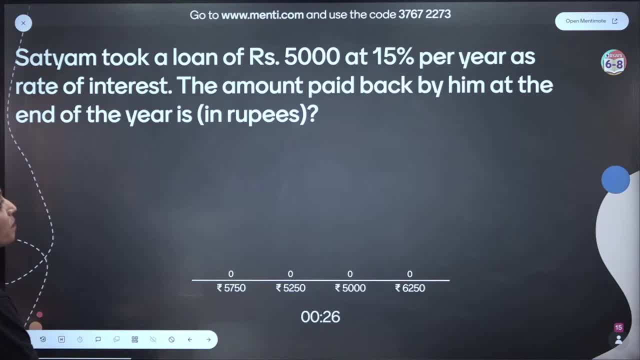 15% per year rate of interest. bhi aagya amount paid back by him at the end of the year. time diya bhai, 1 year amount nikalna hai principle, hai rate, hai time hai amount. 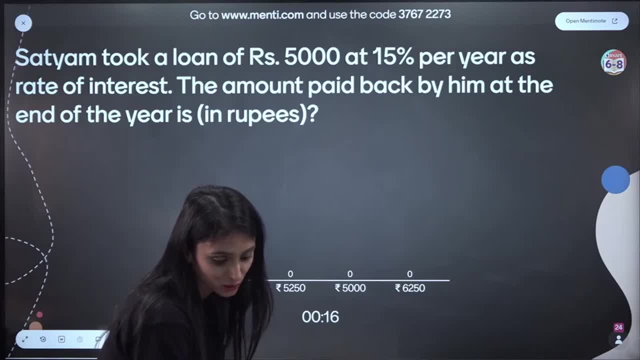 find karna hai answer? mujhe dekhna hai. Nirmal Kumar Gupta: 5250,. accha, ye answer hai. abhi dekhte hain. chalo, farafat, se jinko bhi session samaj aara hai. useful laga hai? please subscribe? 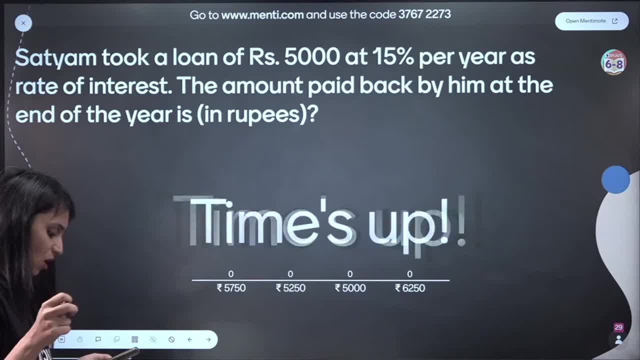 bhi karo channel ko and like the session also Kaunsa session. Kaunsa session chal raha hai, Shakuntala. this is comparing quantities. grade 7, yes, come on, everyone chaldi se Balraj Salan. jo bhi new students hai, please subscribe also. 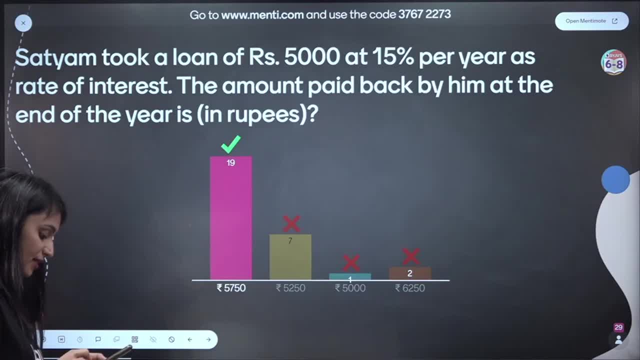 yes, Nirmal Kumar, abhi 8th ka session bhi hai, anthe ka. once it gets over, tab hum next session grade 8 ke liye hi hai. ok, answer is 5750,. let's quickly take a look kyaise. 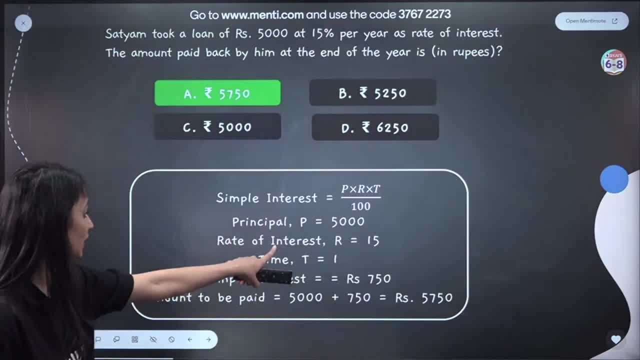 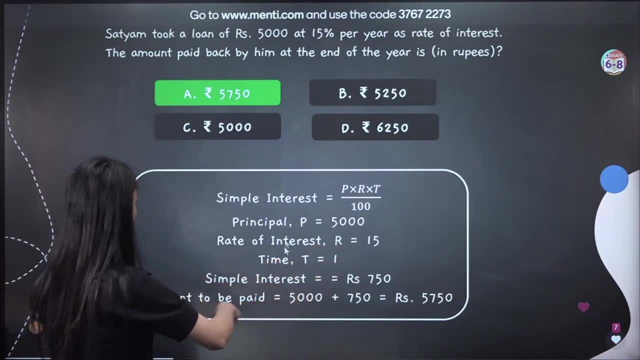 nikaala hai simple interest: P into R, into T upon 100, principle hai, rate bhi hai, time hai 1% right. So simple interest kya hai? kaise niklega? isme put karke 750,, so amount to be paid aapke. 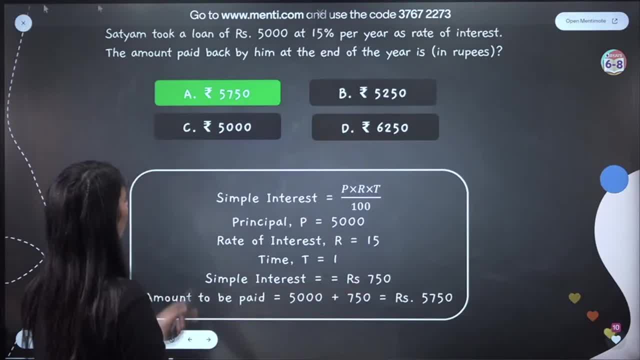 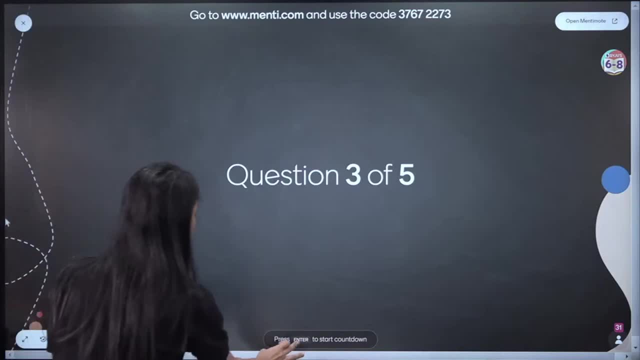 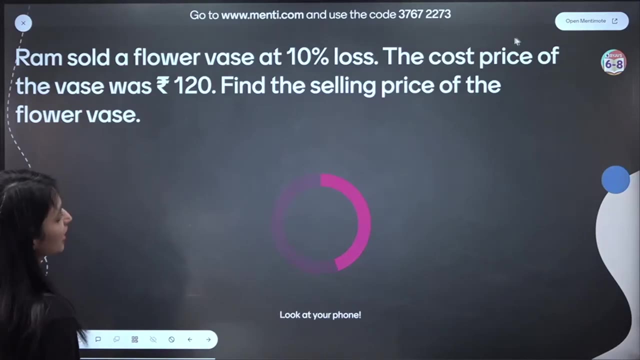 paas kya aega. 5000 plus 750,, that's 5750,. option A: that's the right answer. right chal ye. let's move ahead now. Question number 3,. ok, so Ram sold a flower vase at 10% loss pe and cost price tha uska. 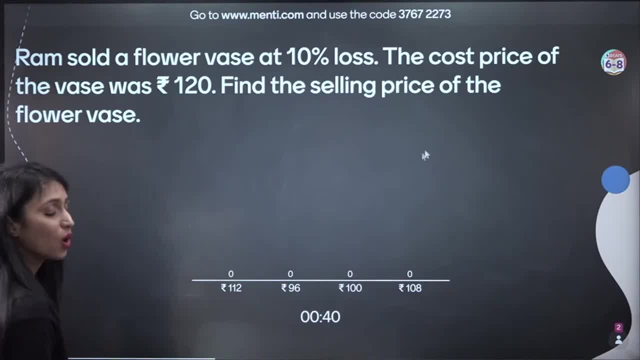 120, find the selling price of the flower vase. Aapko loss percent pata hai. aapko cost price bhi pata hai. aapko formula. maine bataya tha loss percent ka loss upon CP into 100, aap wahan se cost price nikaal sakte ho aapke paas loss. 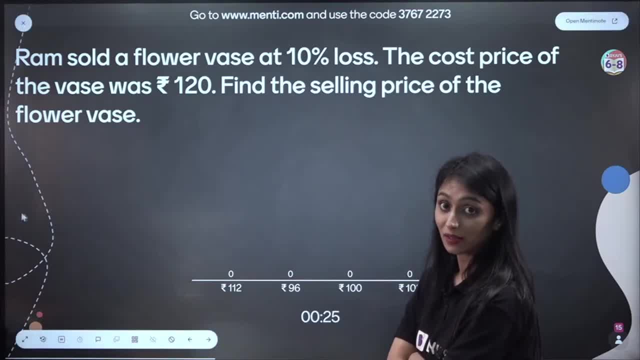 bhi hai, aapke paas, I mean aapke paas loss aa jayega cost price bhi hai. then you can find out the selling price right. Chal ye farawat se, farawat se. yes, kya hai. 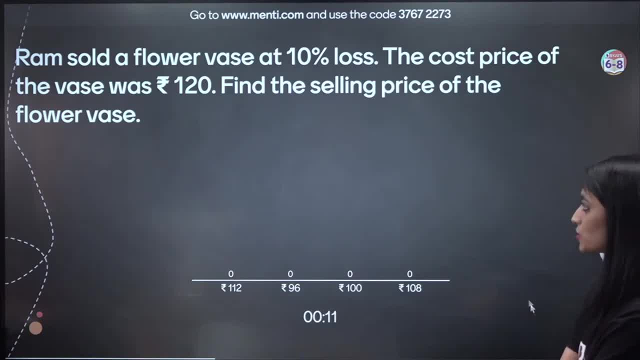 Farawat se, Farawat se, Farawat se. Karon aap hangar kya aega answer quickly. let me know in the chat: Bhagya dar oja beta. bohot simple hai. aap simply chrome par, agar aap android use kar. 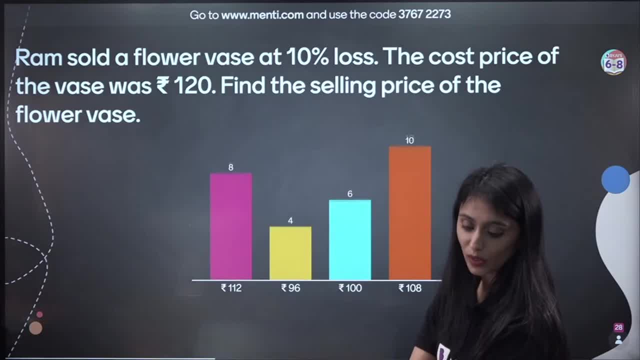 rahe hain. simply aap jaayegi wwwmenticom pe, aap click karoge, it will ask you for a code. Yes, ask you for a code. wo code put karna, jo upar likha hai: 37672273, 108 is the answer. 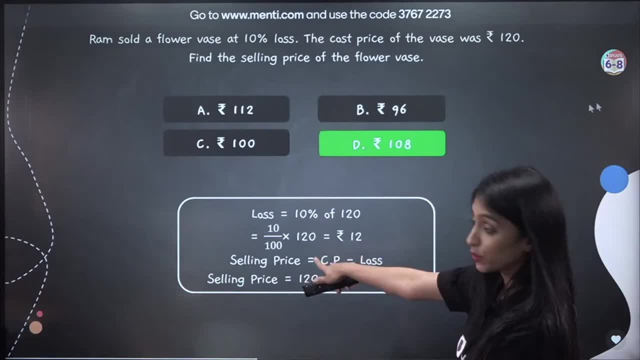 chalo, let's take a look: Loss. maine kar ata ye formula aap use karo: loss is loss, percent is loss upon 100 into upon cost price into 100, wahan se aap loss nikaalenge Rs 1.68.. 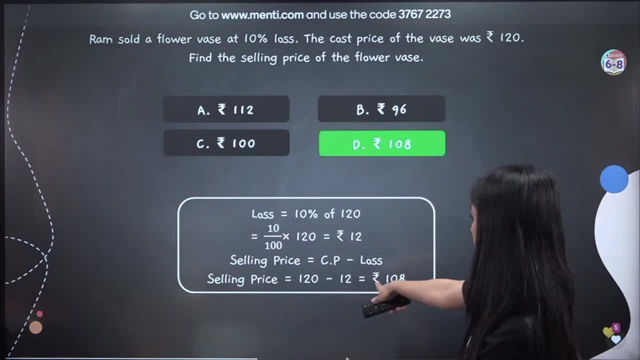 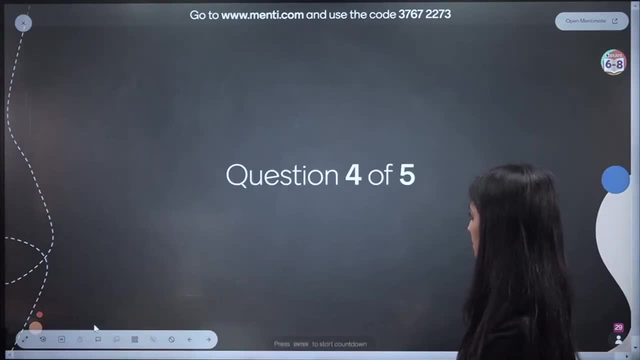 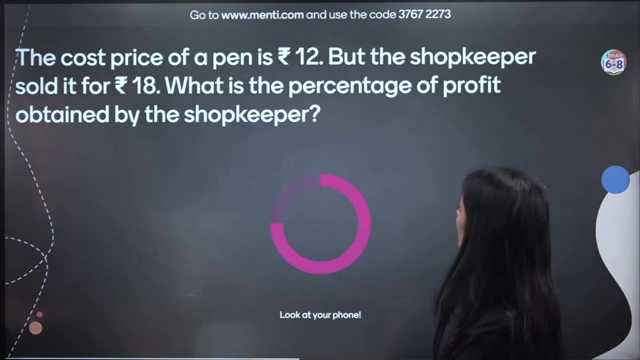 loss nikaalenge rupees 12.. Selling price: hota hai cost price minus loss, that's going to be 108.. So option D is the right answer. Right, chaliye. let's move ahead now to the next question, Question number 4,. yes, the cost price of a pen is rupees 12, but the shopkeeper 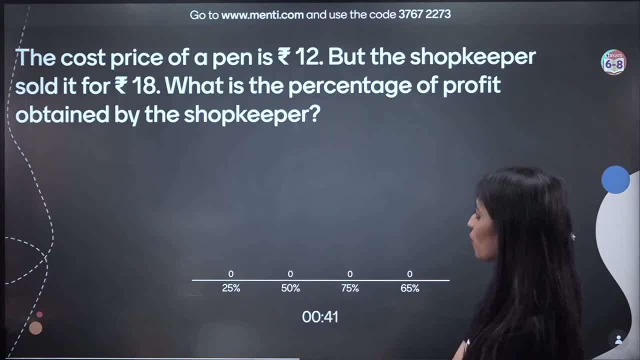 sold it for rupees 18.. What is the percentage of profit obtained by the cost shopkeeper? Cost price de diya aapko CP given hai, but the shopkeeper sold it for rupees 18, selling price bhi given hai. Right percentage of profit. nikaalna hai aapko Right percentage. 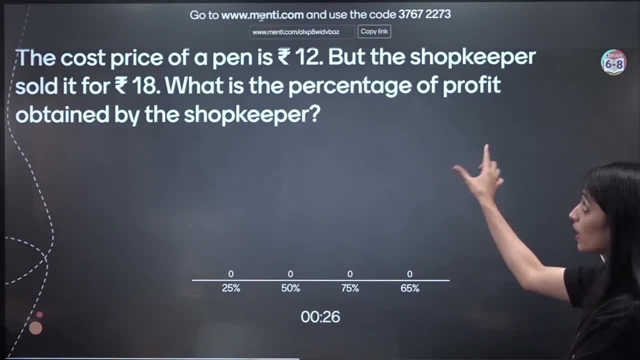 of profit. profit percent nikaalna hai, Jiske liye pehle aap profit nikaaloge upon CP into 100.. Aapko profit percent nikaalna hai, Jiske liye pehle aap profit nikaaloge upon CP into. 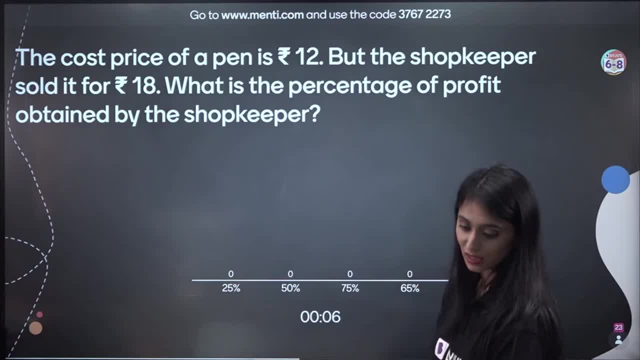 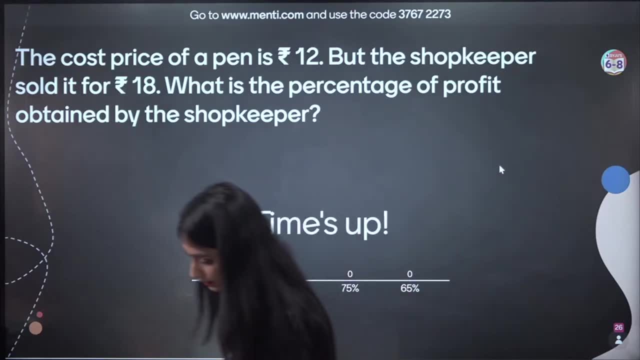 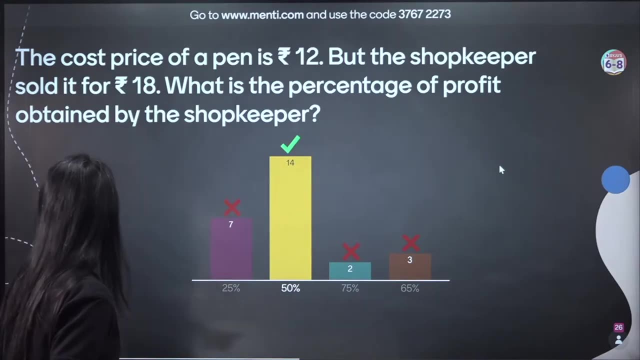 100.. Yes, so what is the answer? kya aayega 50, arre acha tu enter your name: haan, haan, haan, definitely, definitely, I will. I will Jaldi se 50 percent. that's going to be the answer. 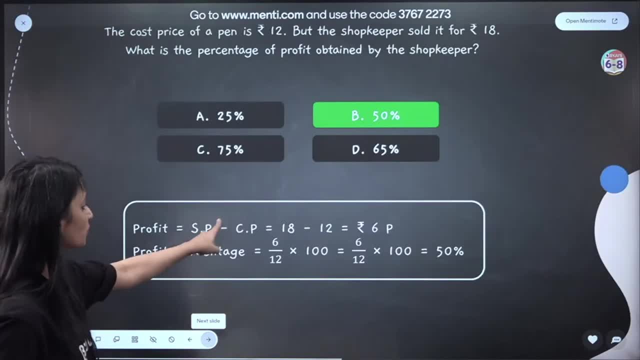 Chalo. dekhte hain, kaise ye answer aa raha hai. profit kaise nikaaloge? cost price minus selling price aa gaya 6 rupees. Right, that's the profit. Profit percentage kaise nikaalta? 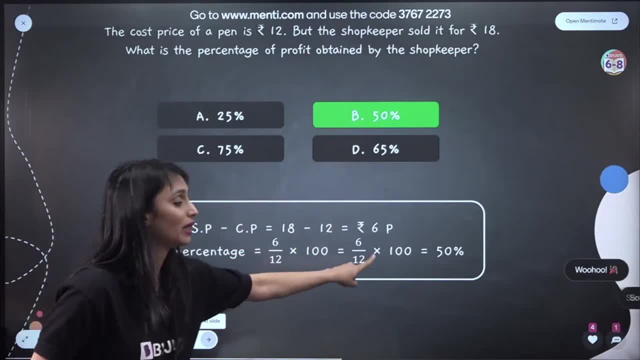 hai profit upon CP into 100.. Matlab 6 upon 12 into 100.. Matlab 6 upon 12 into 100.. Ye aa gaya aapke paas 50 percent Clear sabko, 50 percent answer aayega. 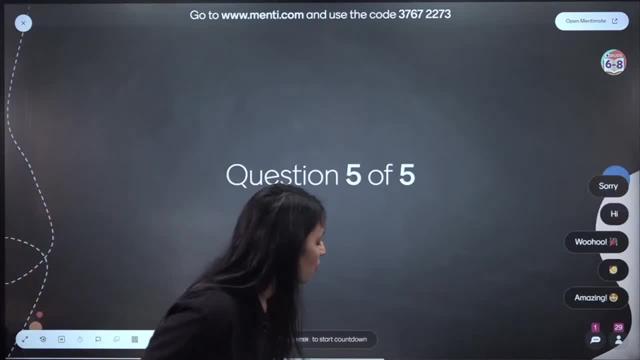 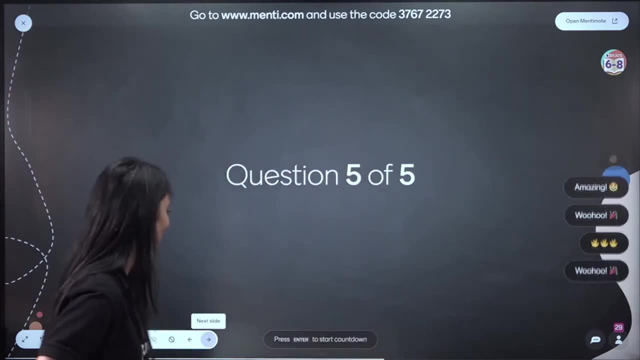 Chalye, let's move ahead now to the next question. wow, wow, I can see your chat here also amazing, Chalye. let's move ahead now to the next question. maza aa raha hai. yes, enjoy kare ho session. 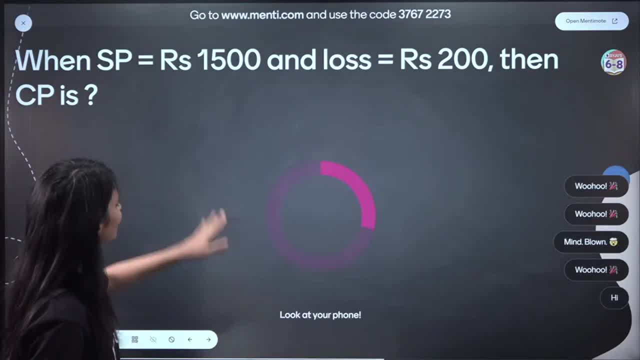 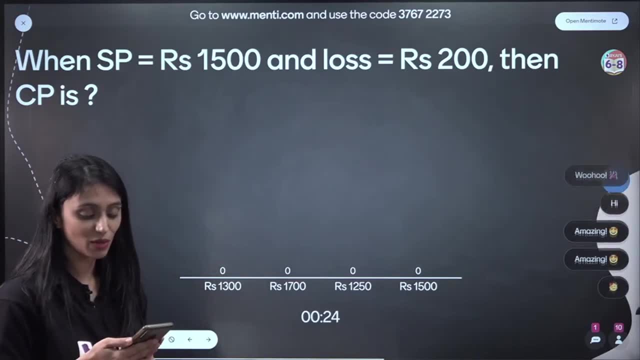 toh vada bache like like karna. toh banta hai. Selling price is 1500 rupees, loss is 200, then CP is simple se formula hai: come on everyone, Ma'am class 8, mein life kab ahoge beta jaisi ye khatam hoga. na, just give me 5 minutes. 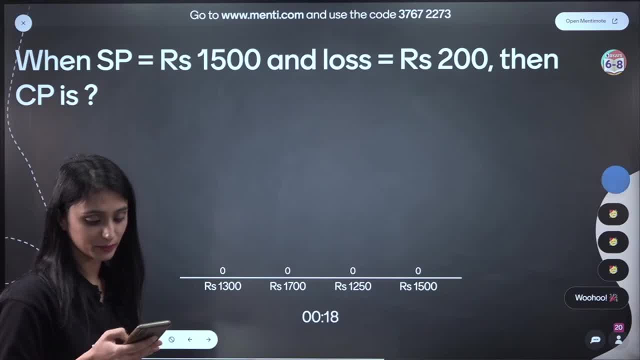 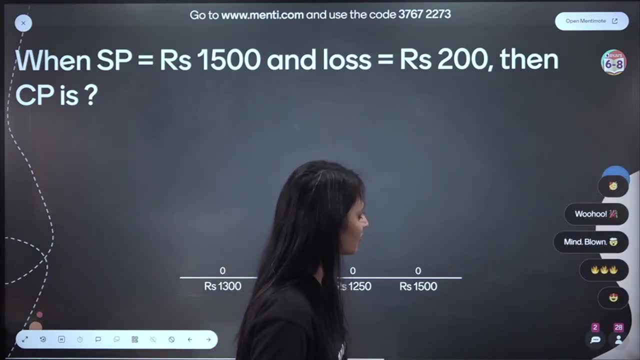 maximum. then we will start with class 8, don't worry, But I know there is no point rushing, because aise samajh nahi aega aap log ko. Wow, this is amazing. this is, I think, our new feature. 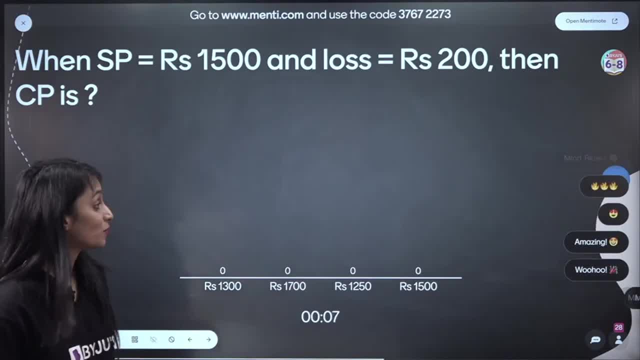 Yes, Nirmal, everyone wow. but. but but agar session enjoy karo hai, sabko samajh aaya hai na like likes, toh banta hai and jino ne subscribe nahi karo hai, please subscribe. 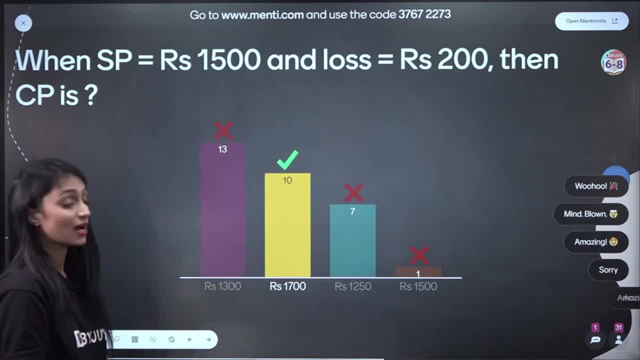 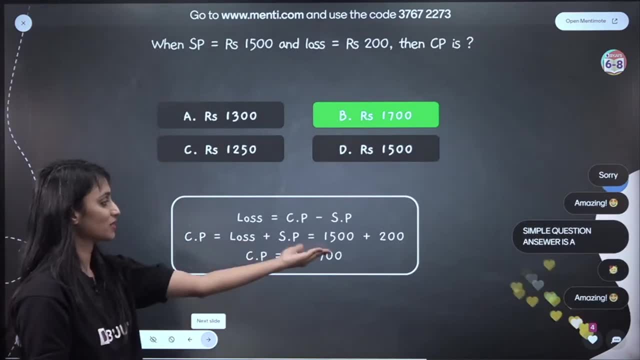 also because bahut baar aap miss out kar dao aate ho sessions aise hi Selling price is 1700 rupees. that's the answer. simple question: tha waise Selling price hai loss, hai cost price nikalna tha toh cost price is loss plus SP rupees. 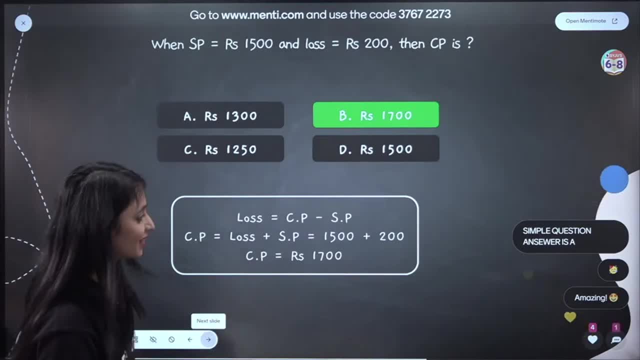 1700.. Ispe toh galat answer aana hi nahi chahiye tha. Yes, simple one right, Great, great, great. Now let's take a look at the leader board. Time chahiye likhne ke liye. next time onwards I will keep this in mind. 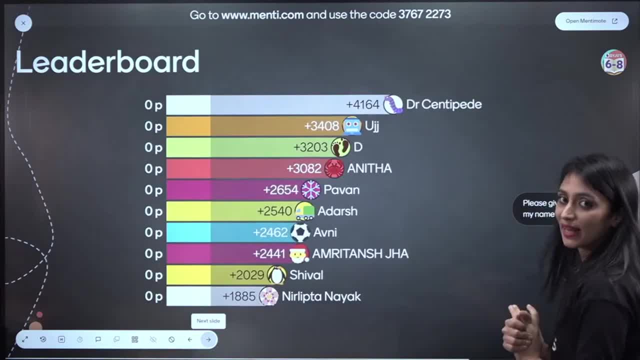 Oh, Dr Centipede. wow, wow, wow, wow. who is this? kya naam hai bhai, achcha naam likhne ka time nahi mila hoga, congratulations, Thank you, Thank you. 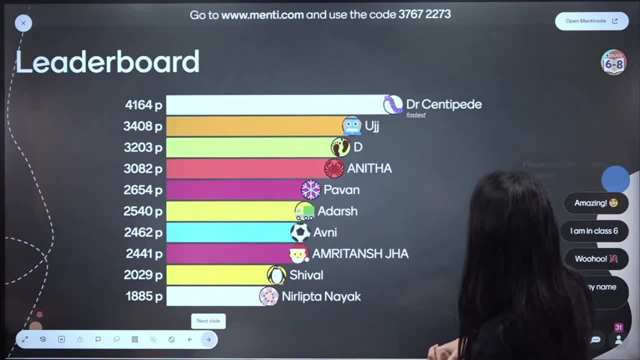 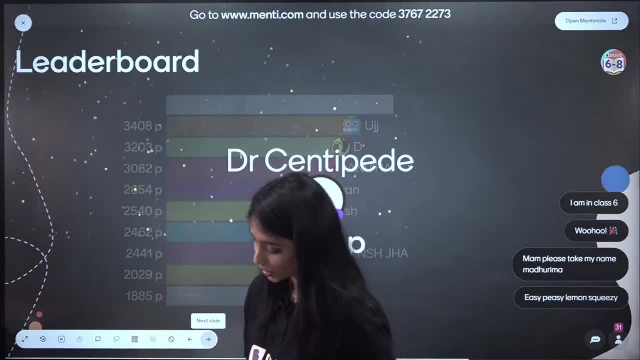 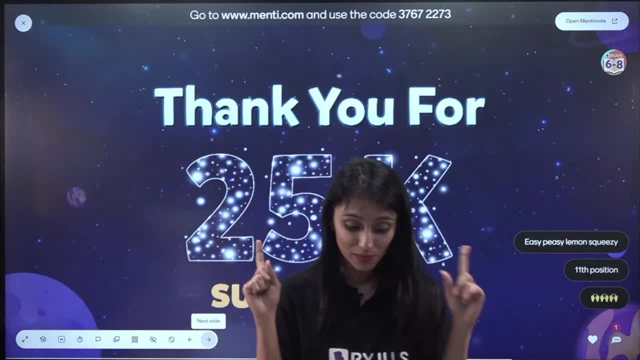 Thank you, 8th graders. thank you for understanding Chaliye. very nice. Jinka log am leader board pe nahi diya. koi baat nahi, And jindon ni abhi tak subscribe nahi kara hai. fatta fatte, please subscribe jitne bhi new. 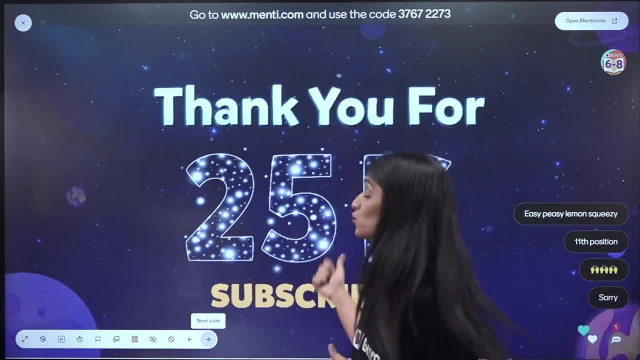 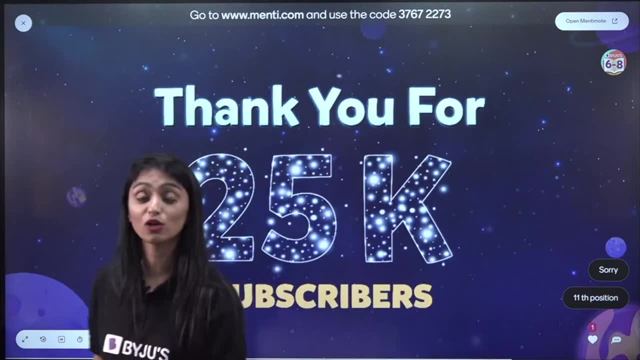 students hain because aap log bhool jaowa hoge. it hardly takes seconds Bhool jaenge, then you will be missing out on a lot of important, lot of useful sessions. trust me, Please subscribe the channel. hit the bell icon. also Telegram channel bhi join karo. and